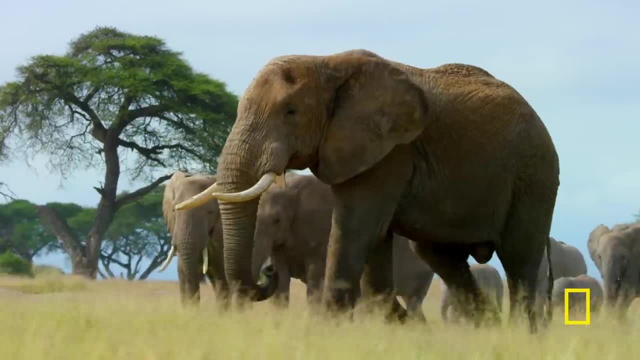 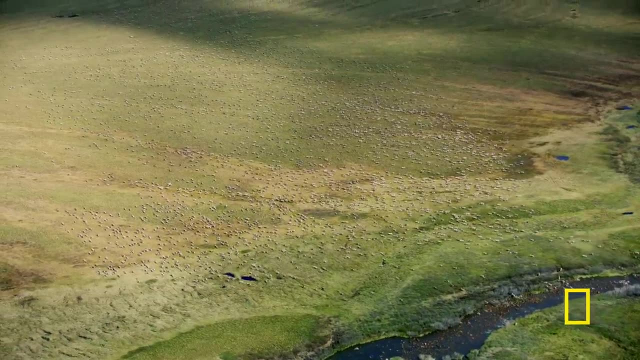 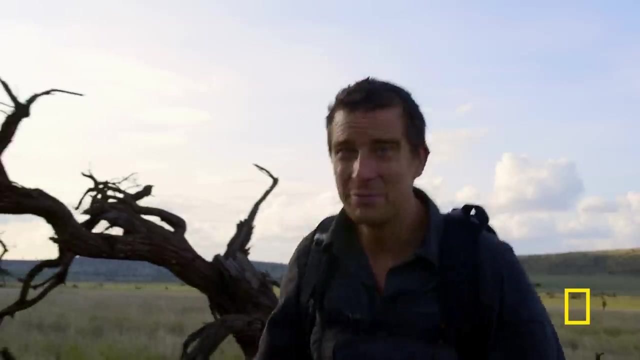 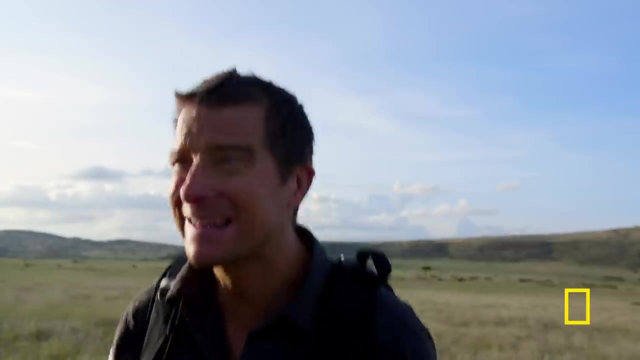 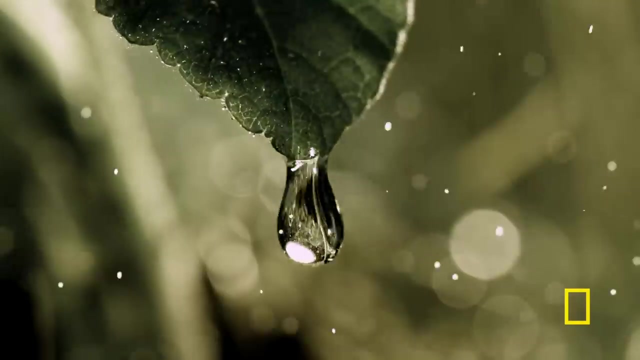 They support the largest animals And the biggest herds to walk the earth. Life on these great plains may look easy, But don't be fooled. When conditions turn, they can become some of the most volatile landscapes on our planet. A relentless cycle of flood. 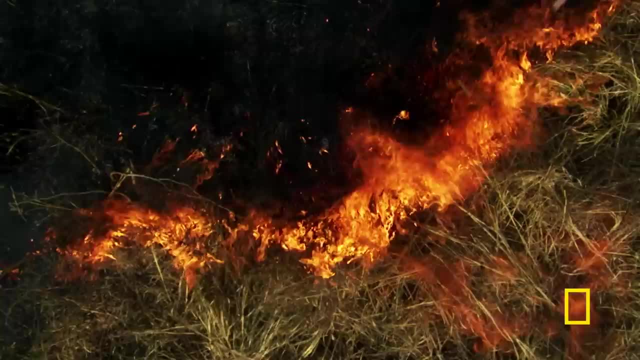 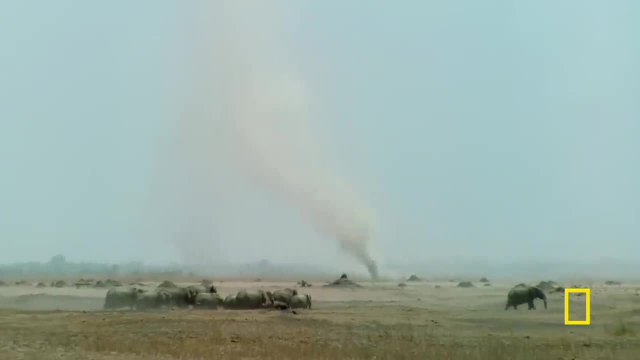 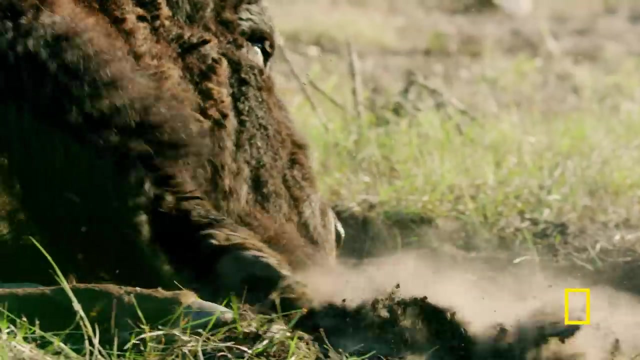 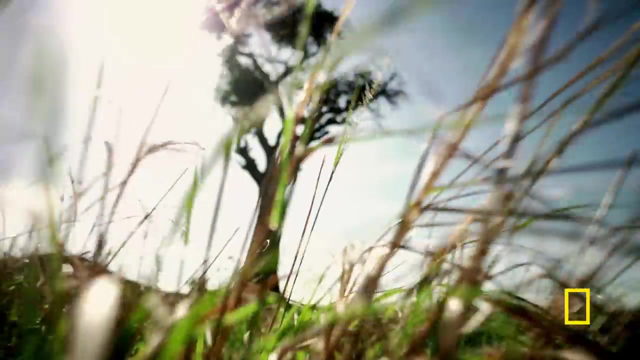 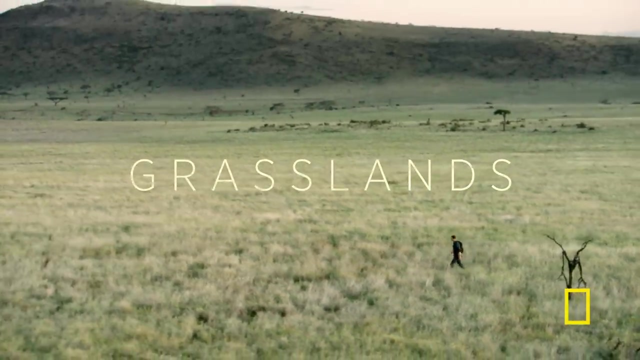 Famine, Freeze And fire, And as our climate becomes more unpredictable, It takes the animals of the grasslands to hell And back. The most ferocious of the carnivorous, Tarantulas, And my new favorite, The prairie. 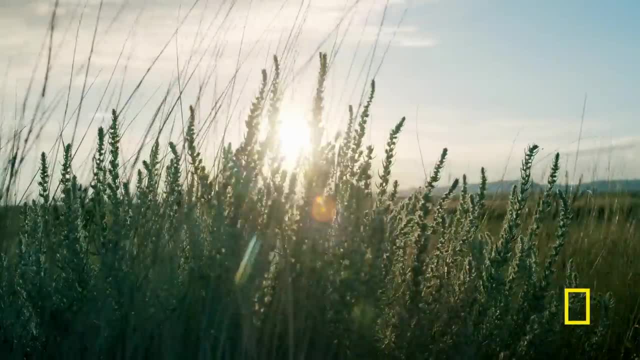 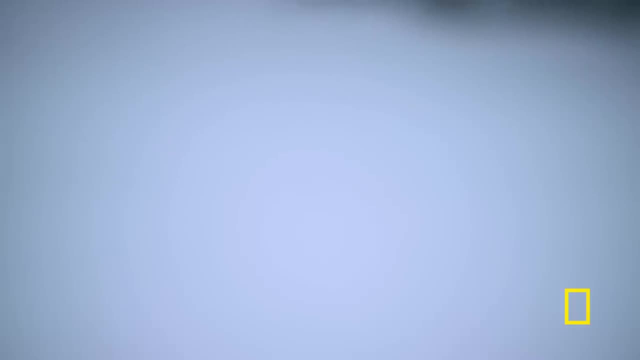 Yes, the prairie, And the vast swathes of spring And the vast swathes of fall And the vast swathes of winter And the vast swathes of winter And the vast swathes of autumn, Right below the Arctic. 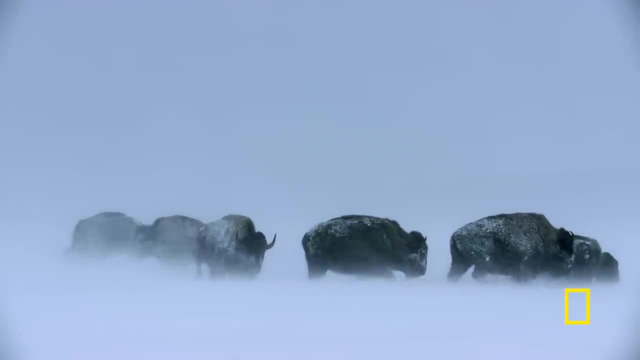 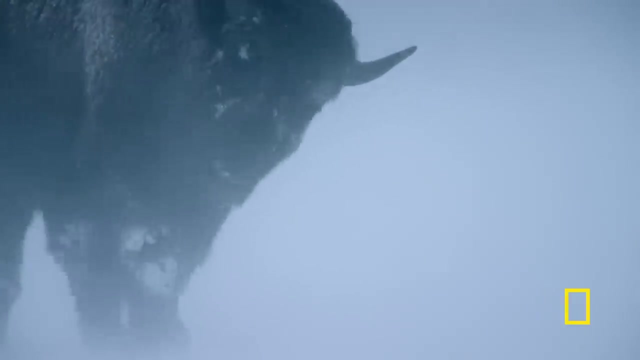 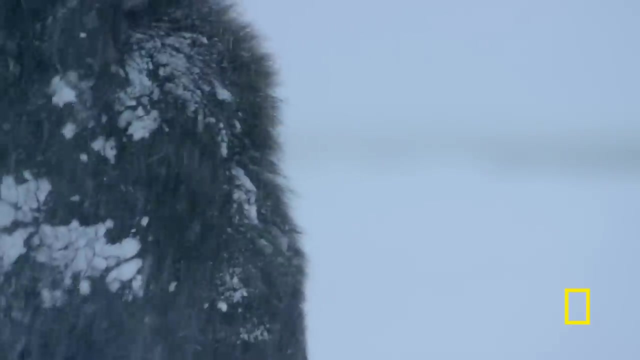 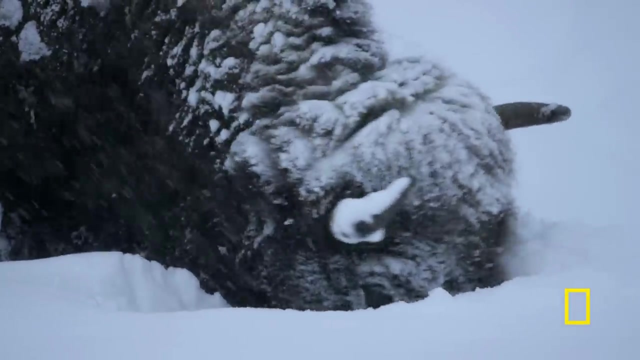 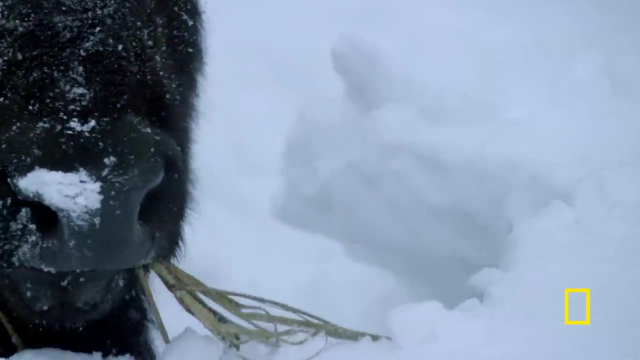 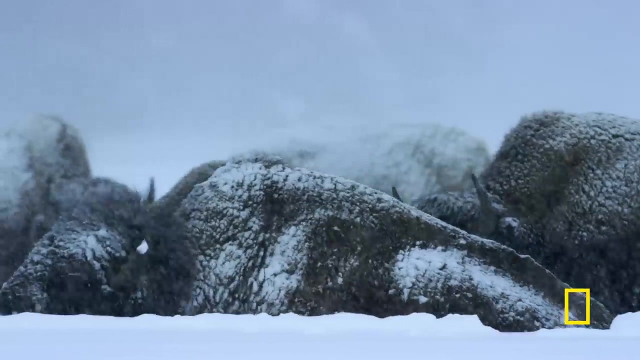 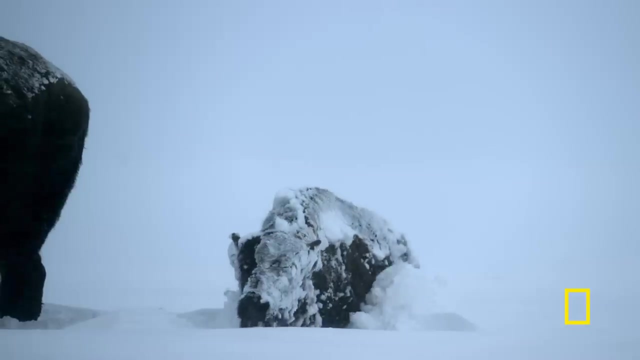 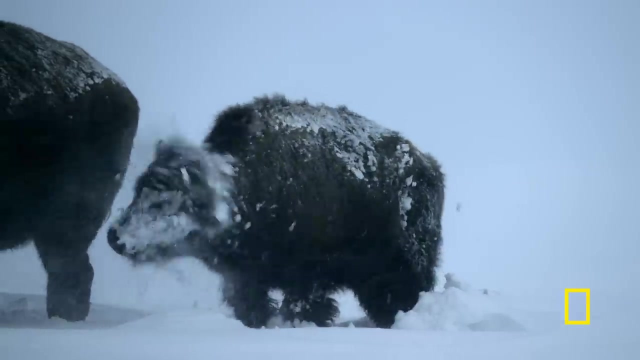 Deepest winter on North America's Great Plains, 40 below and record snowfall. Bison dig deeper for diminishing returns. Dead grass with the nutrition of cardboard. 23 pounds of the stuff every day still isn't enough. They're starving. The calves are the most vulnerable. 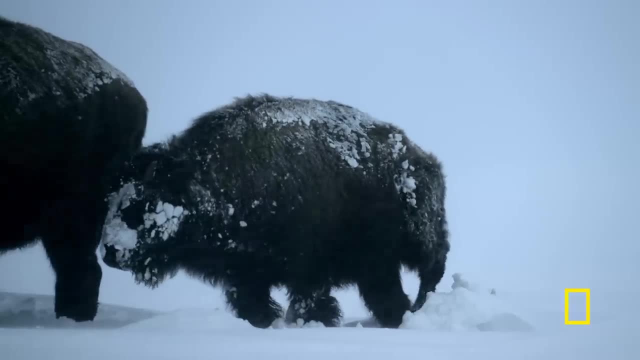 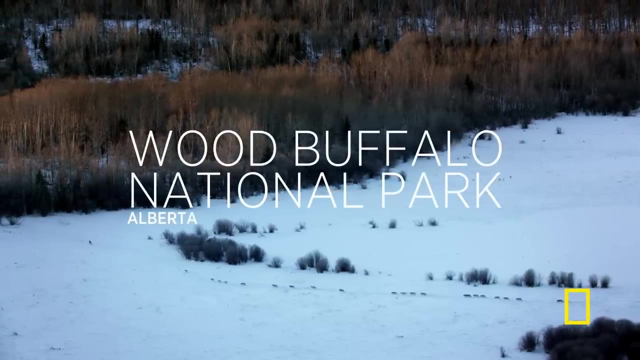 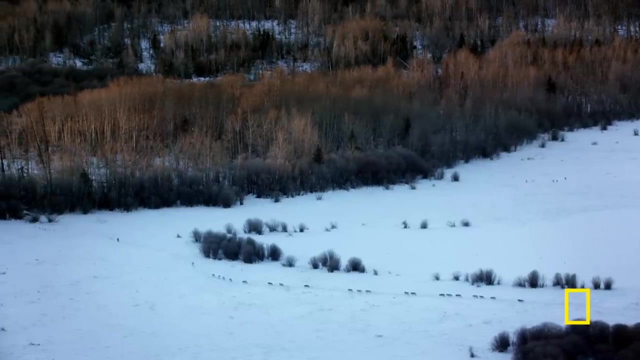 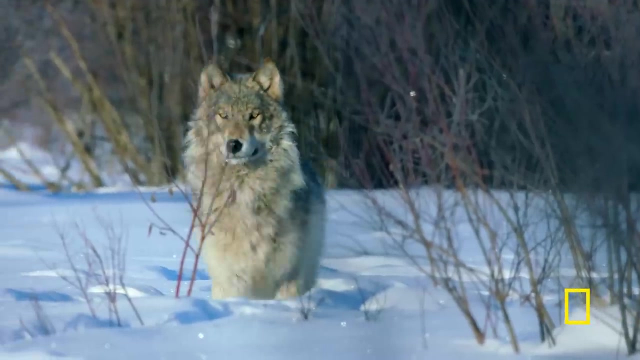 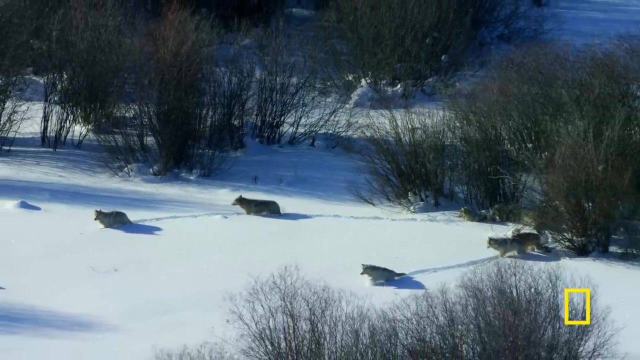 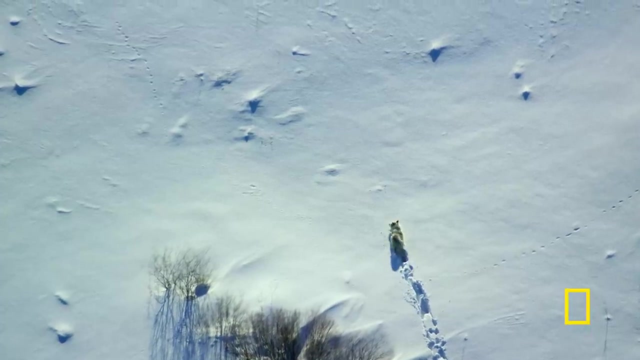 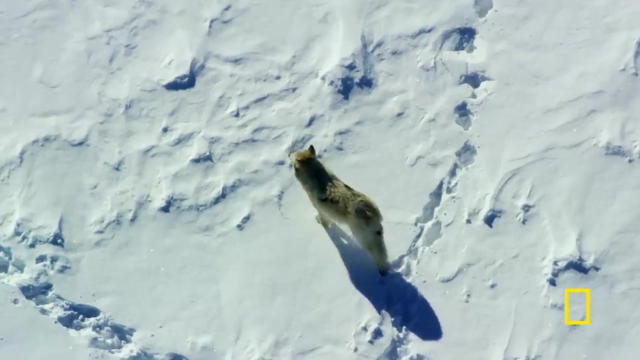 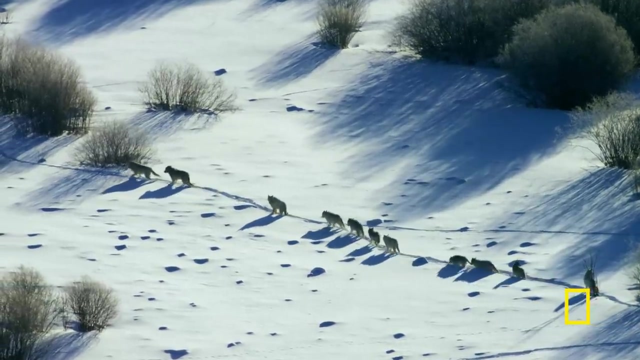 They're the most vulnerable, And they're the most vulnerable. And if the cold doesn't get them, another enemy might. Winter is a wolf's ally, A time to feed off the suffering of others. These are the biggest wolves in the world. 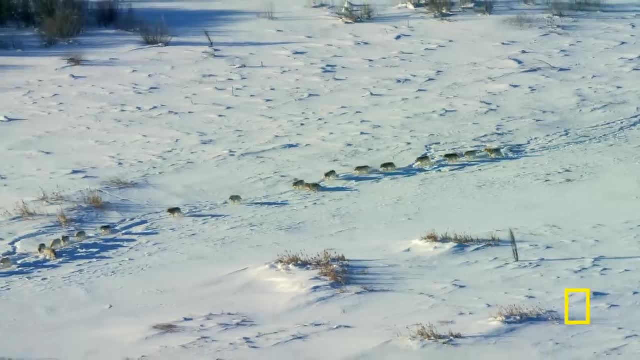 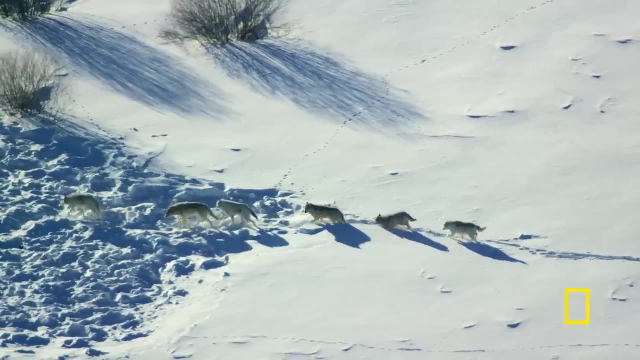 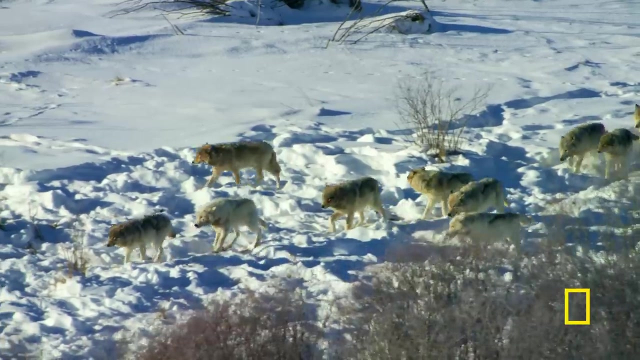 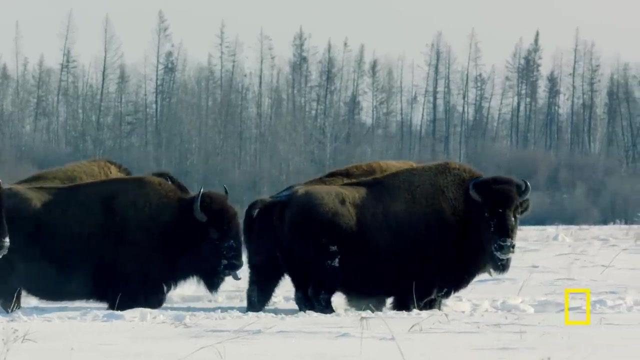 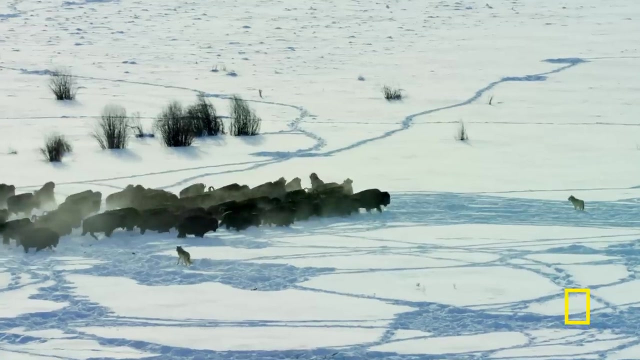 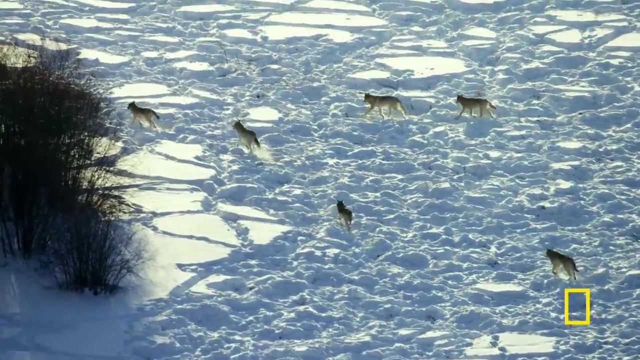 And at 25 strong, they're one of the largest packs. Size matters when you hunt giants Ten times heavier and well-armed. the bison are stronger. As long as they stand their ground, They're strong, But wolves create panic. 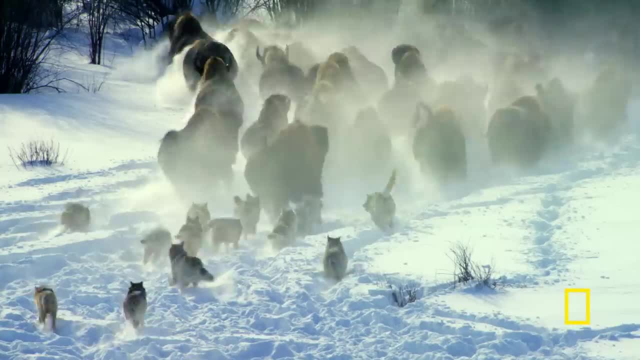 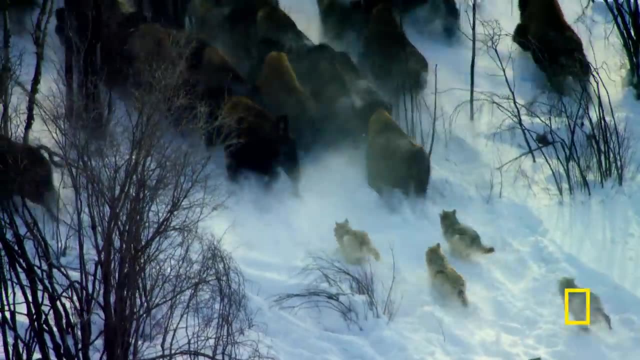 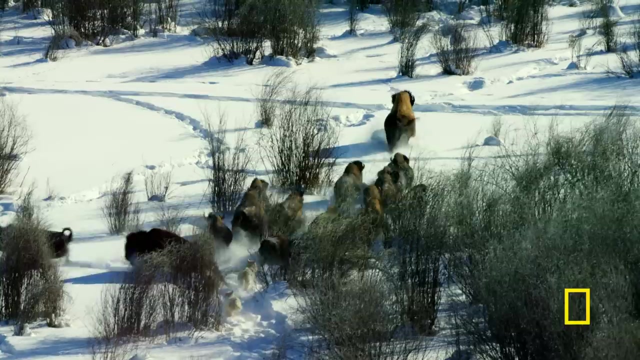 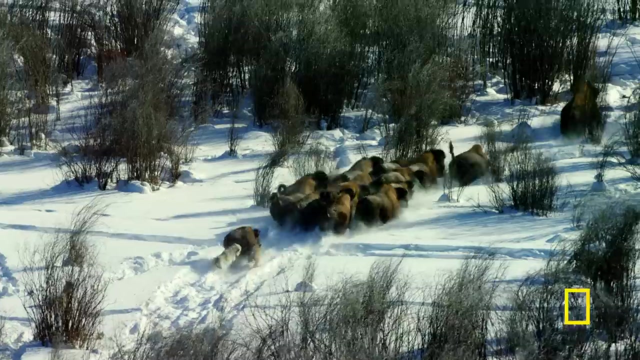 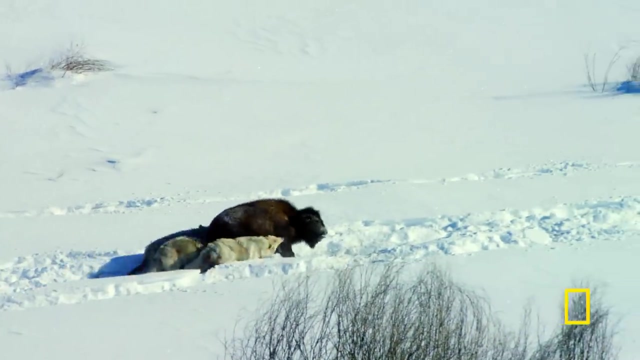 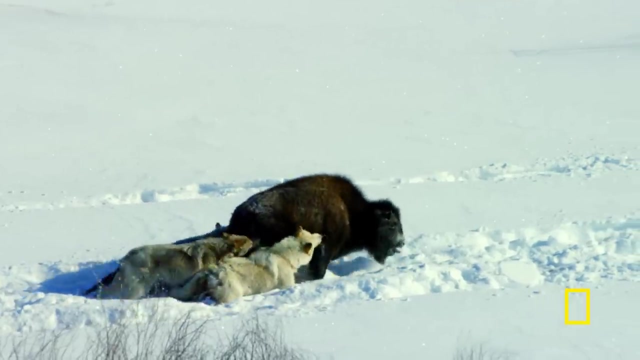 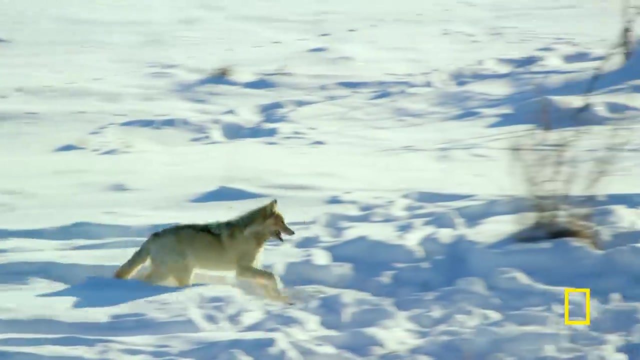 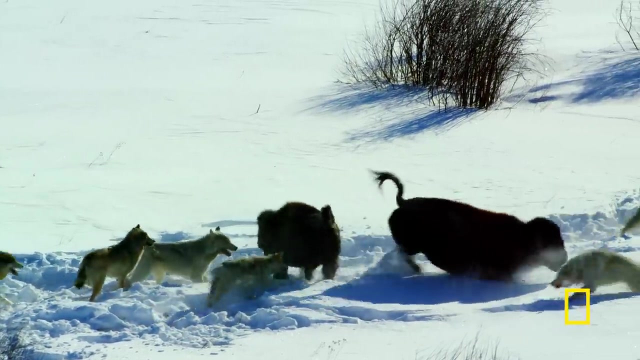 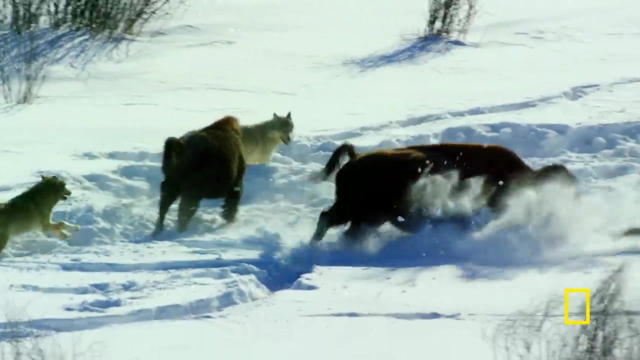 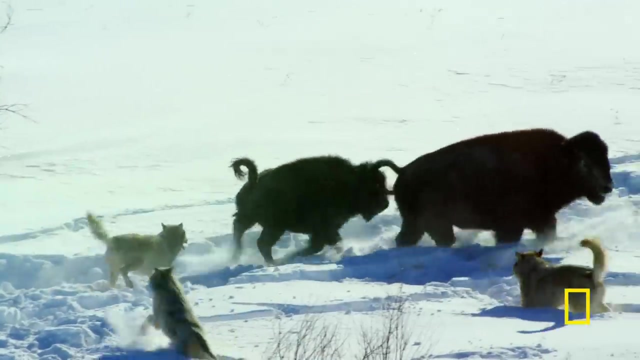 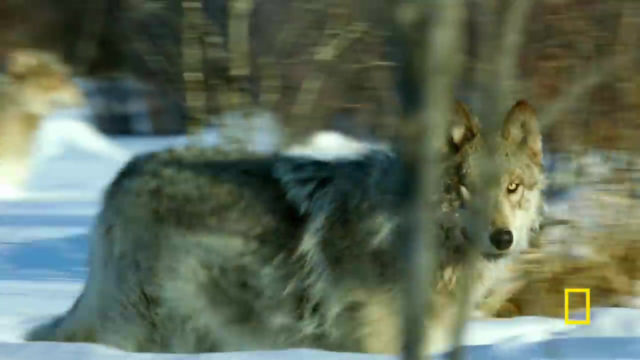 Running for the woods is a mistake. Trees break their formation and expose the weak Alone. a youngster is an easy target, But a mother will risk her own life to save her calf. They must make it back to the safety of the herd. 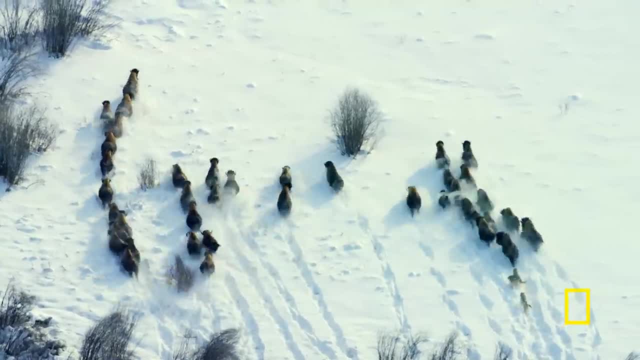 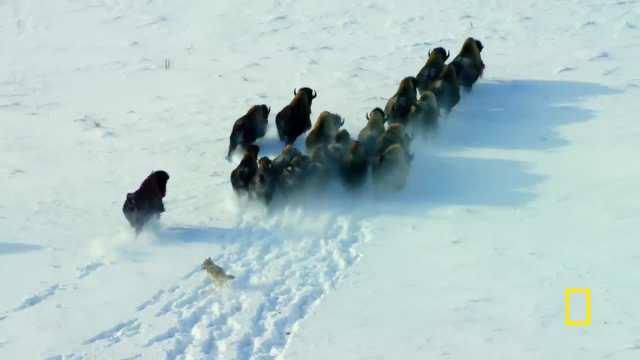 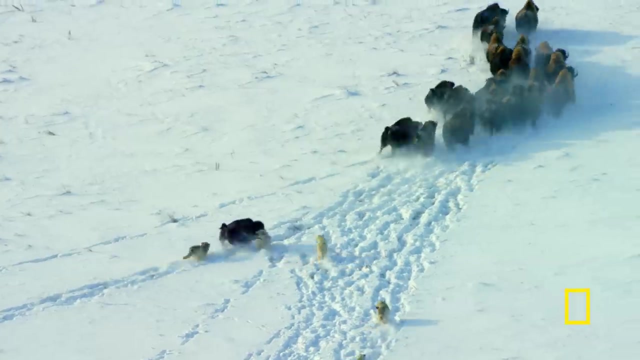 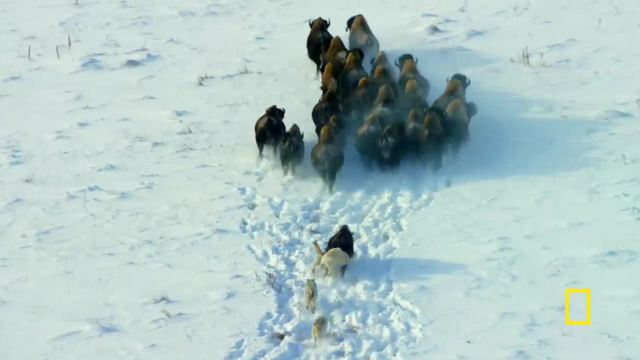 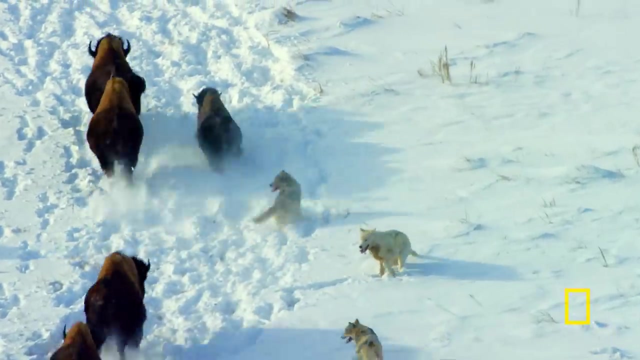 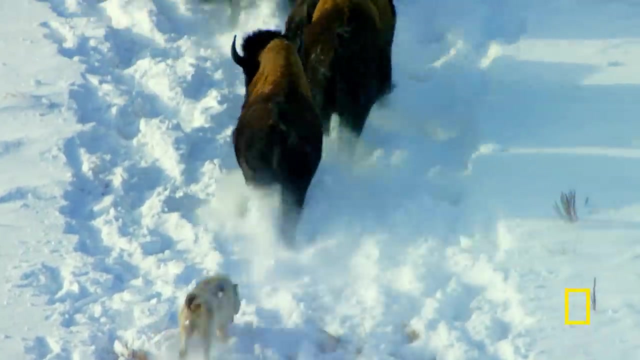 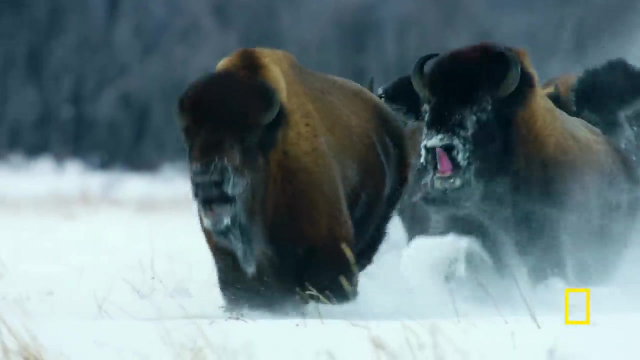 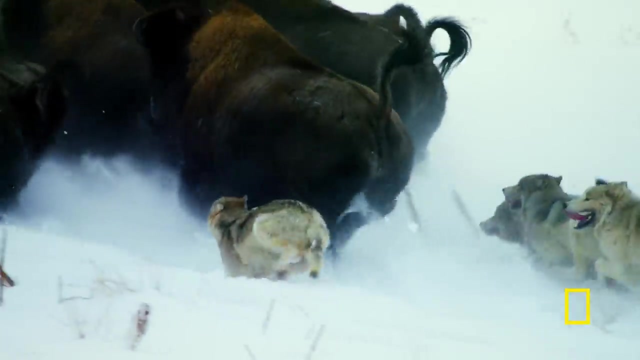 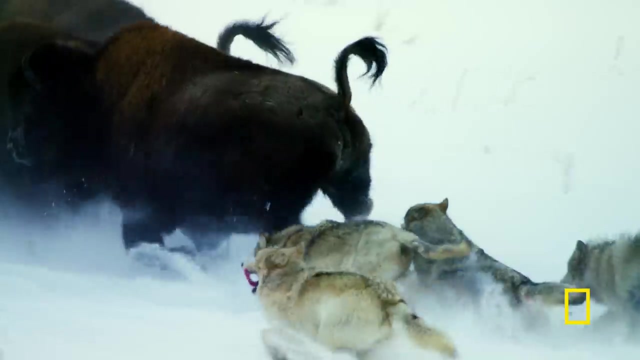 But deep snow saps the bison's energy. Again the calf is isolated, Again it's rescued. Now there's hope As long as the calf can stay hidden within the ranks. But there's a chance that one day aięcy will take it. 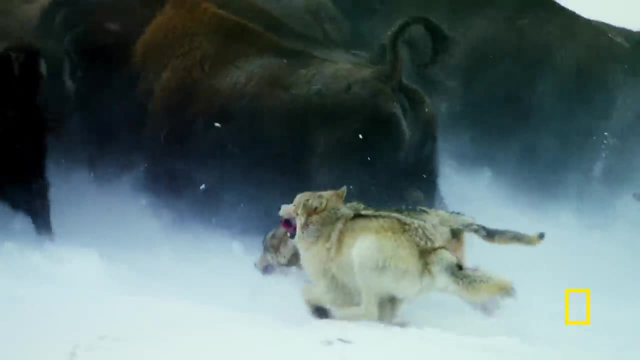 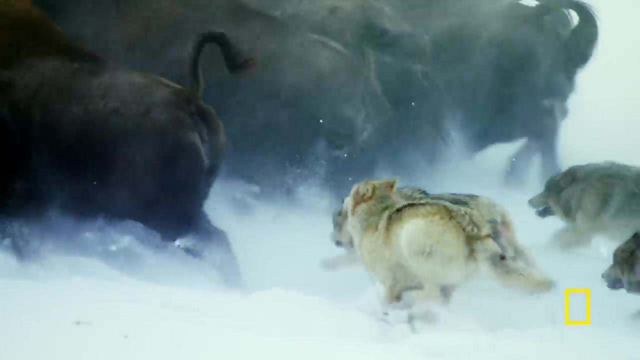 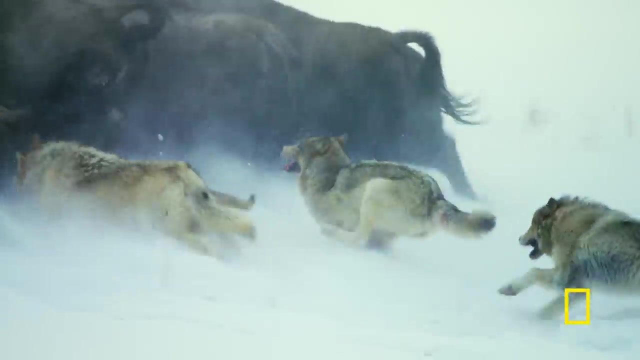 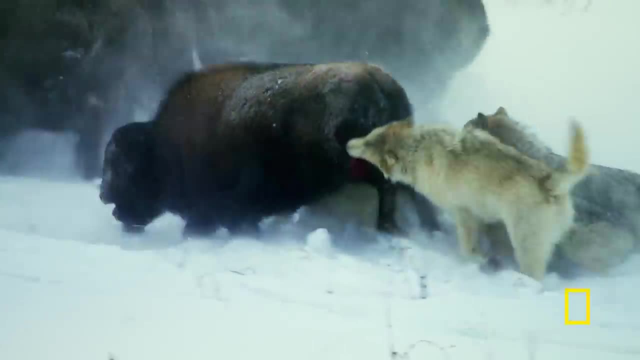 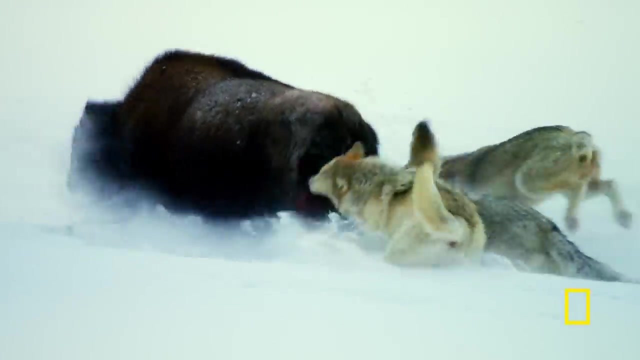 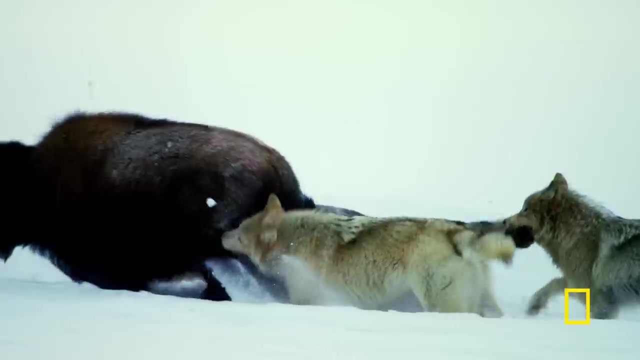 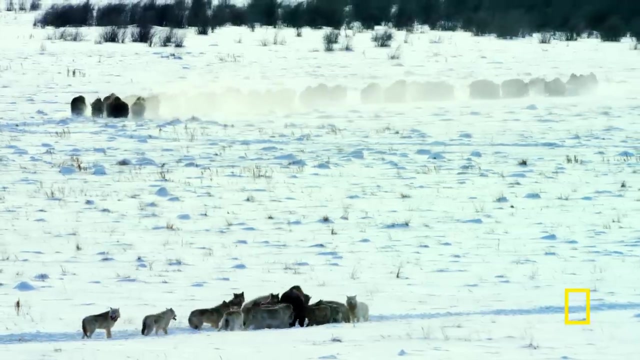 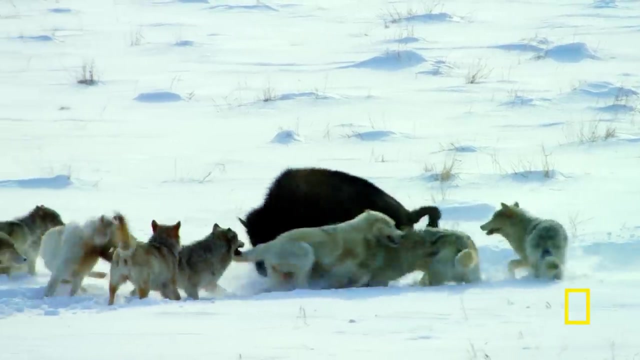 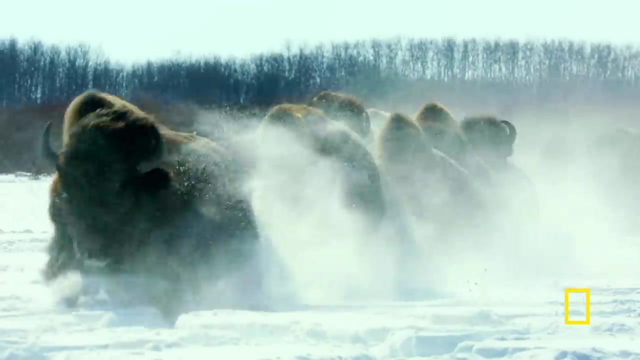 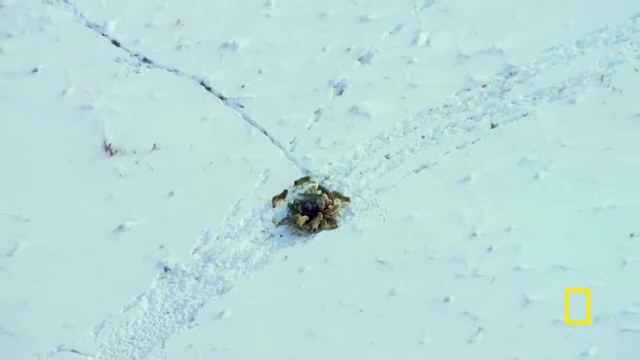 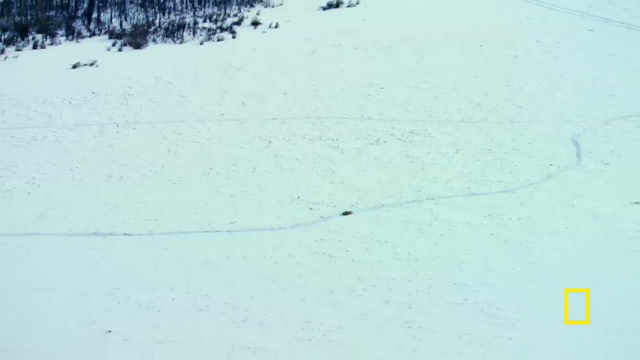 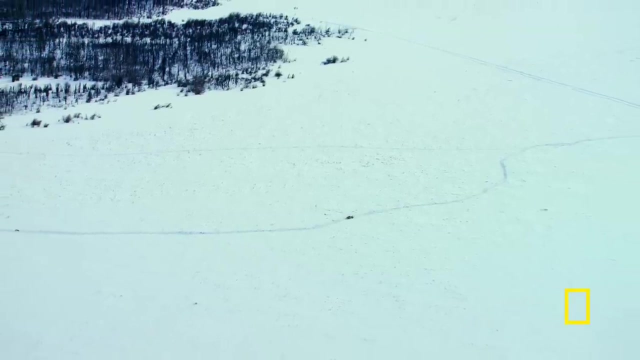 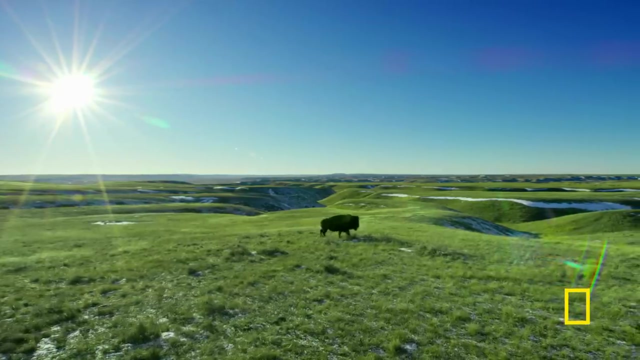 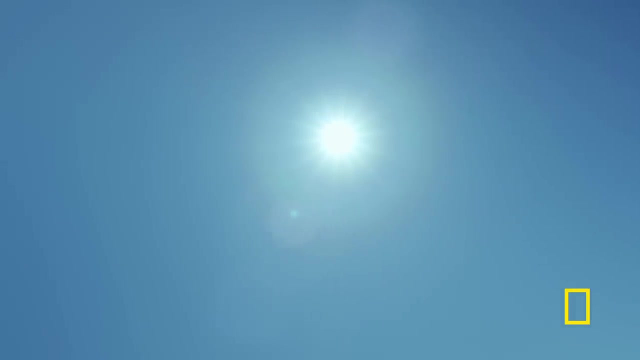 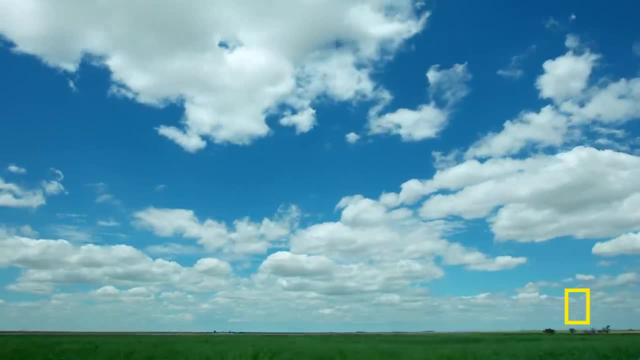 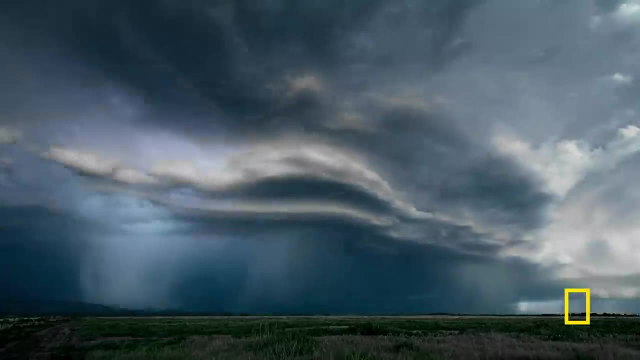 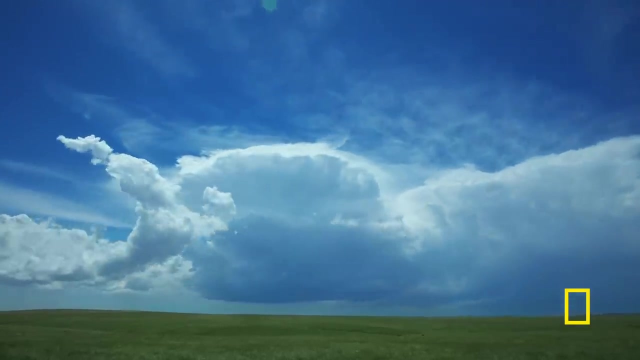 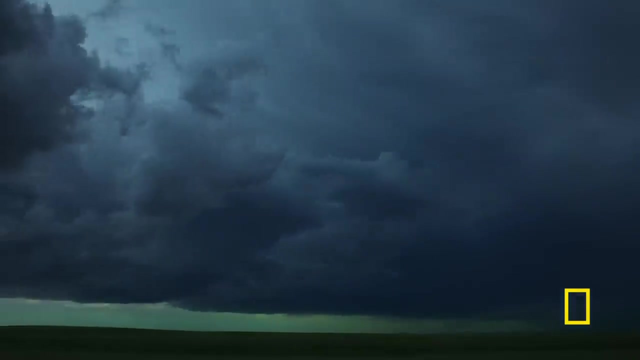 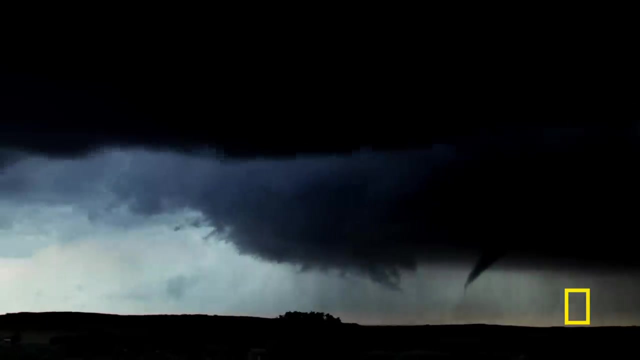 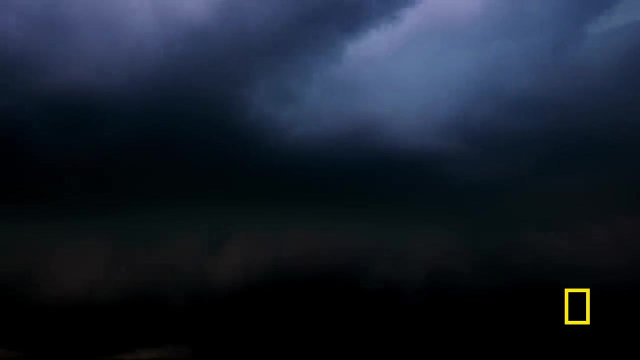 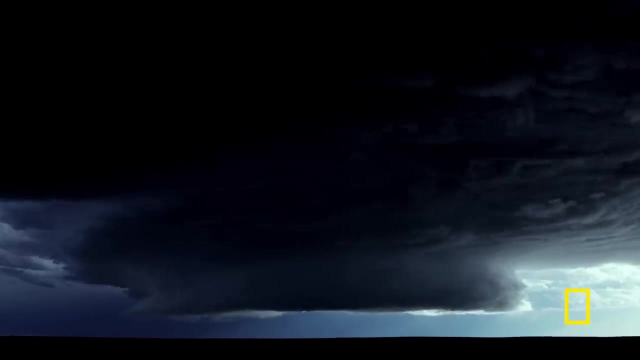 And a new danger is brewing: Spring and the start of storm season. North America's Great Plains are a hotspot for some of the most intense thunderstorms on Earth. Some mutate into supercells, Monsters with the equivalent energy of 100 nuclear bombs. 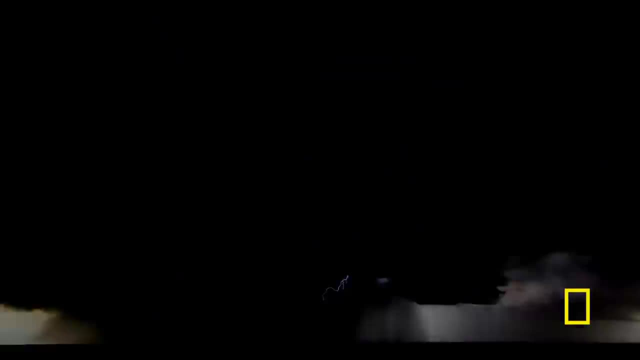 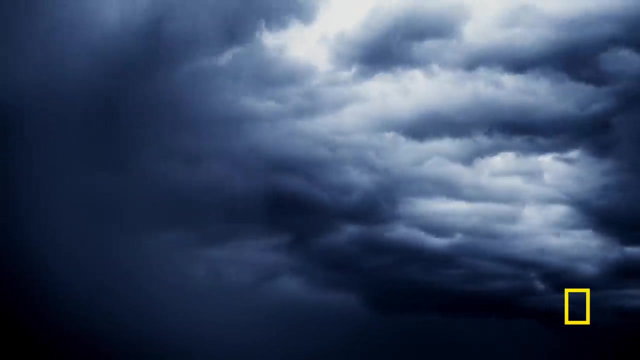 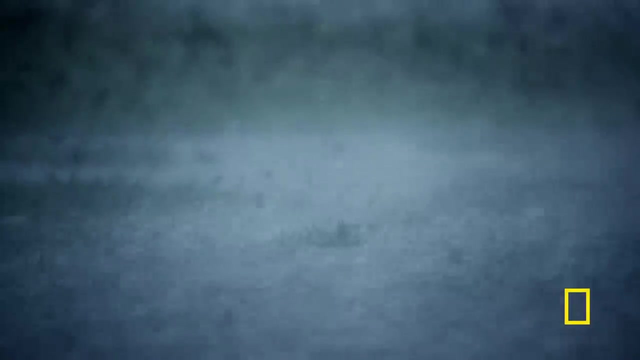 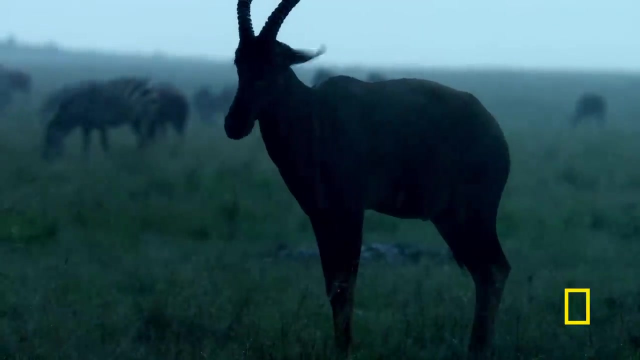 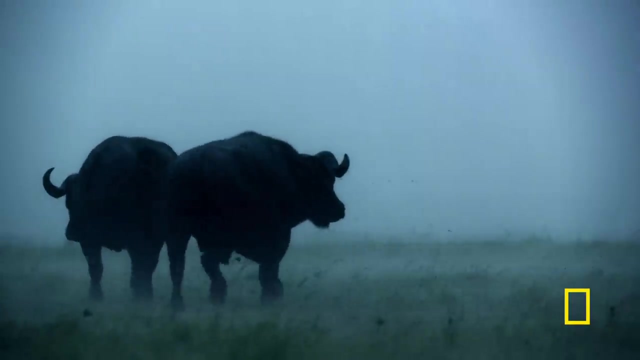 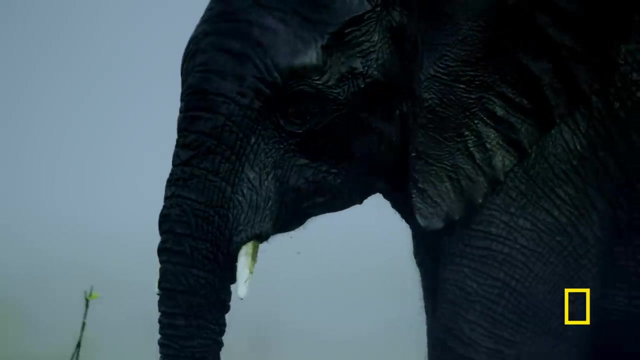 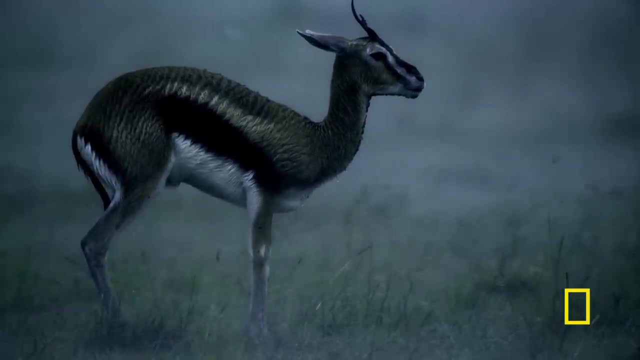 Storms are becoming more frequent. here And in grasslands across the globe, weather patterns are increasingly erratic. Here, the rains are a month early and hitting hard. Over a year's worth of rain in just a couple of months. 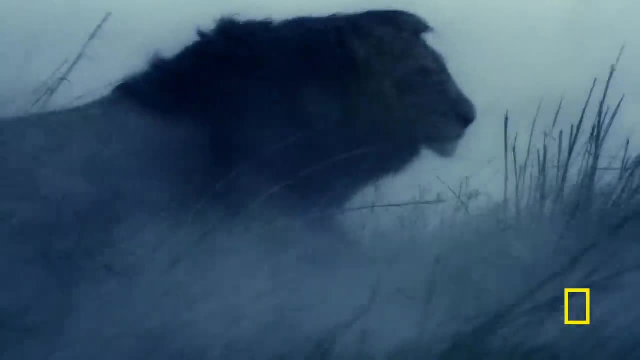 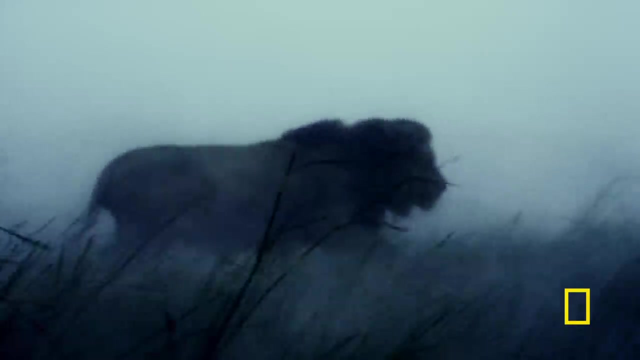 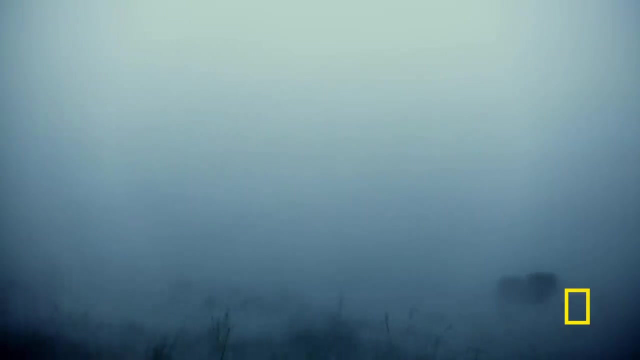 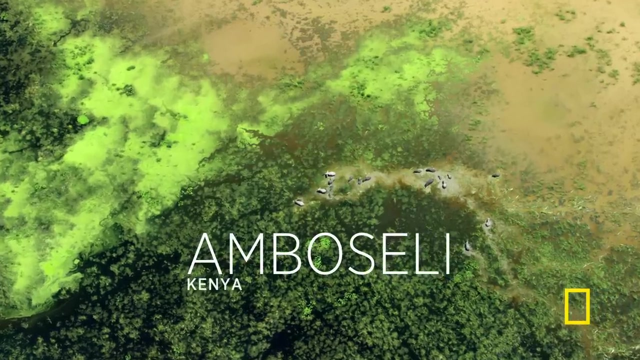 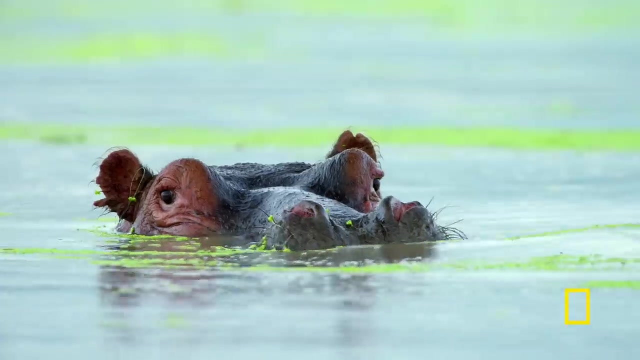 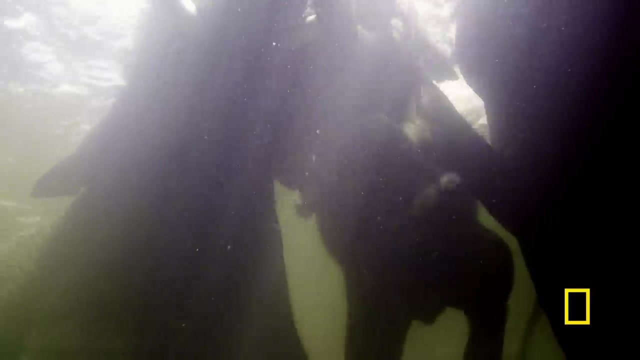 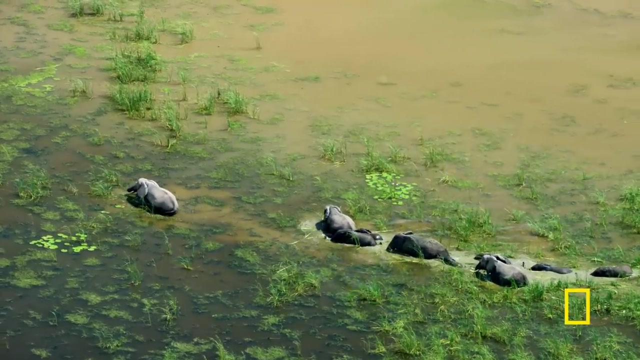 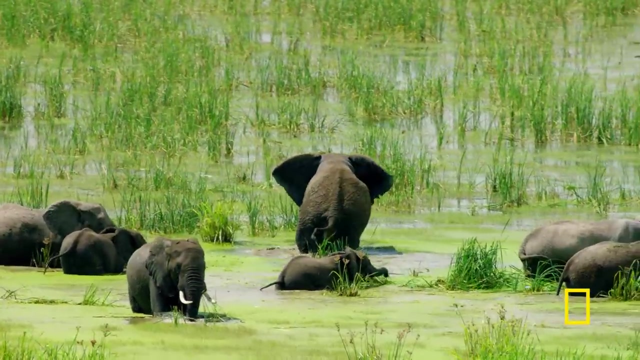 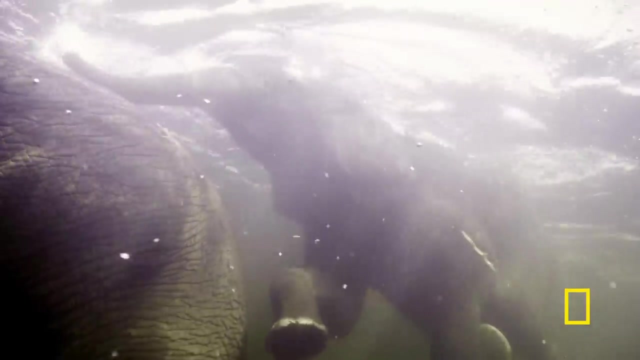 Not a problem for the adults and plenty of fresh grass, but a bit deep for a calf. 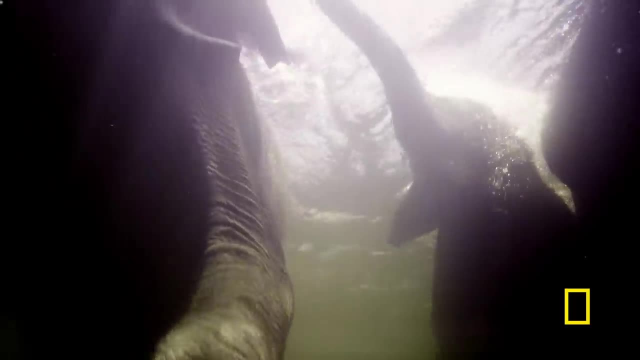 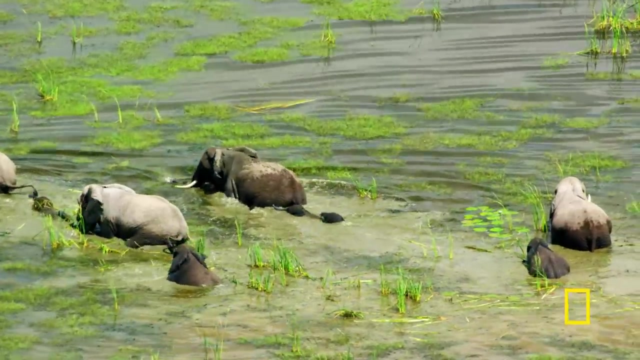 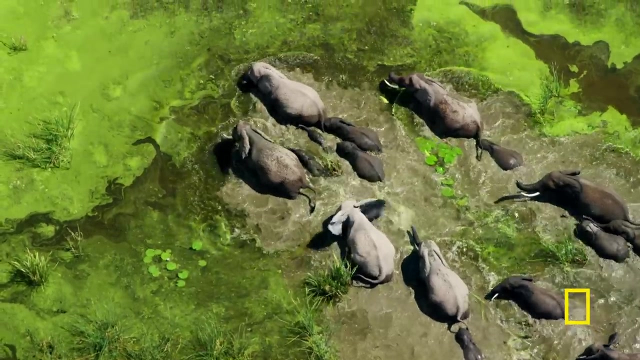 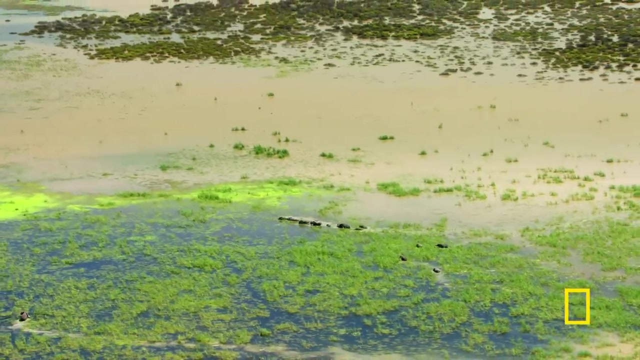 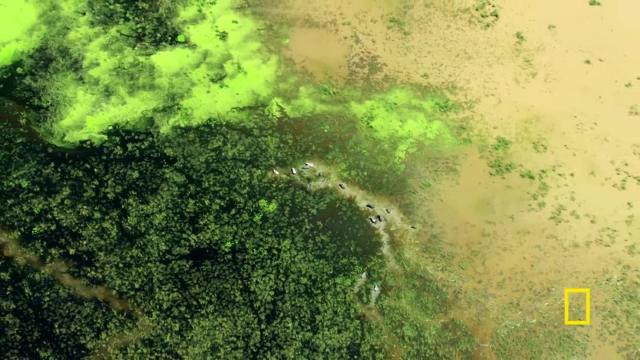 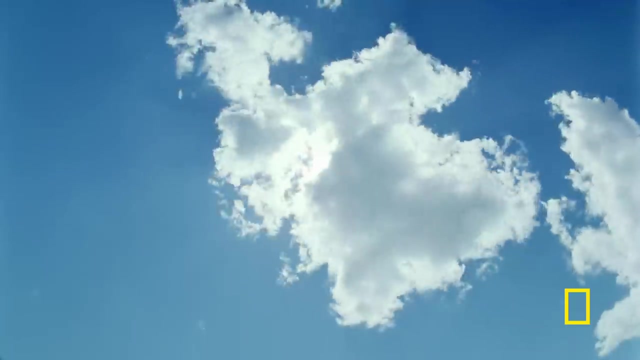 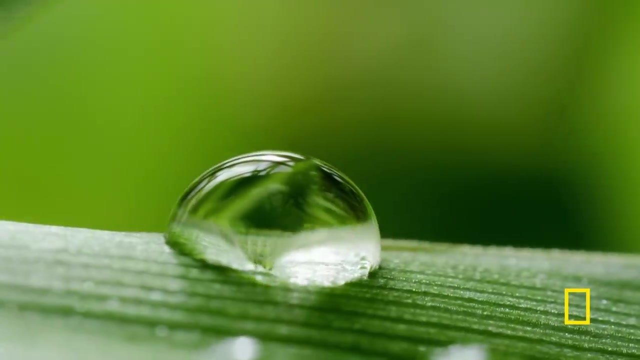 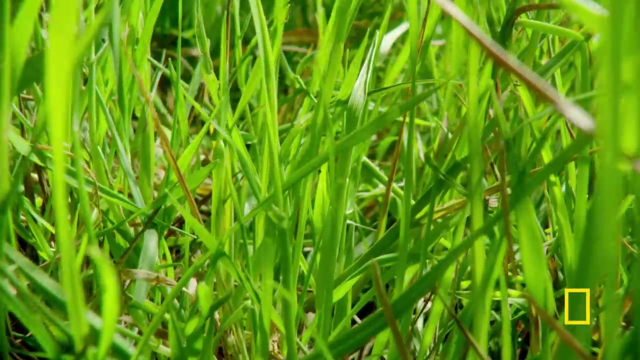 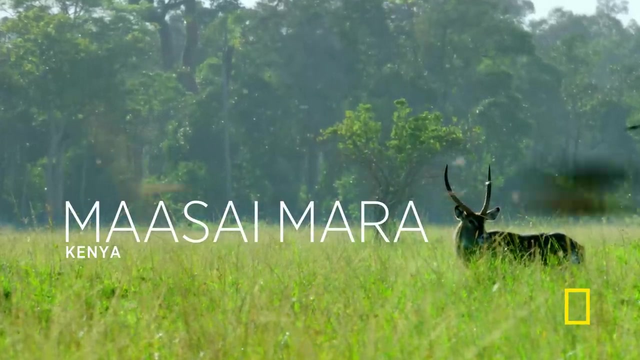 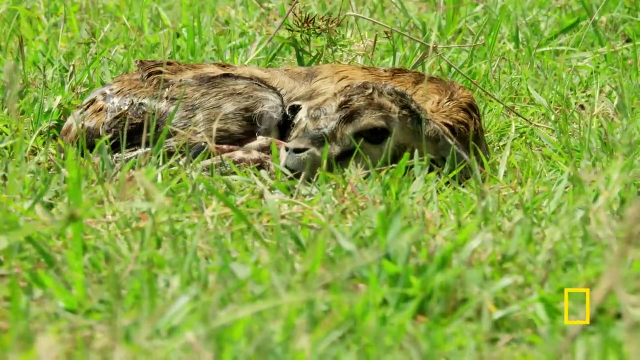 Luckily he has a snorkel. These floods may complicate things a little in the short term, But they'll revitalise life on the savannah. As the flood waters subside, they reveal the flush of new growth And fuel a baby boom. 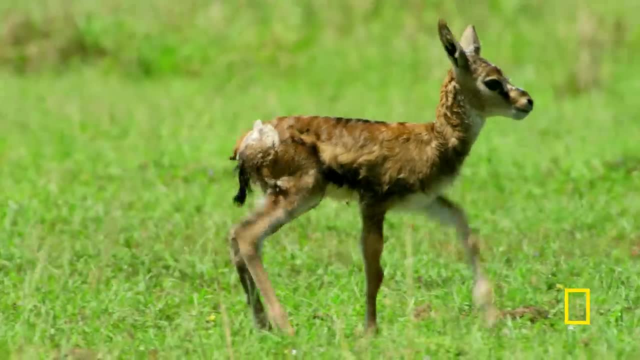 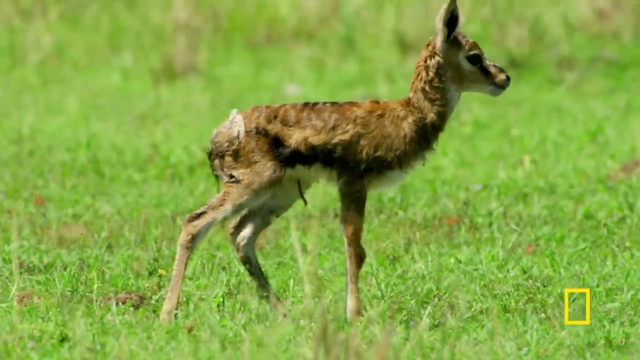 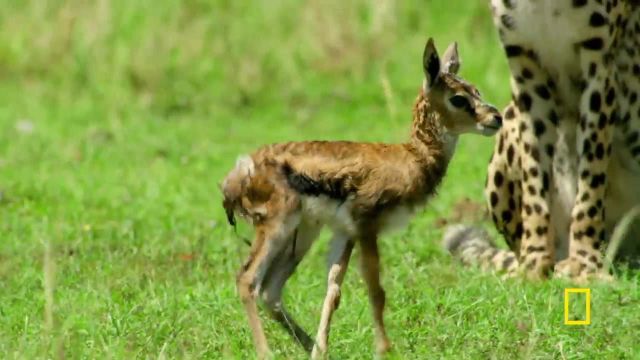 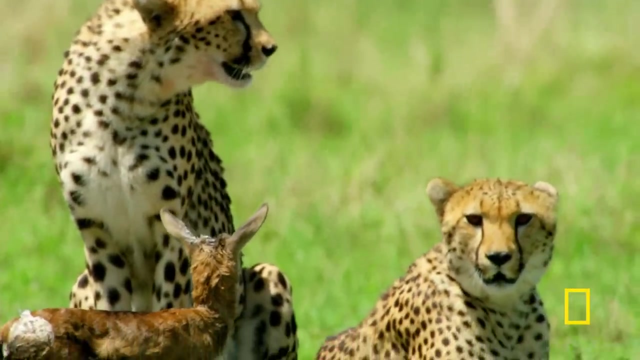 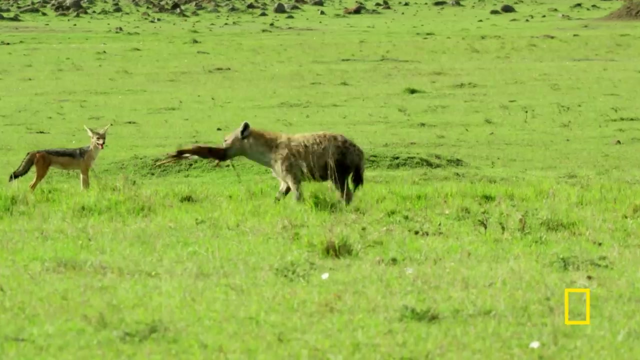 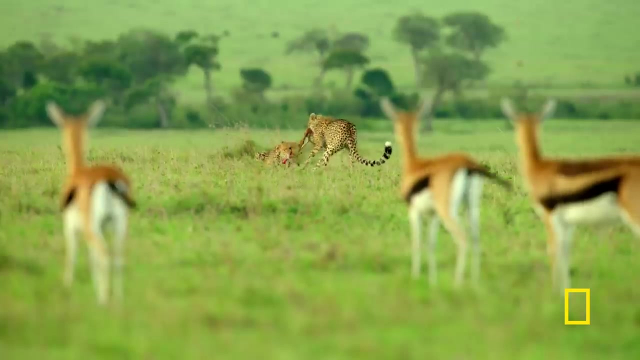 But this can be a dangerous place to take your first steps. It's home to more large predators than anywhere else on Earth. 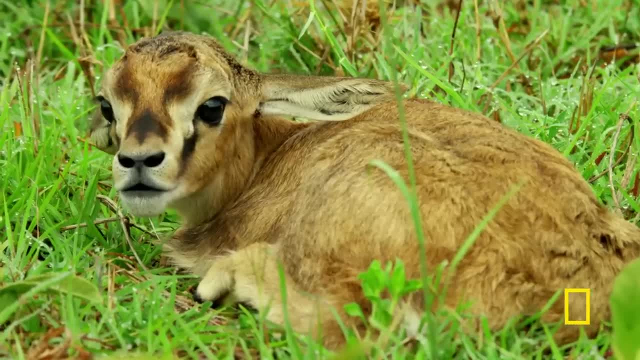 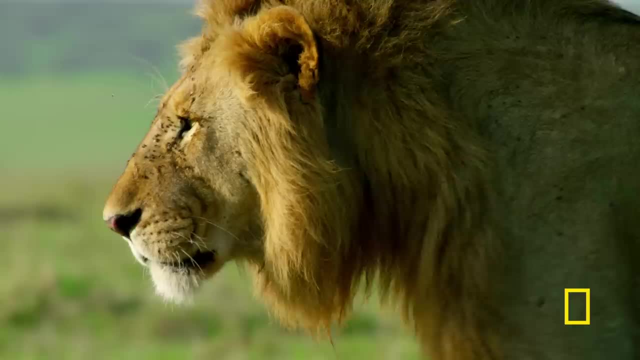 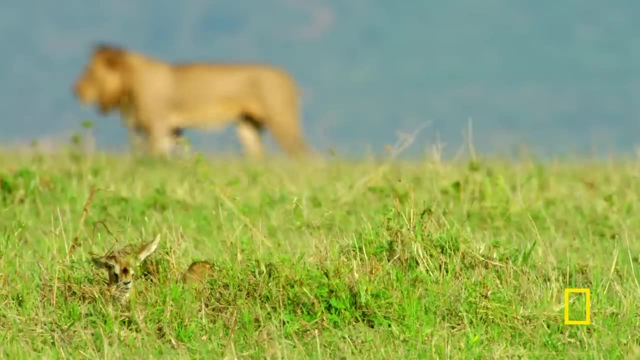 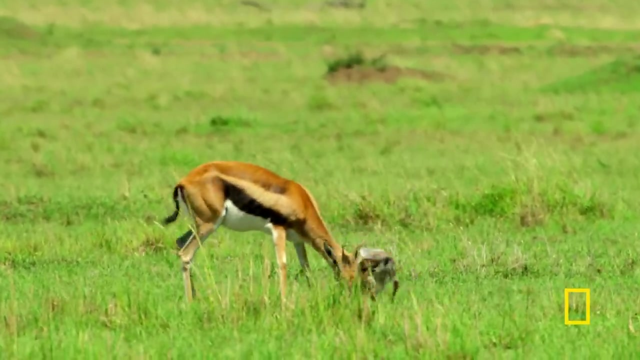 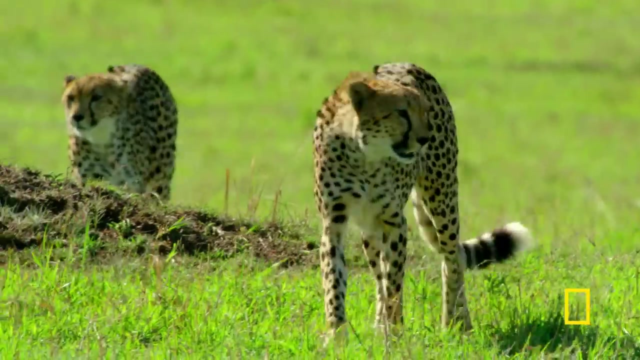 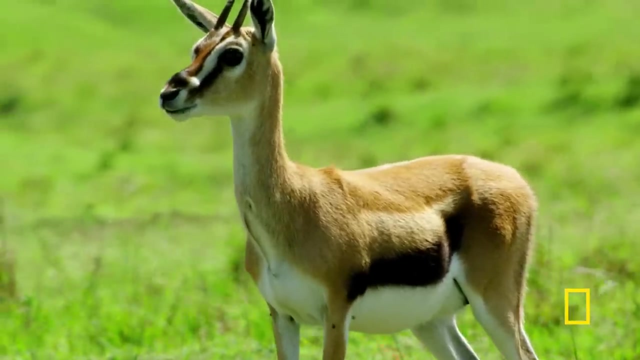 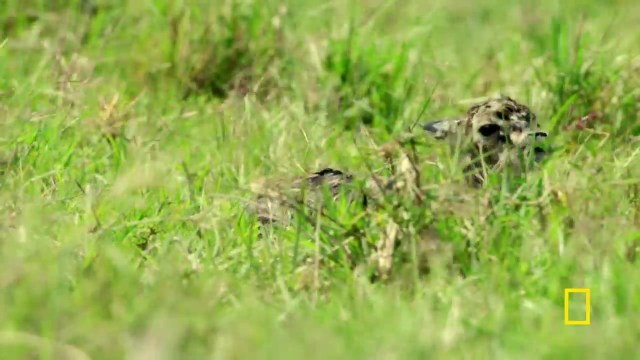 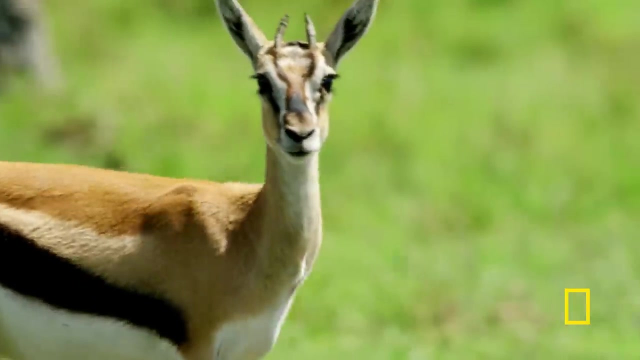 Their only hope is to hide. Mothers clean their newborns to remove any scent, But for this fawn there isn't time. If mum stands guard, she'll blow its cover. She has no option but to walk away. 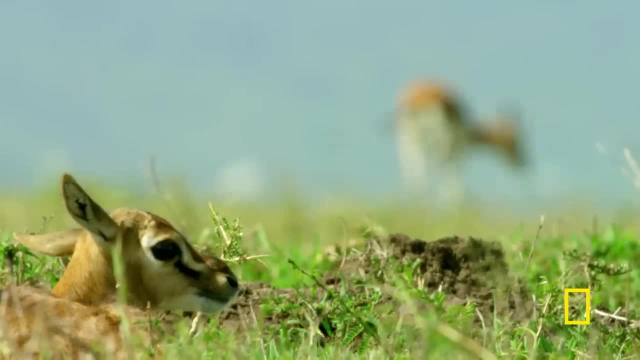 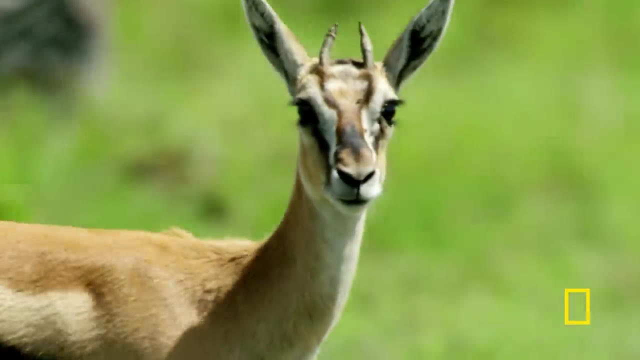 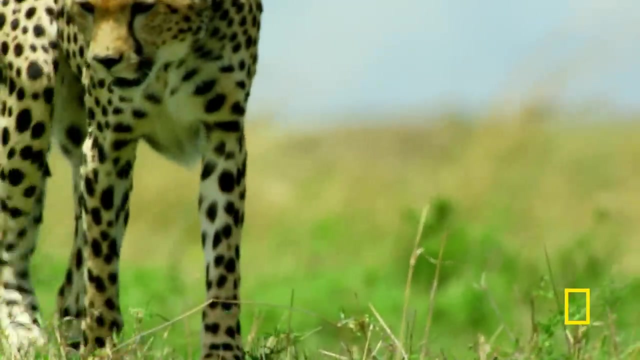 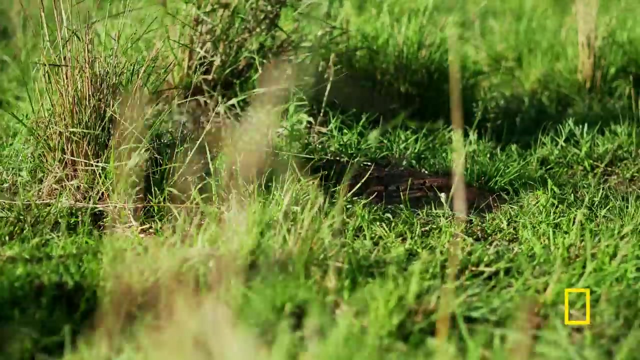 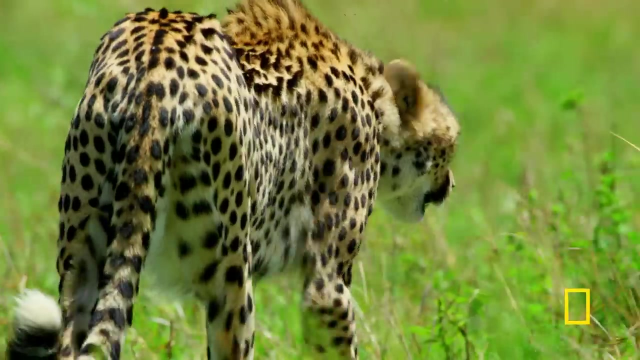 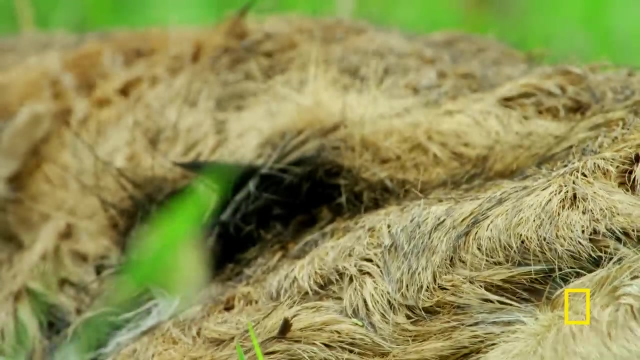 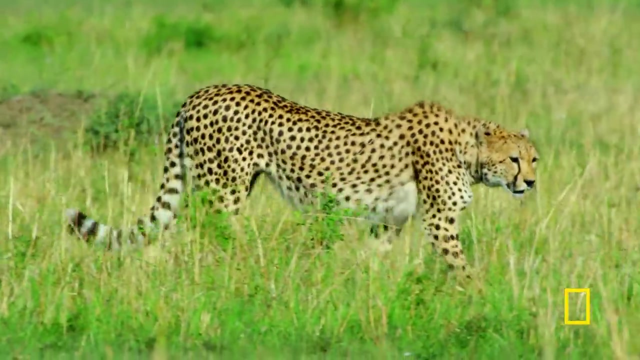 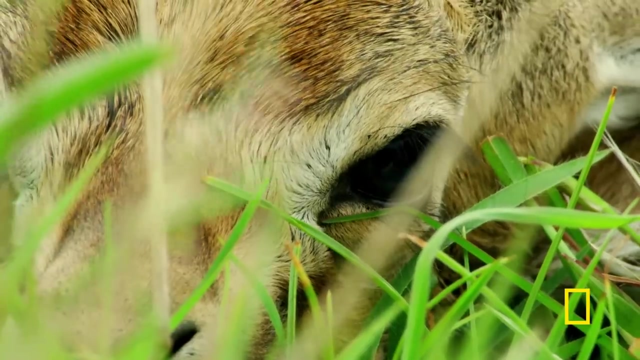 The cheetah's hunting instinct is triggered by movement. A motionless fawn looks remarkably like a mound of earth. All it can do is stay down, stay still, hope someone else is spotted first. 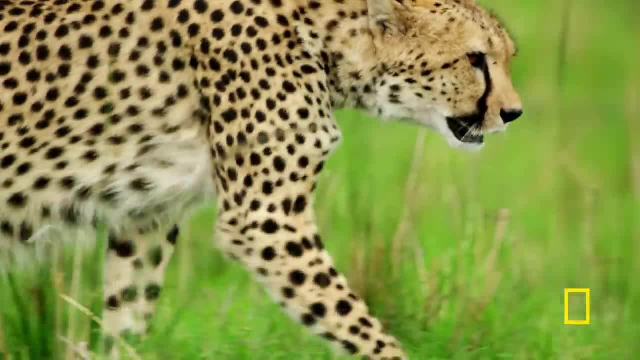 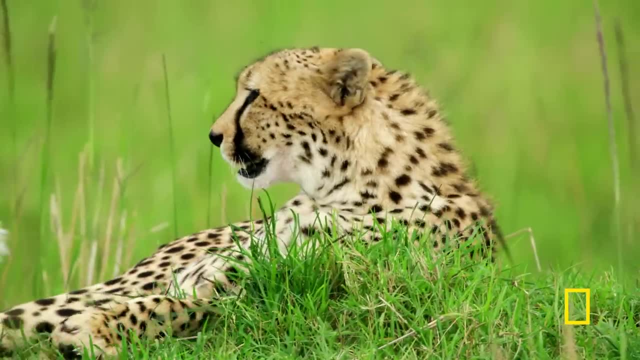 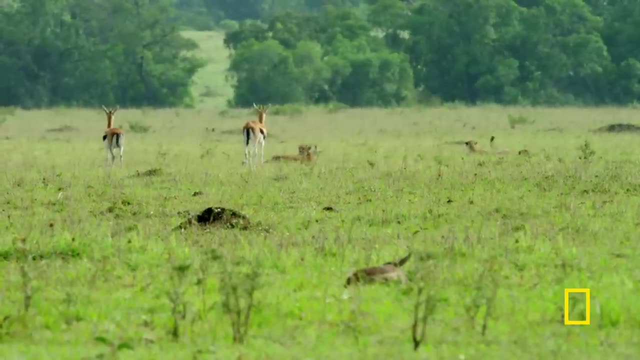 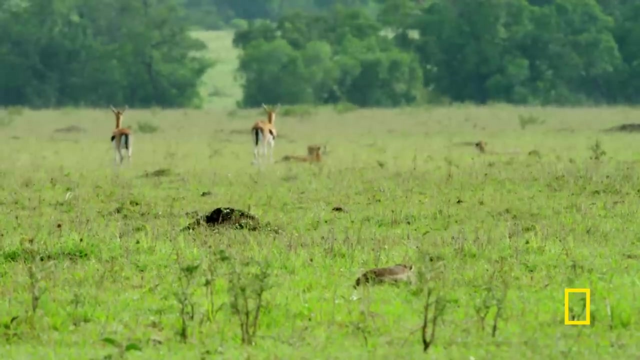 Cheetahs are patient, But the fawn will need to suckle soon. Worse still, the birth fluid is attracting flies. 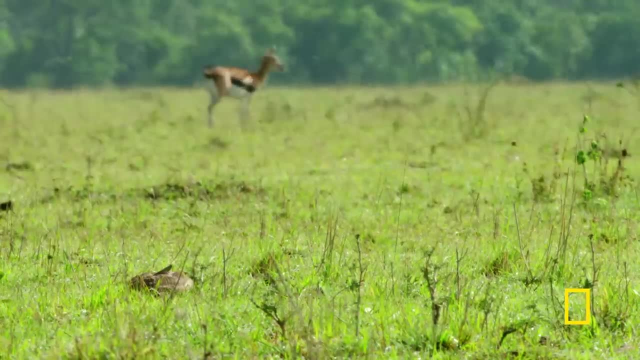 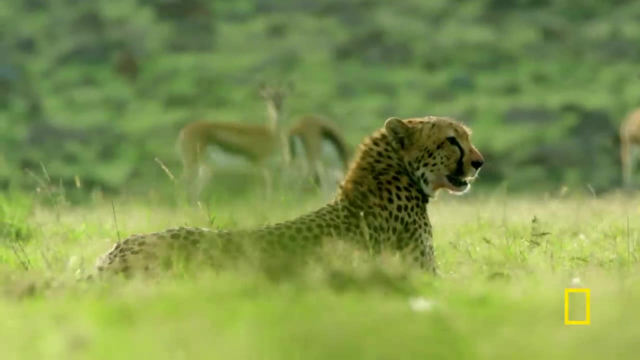 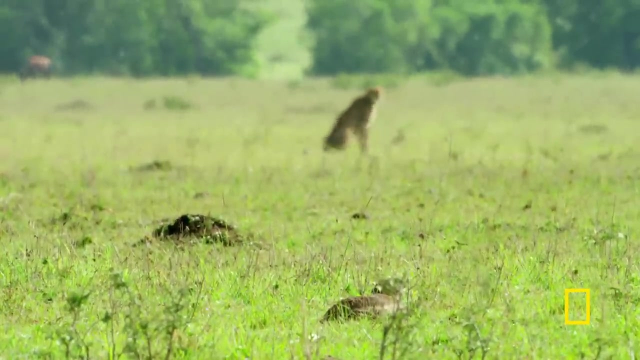 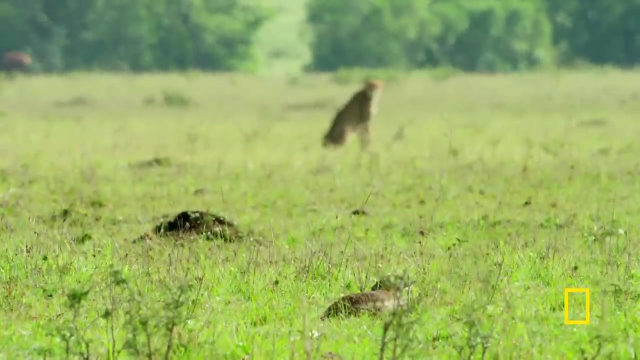 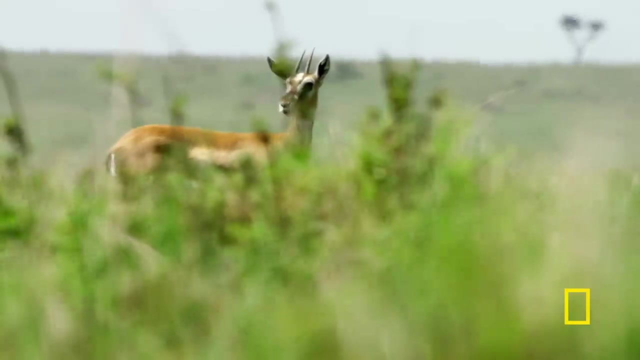 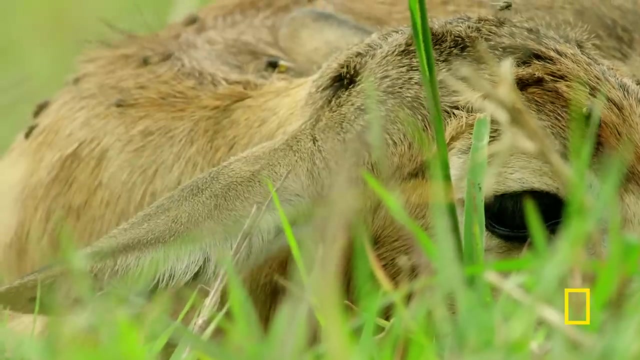 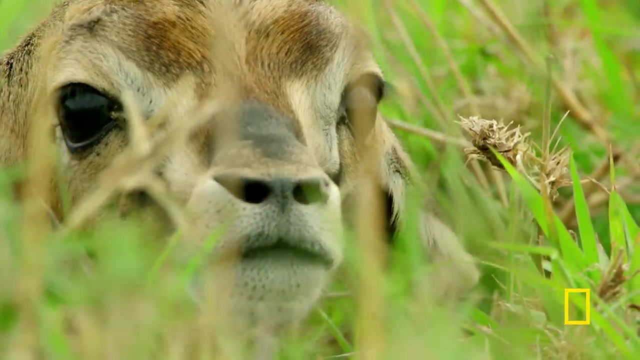 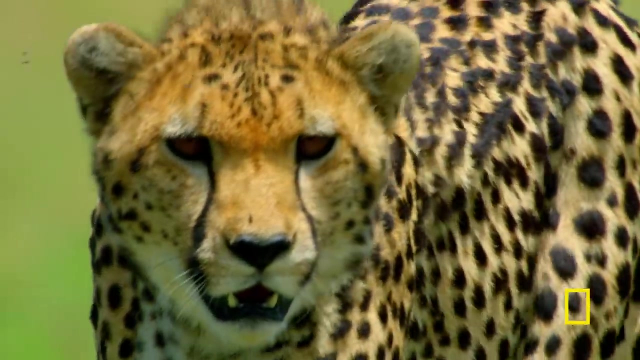 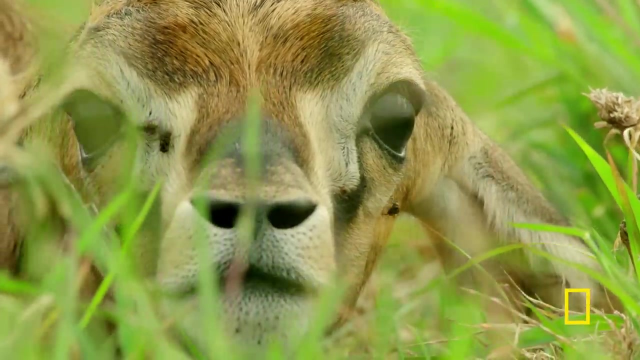 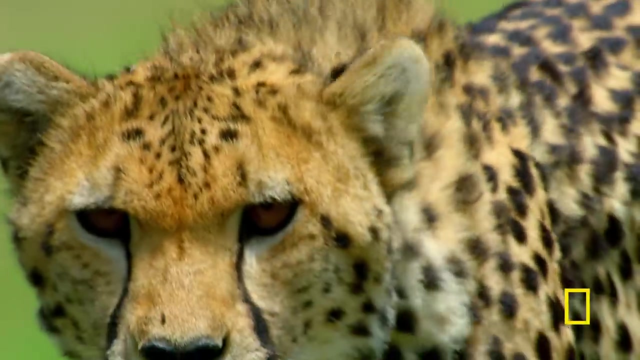 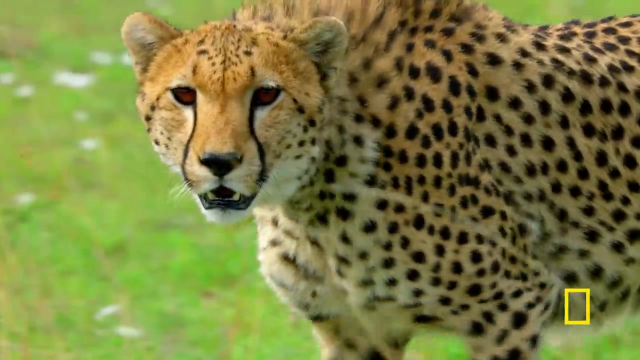 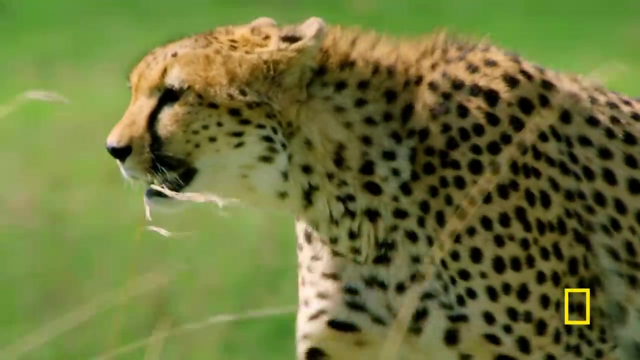 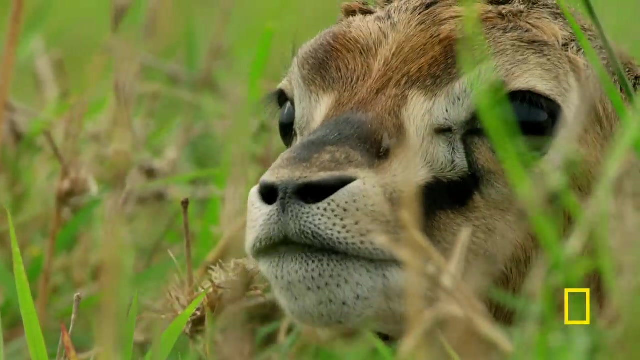 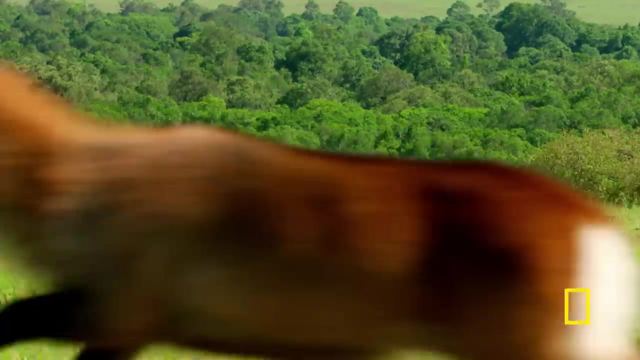 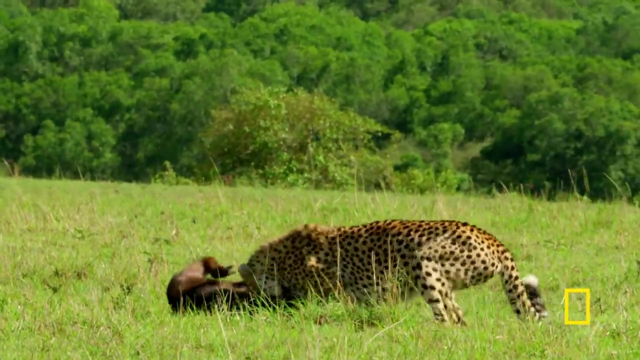 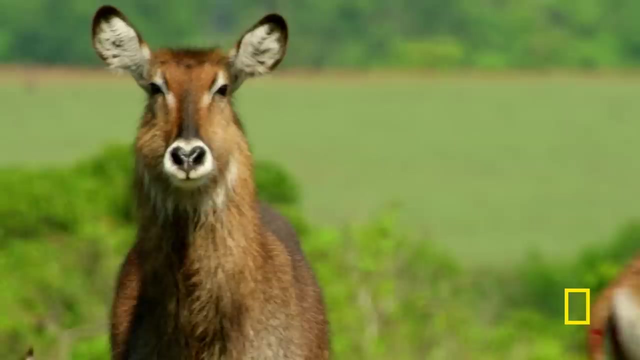 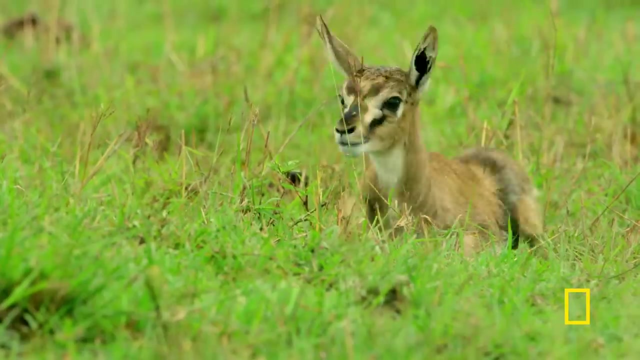 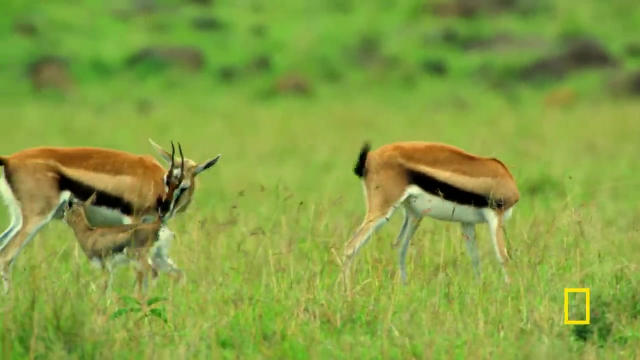 Oh, Oh. A Distraction and a narrow escape. a Waterbuck calf One fawns, fate is another's fortune. Surviving its first 24 hours is the greatest challenge the form will face. 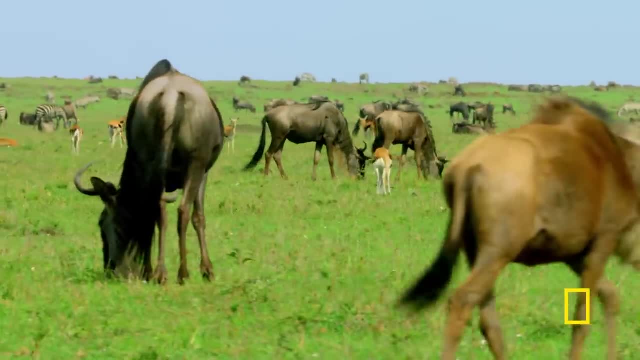 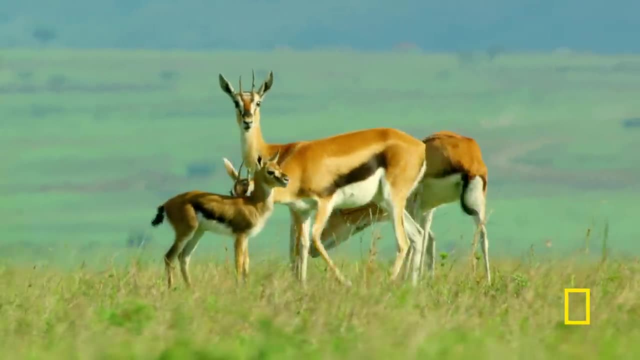 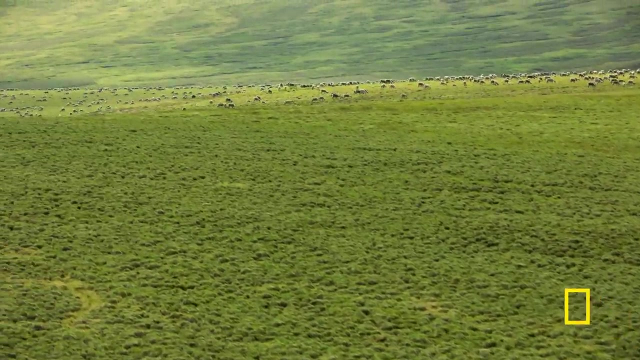 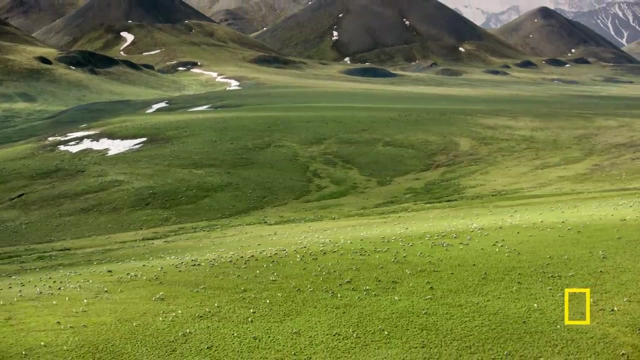 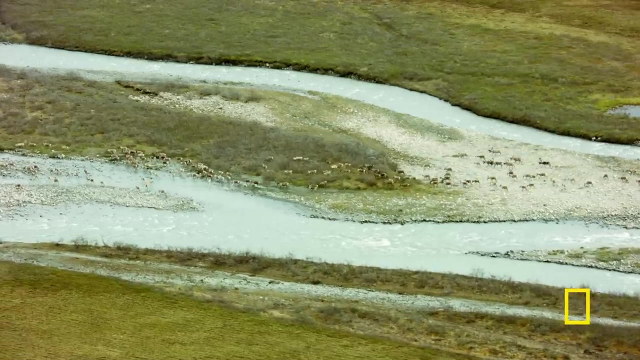 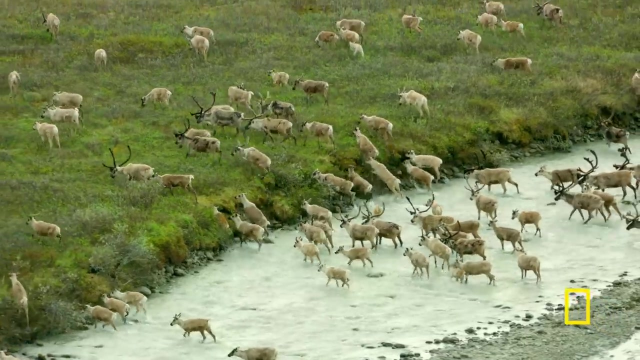 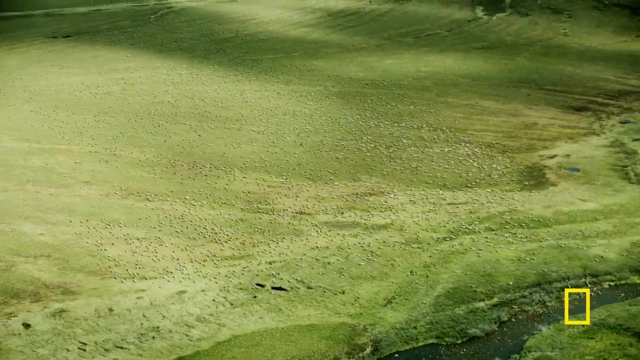 Those that make it can enjoy growing up on one of the most productive places on the planet. North America's grasslands support three million caribou. They journey up to 3,000 miles a year- the longest land migration on Earth. a Tom, most of the continent. mega herds are a thing of the past. 60 million bison once thundered across these plains Hunting decimated numbers to just over 1,000 animals And And bison are still rare today. Midsummer Time to fatten up before next winter, But that's getting harder. Temperatures here have risen three times more than the global average. 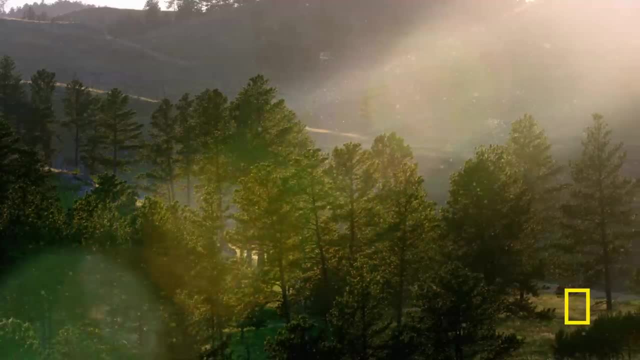 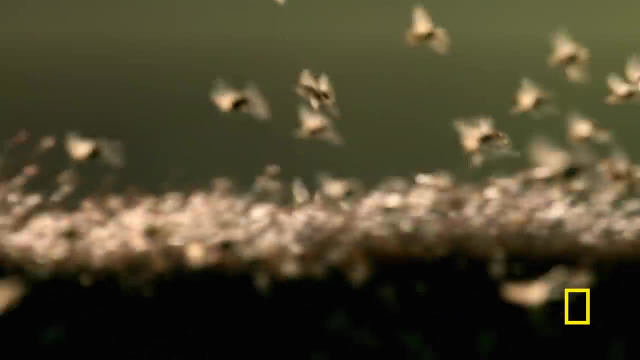 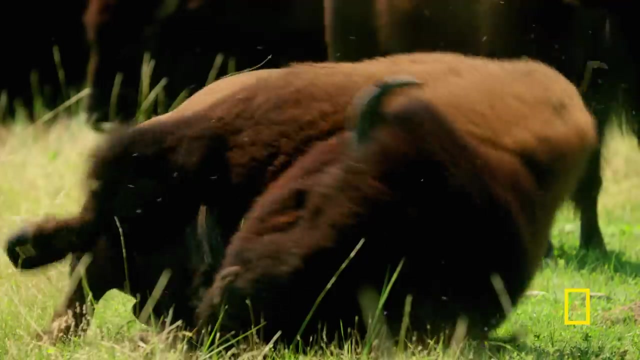 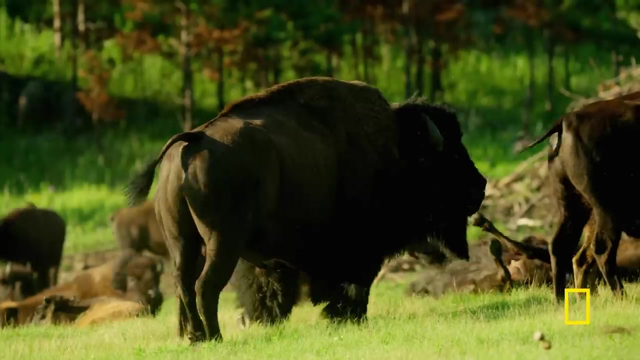 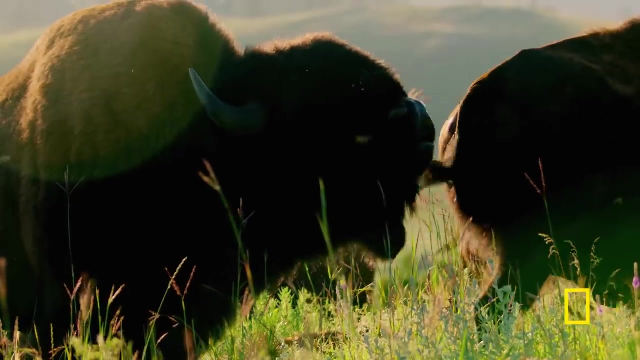 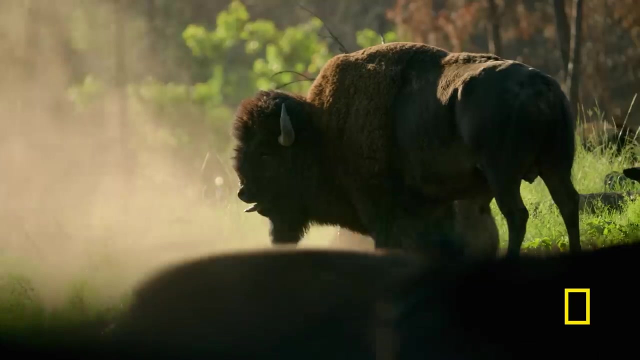 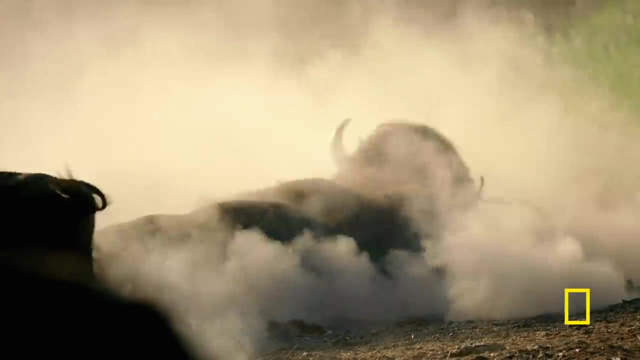 And it's creating plagues of biting flies. Each bison loses as much as a pint of blood every day, And just when the bulls need to be at their strongest to compete for mating rights. The winner will sire up to three-quarters of next year's calves. 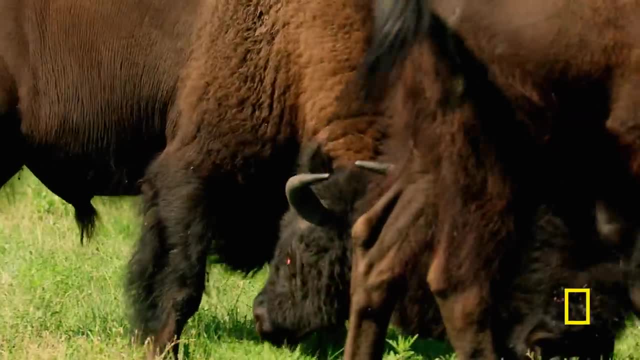 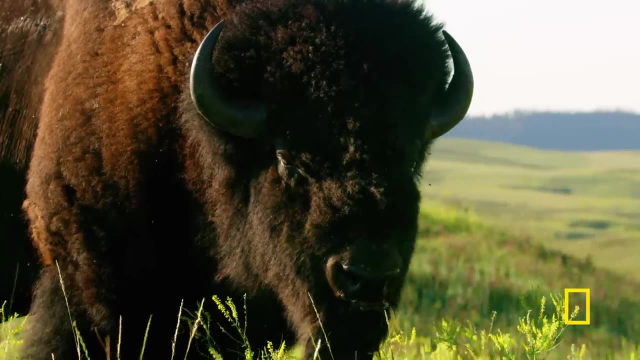 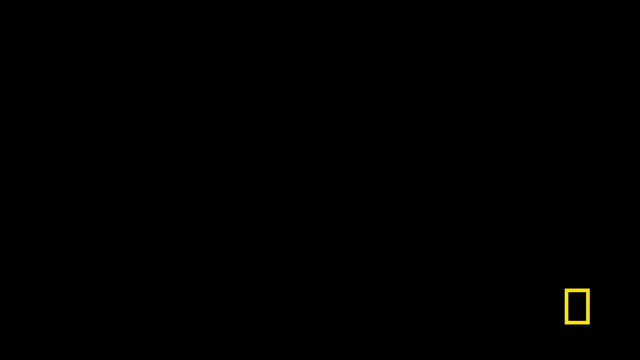 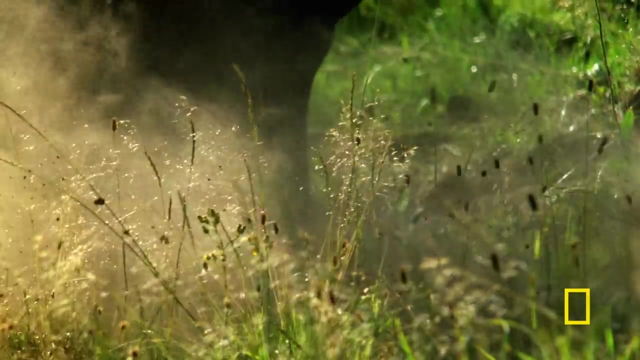 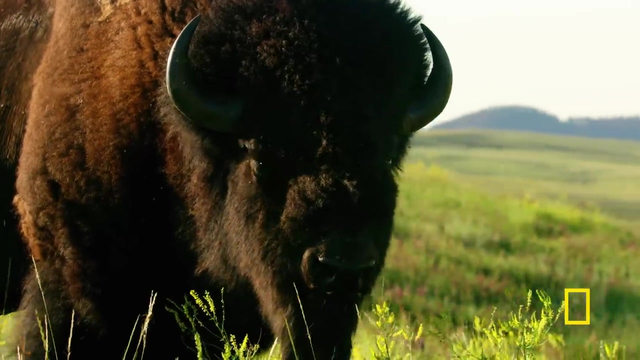 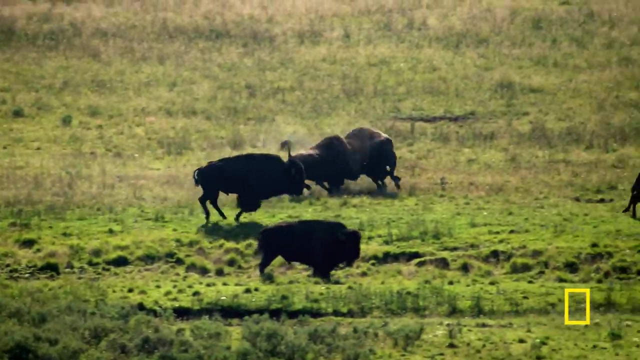 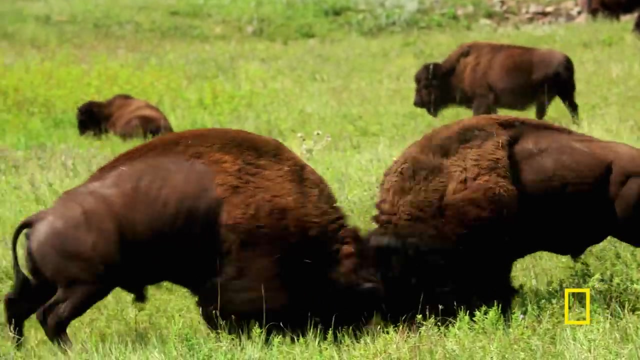 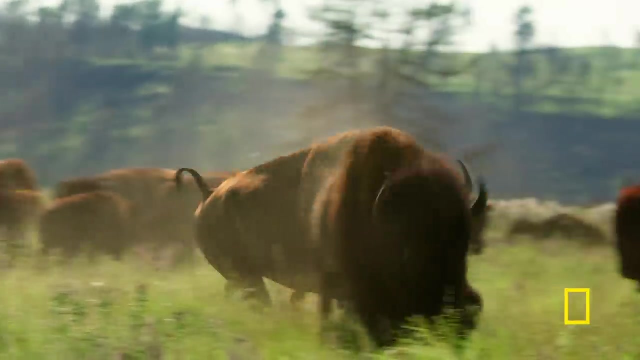 As the young bison scrap, An old bull watches on, Waiting for the perfect moment. Enter the arena. It's mating season. An old bull waits for a worthy challenger to emerge. The spring winds give a chance for the old bull to show up. 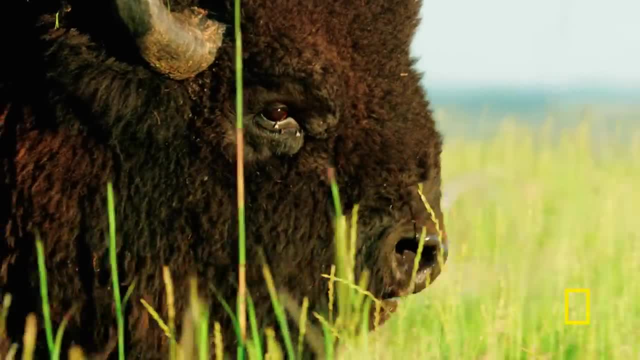 Fresh to the fight. the old bull enters the ring And the bitter battle has begun. The old bull has no one but the old bull. The old bull has no one but the old bull. You must not forget that. You must not forget that. 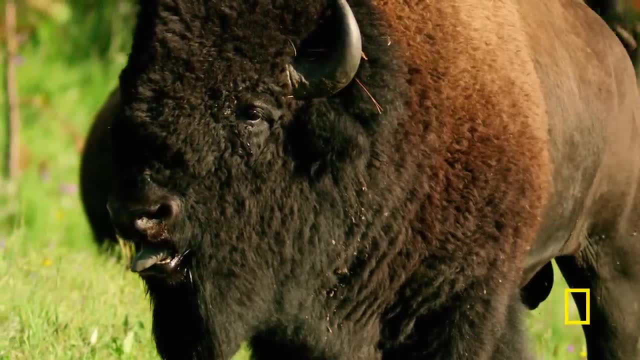 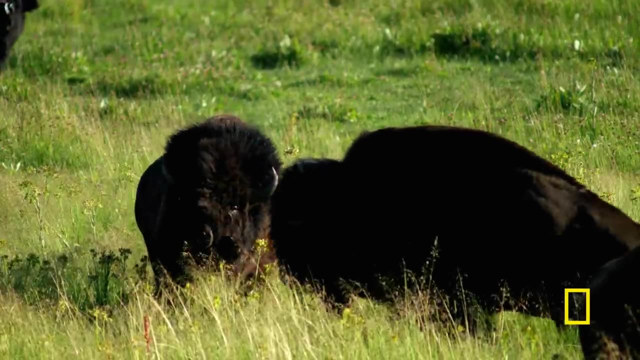 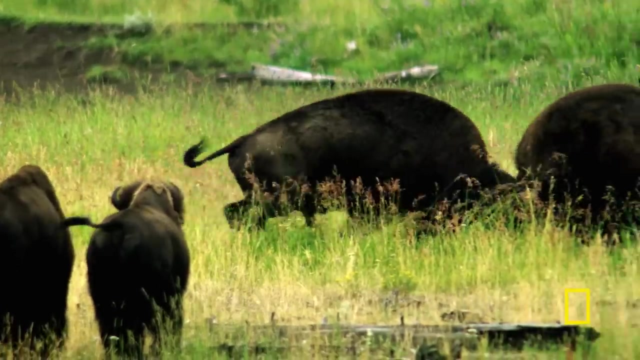 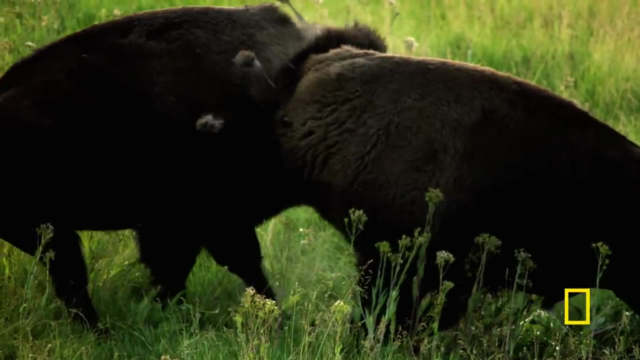 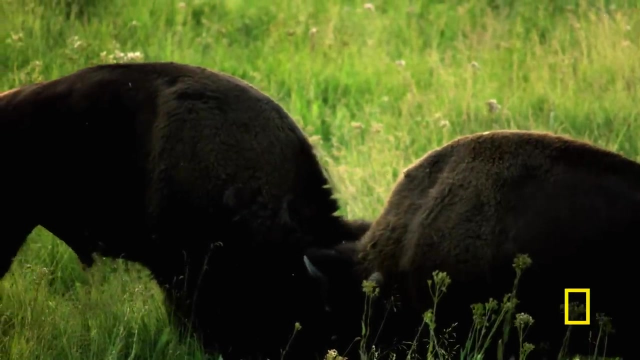 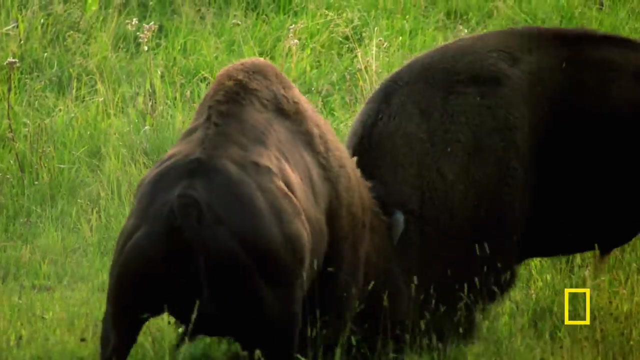 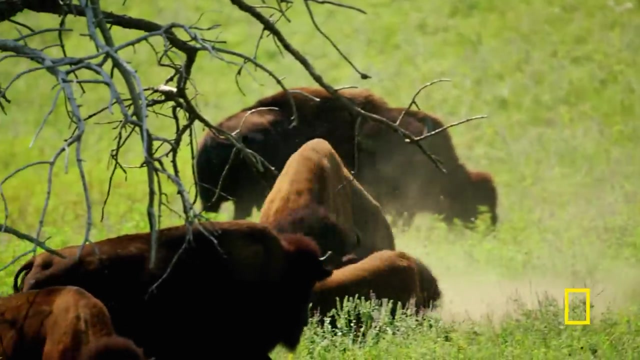 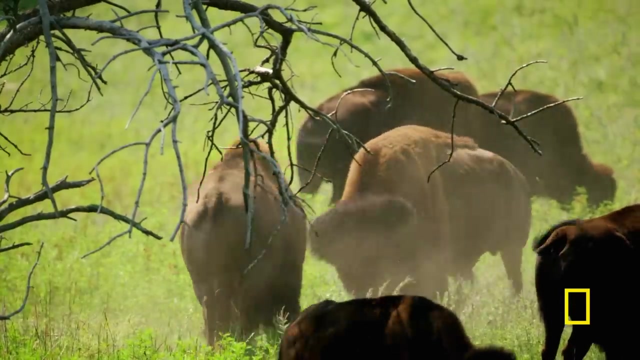 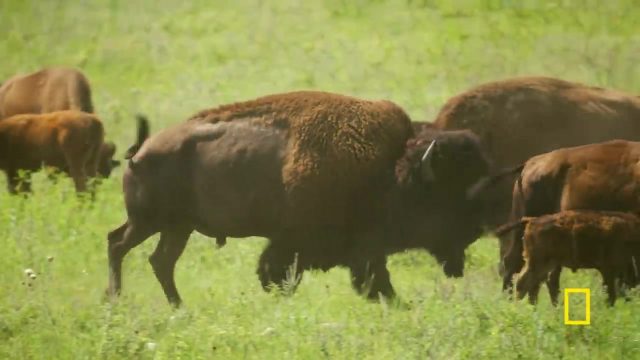 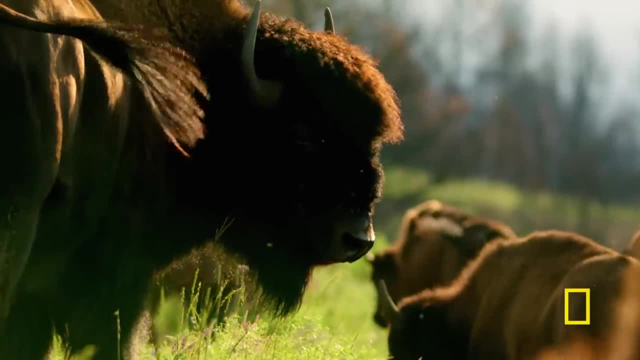 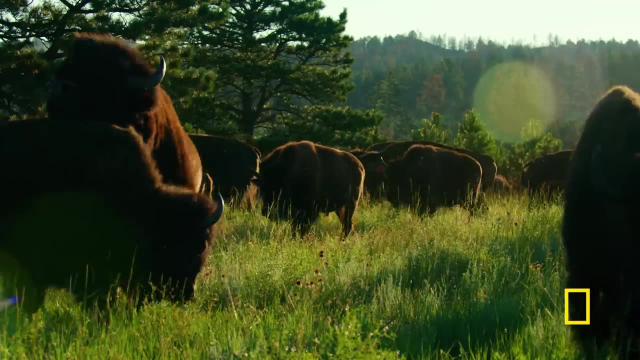 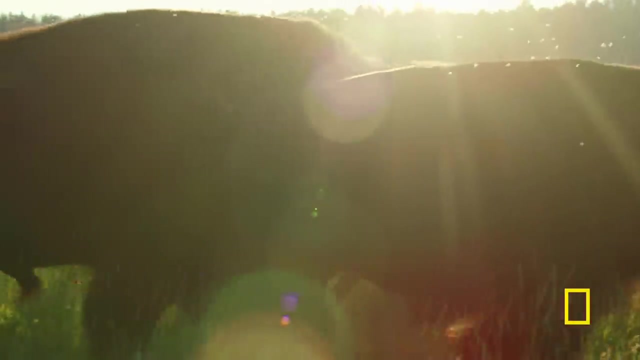 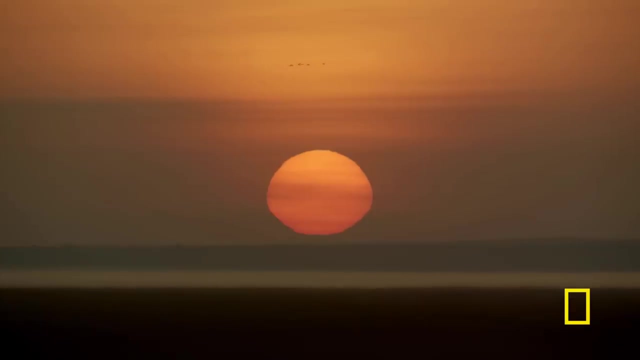 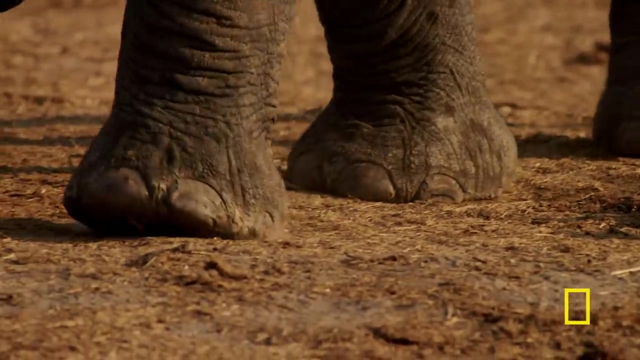 The youngster is more experienced, but the old bull is more experienced, but the youngster is more experienced. The old bull can enjoy the good times. The old bull can enjoy the good times, but they won't last long. but they won't last long. The dry season begins. 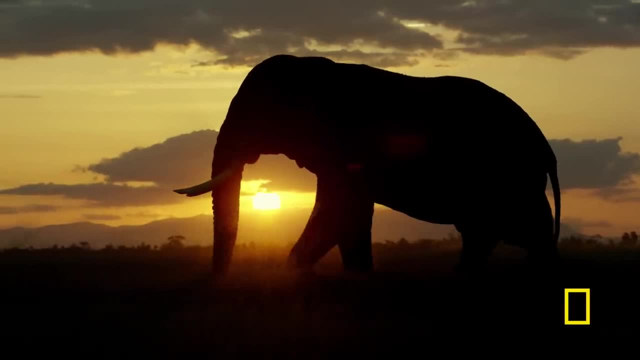 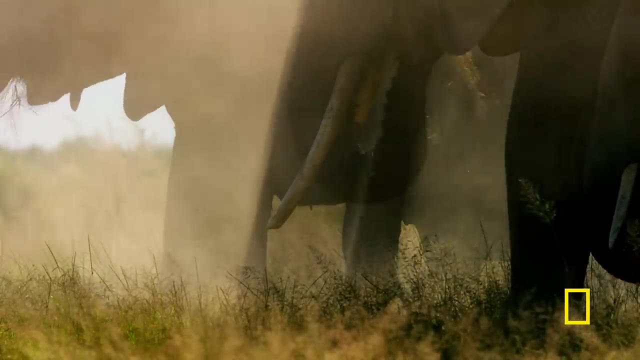 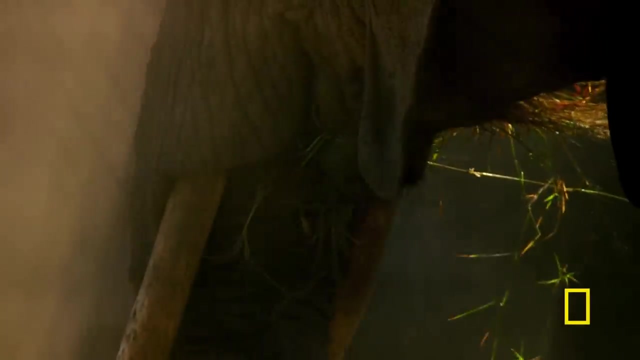 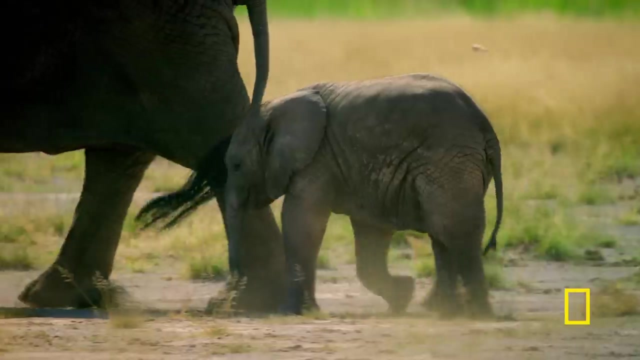 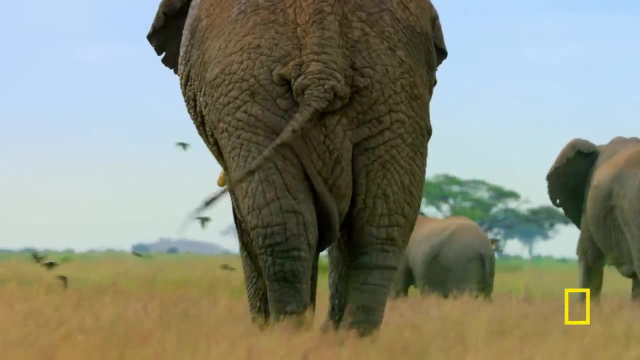 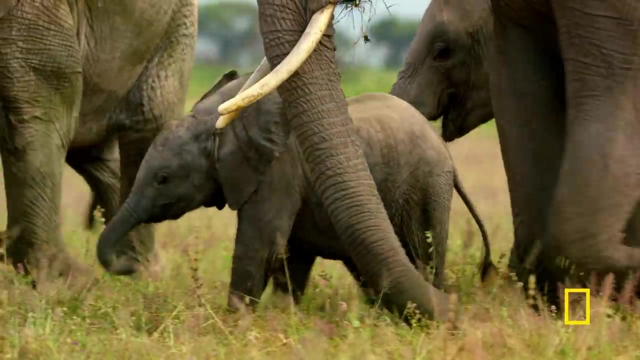 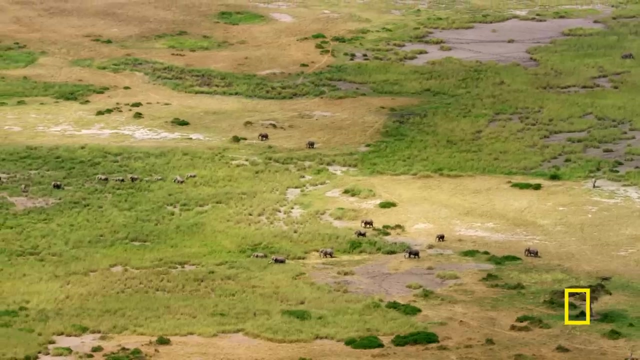 From now on, life just gets tougher. Grass becomes less nutritious And elephants struggle to satisfy their huge appetites. Like so many grassland animals, their only option is to keep moving. Elephants can walk over 100 miles a day in their search for food. 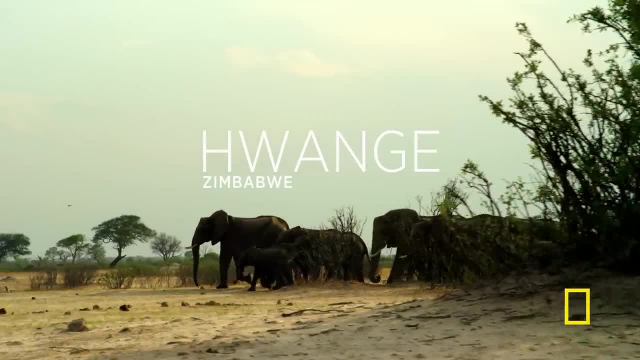 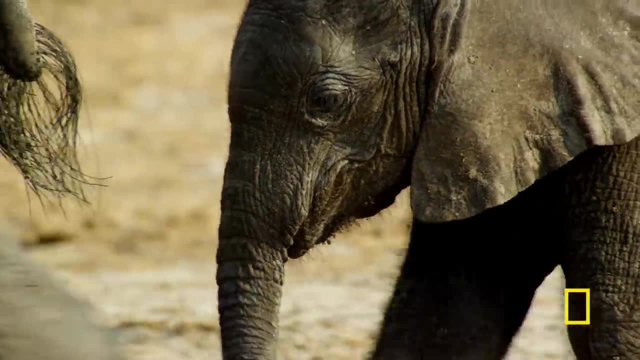 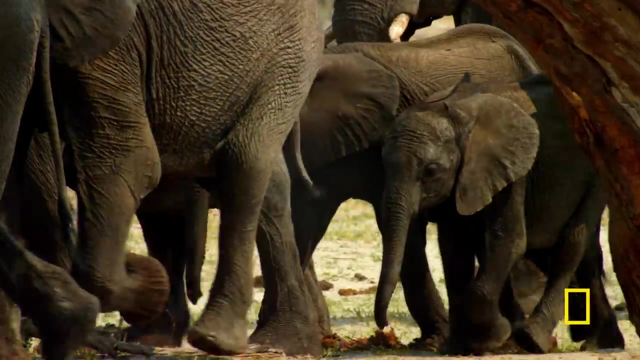 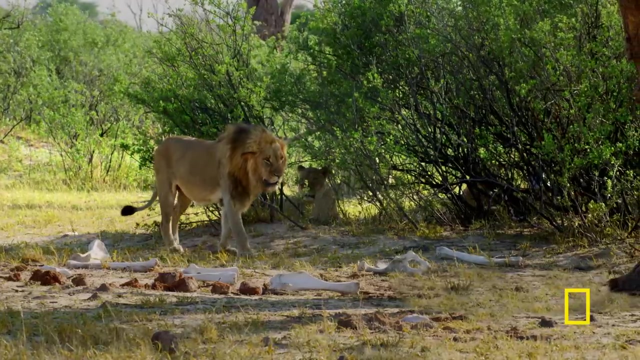 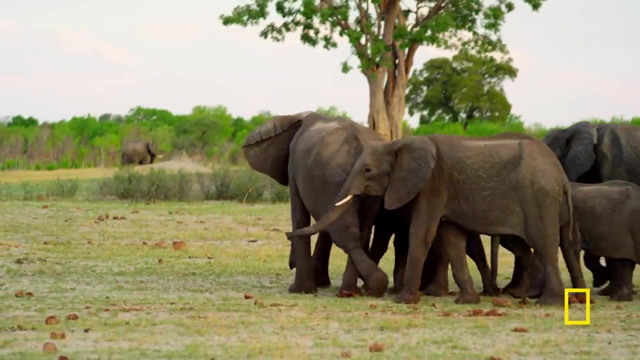 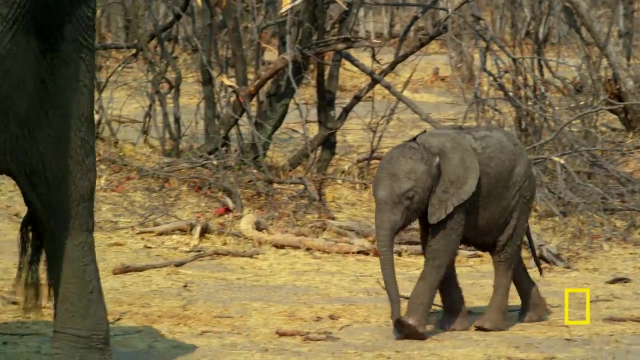 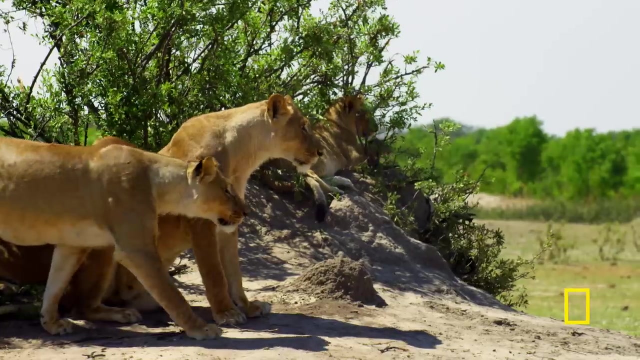 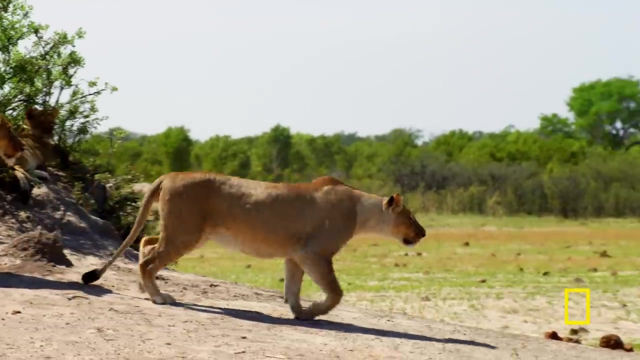 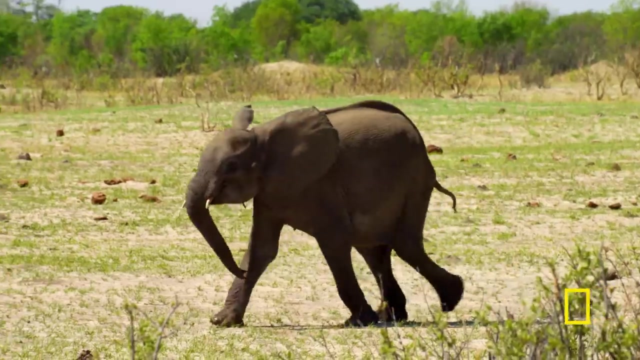 And it can lead them into dangerous territory. These lions specialise in bringing down large prey. Still it's risky, So they target the most vulnerable. Older calves should be safe. Moo Moo Moo, Moo, Moo Moo Moo. 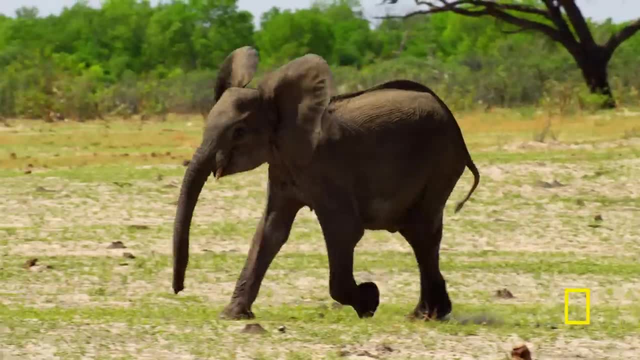 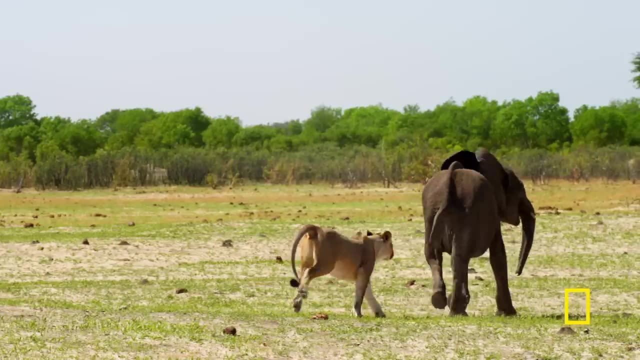 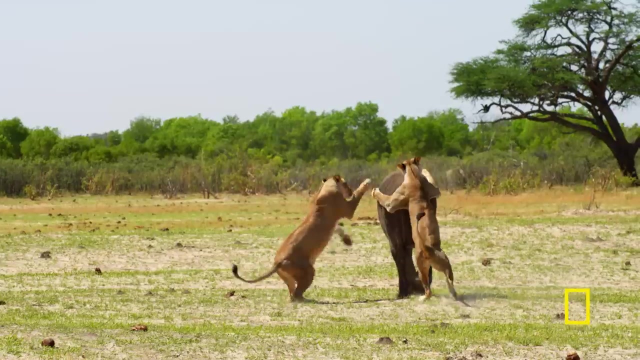 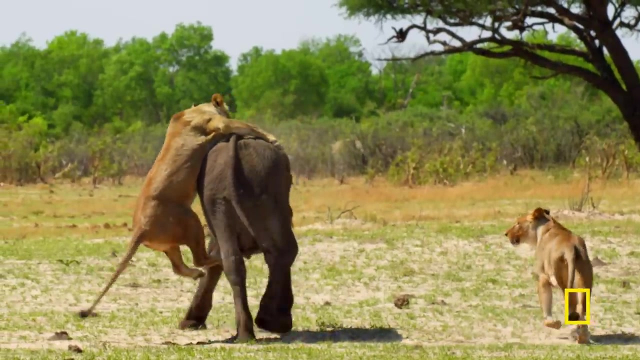 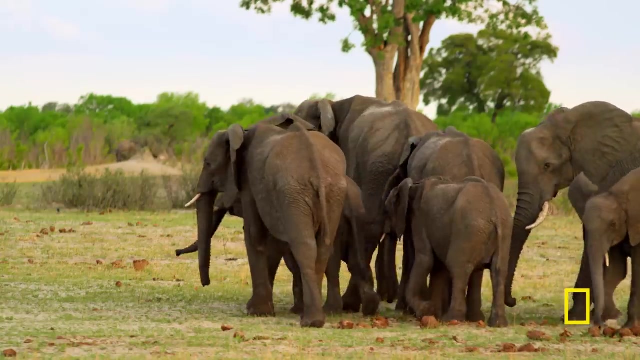 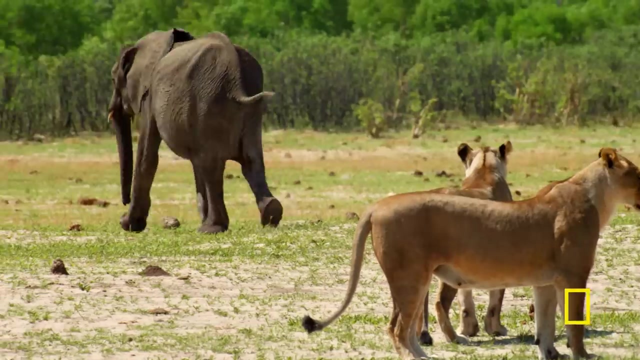 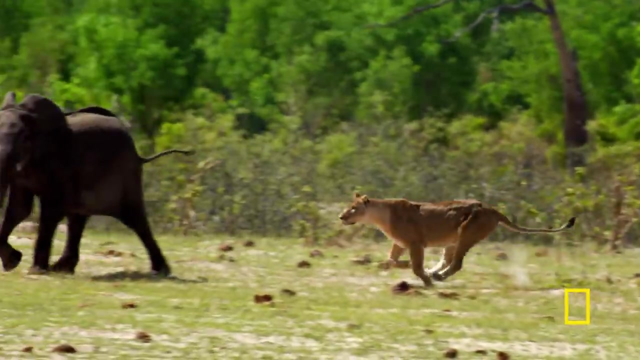 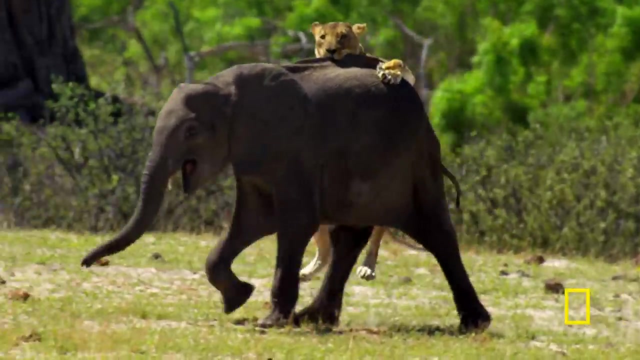 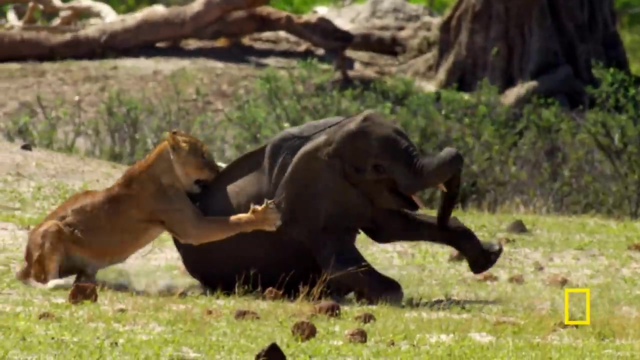 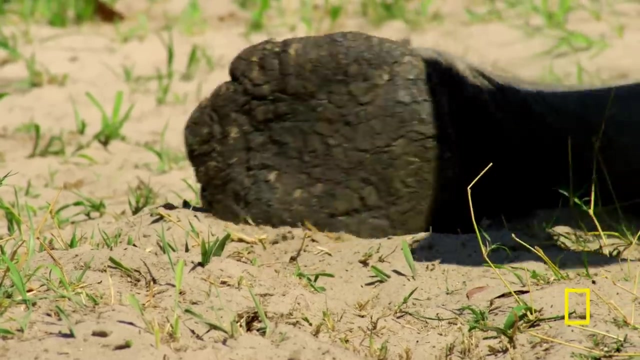 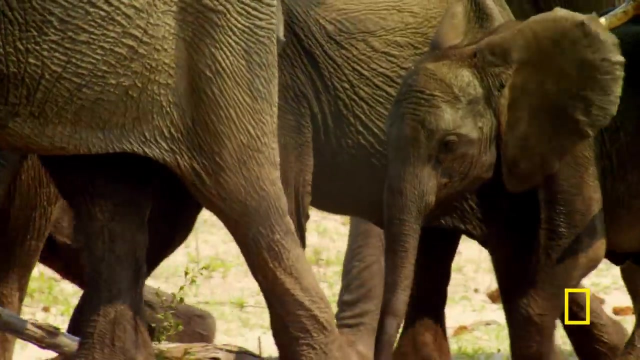 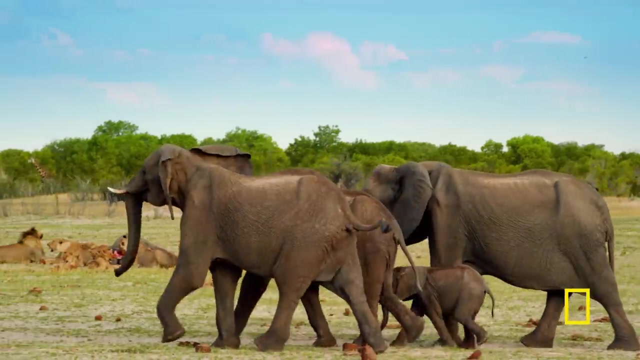 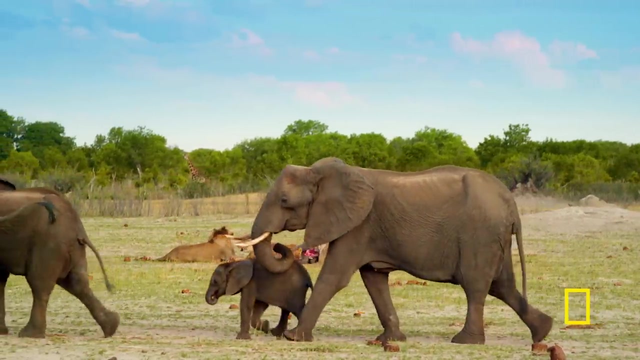 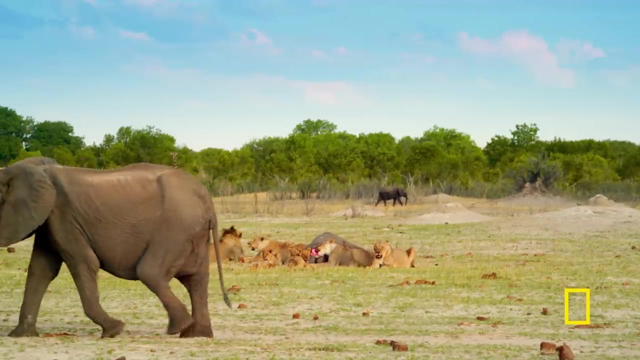 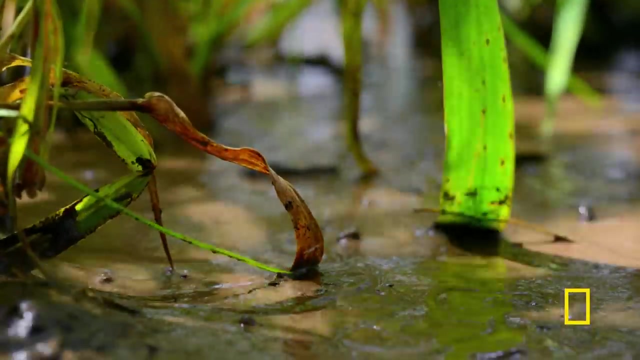 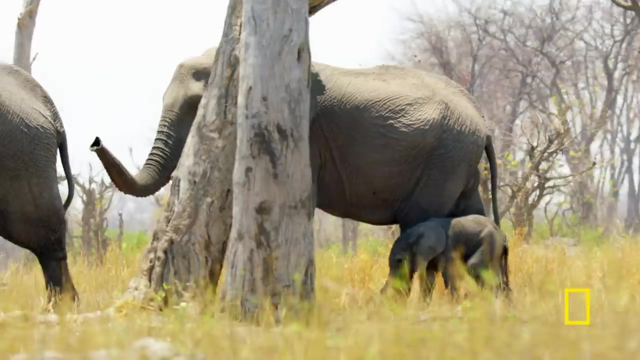 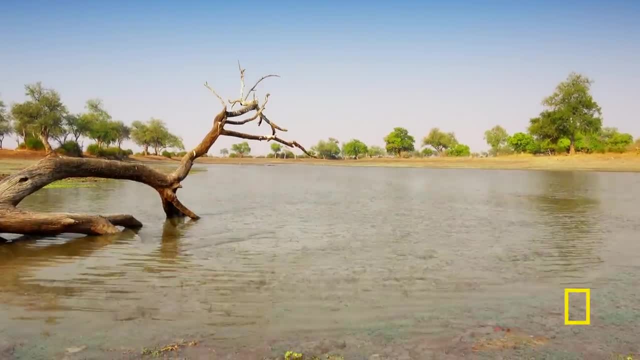 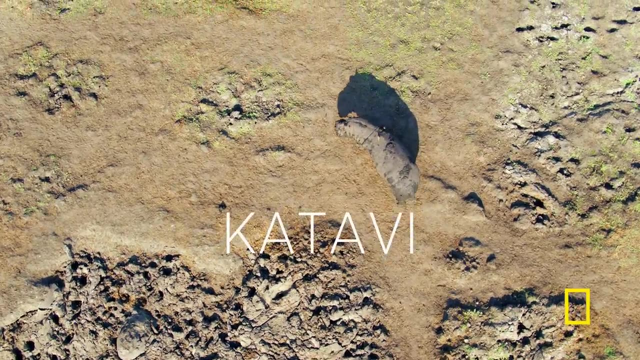 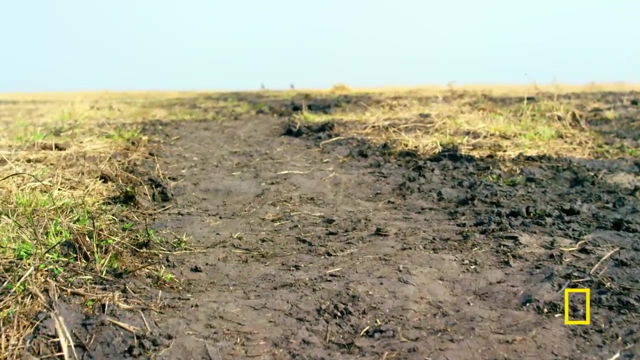 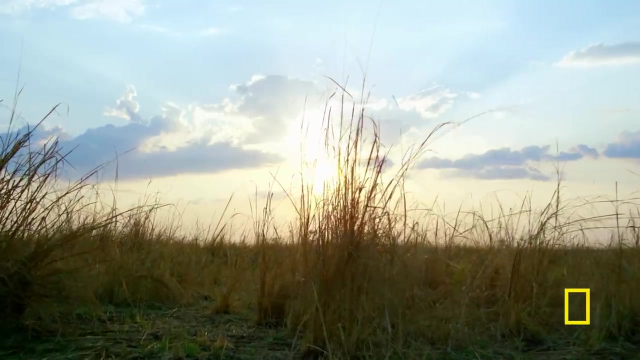 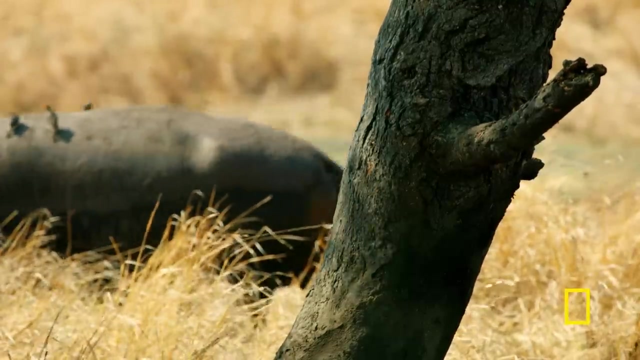 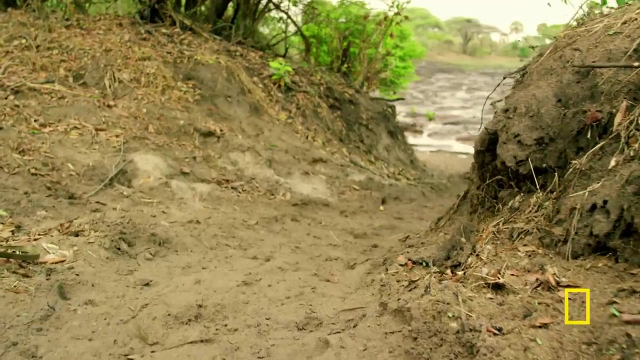 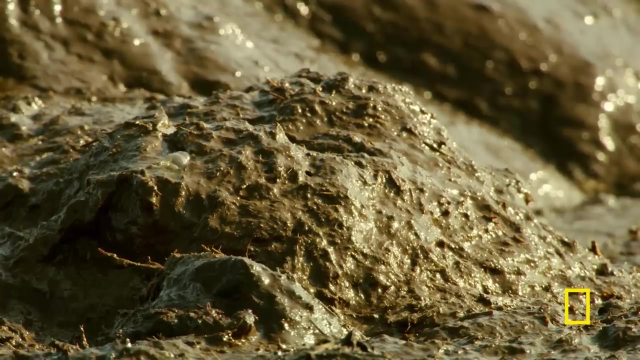 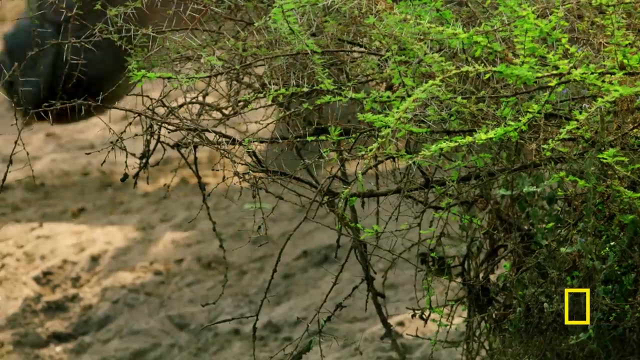 distant memory. Hippos suffer more than most. He spent the night grazing, but now the climbing sun is a threat. Hippos can quickly overheat. He needs deep water, and fast, Hippos. There is one pool But it's occupied. 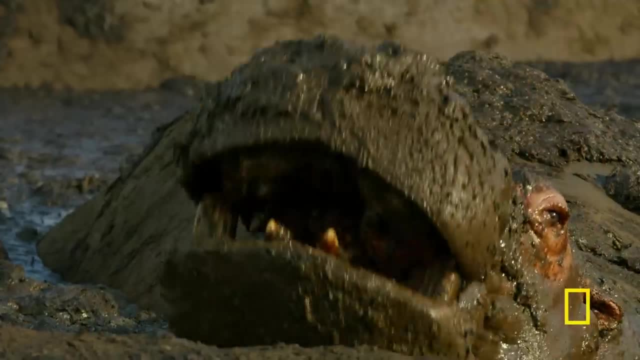 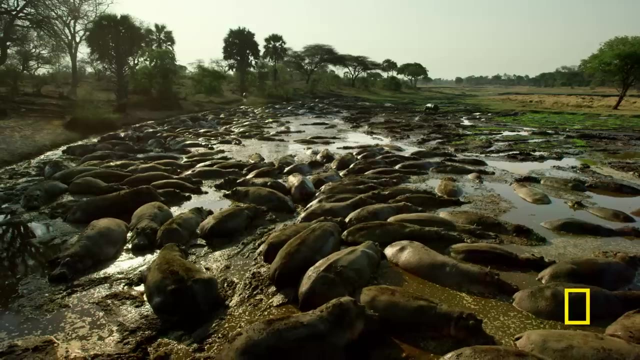 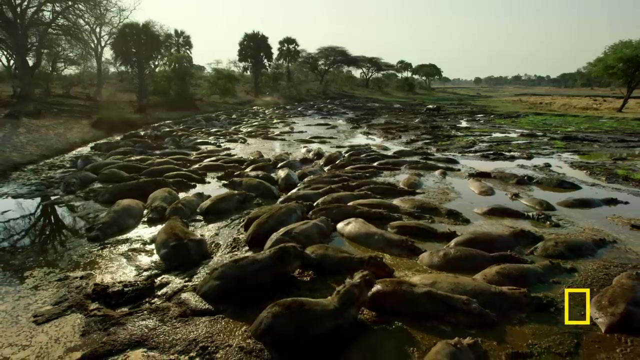 Each bull hippo normally commands a territory of 200 feet Hippos. The population of Visitipoma and Tripitaka is a country of heroes. Now, 800 of Africa's most bad tempered animals are crammed together and, as humans, take more. 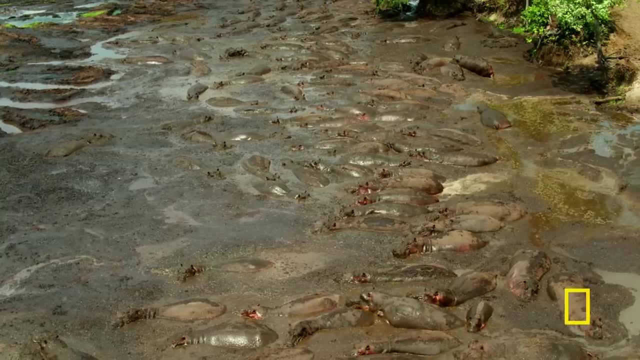 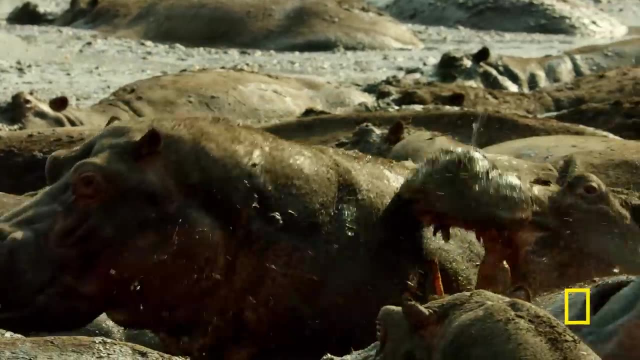 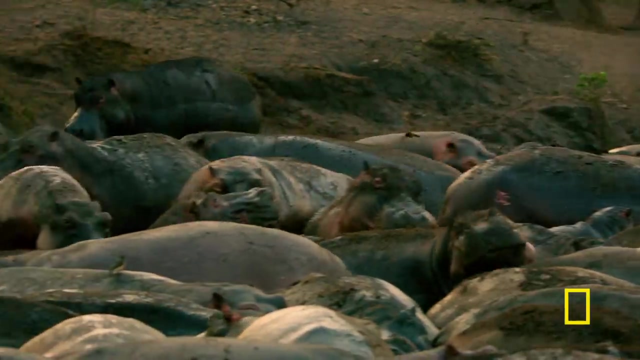 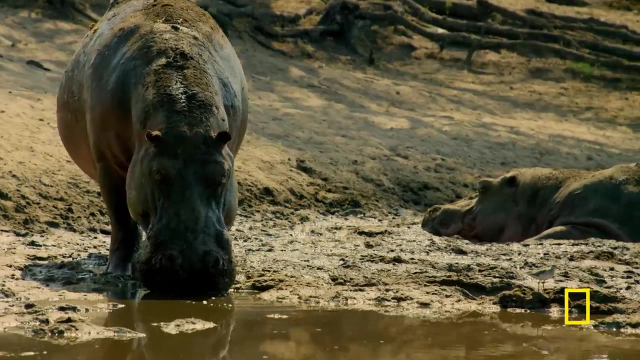 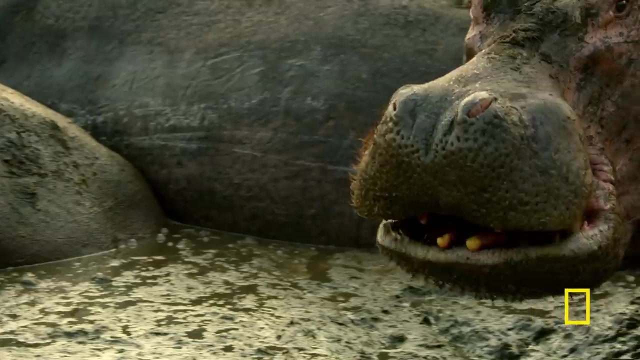 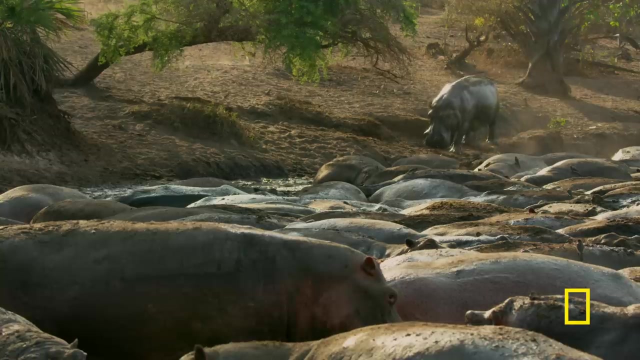 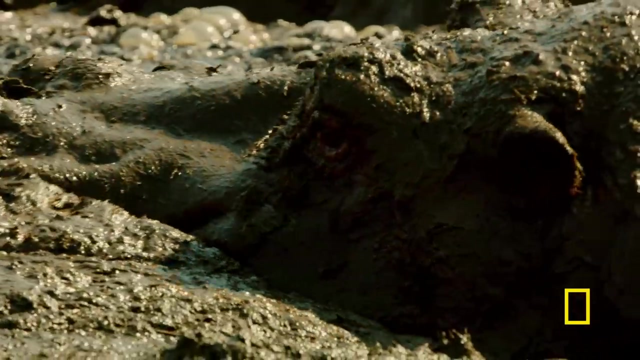 water for irrigation. there's less room than ever before. Hippos, Hippos, Hippos, Hippos. Somehow he's got to find a way in His life depends on it. Out of water, this hippo would soon overheat. 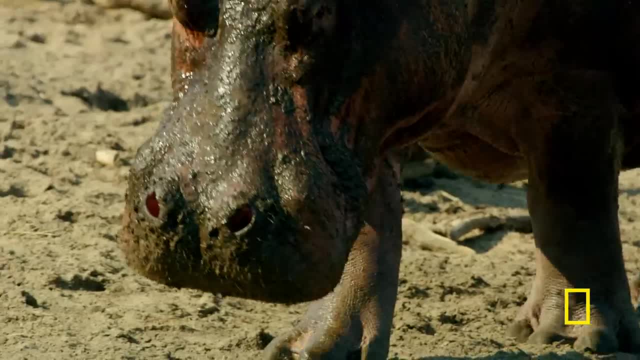 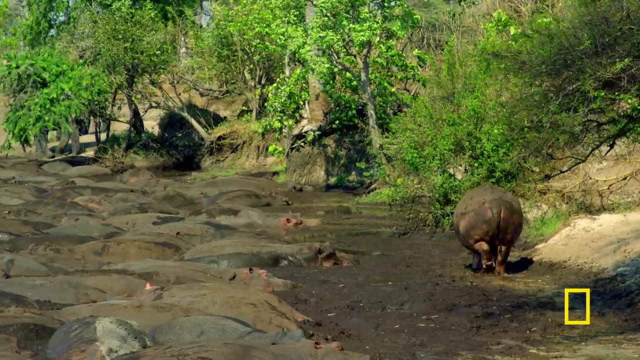 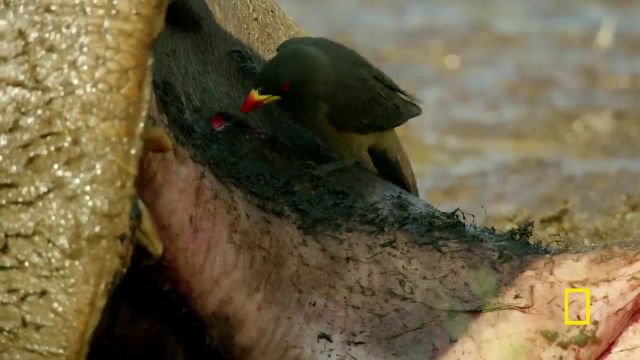 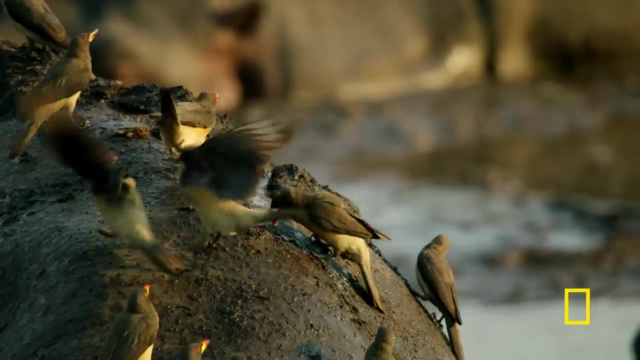 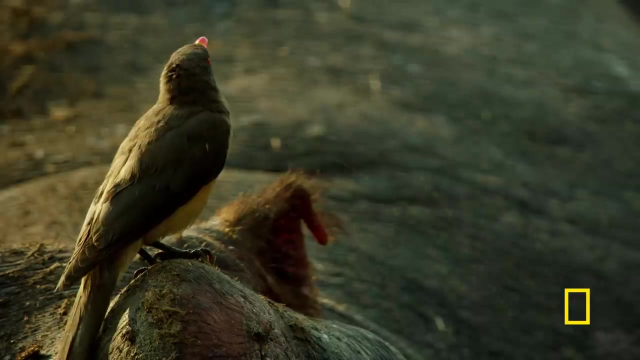 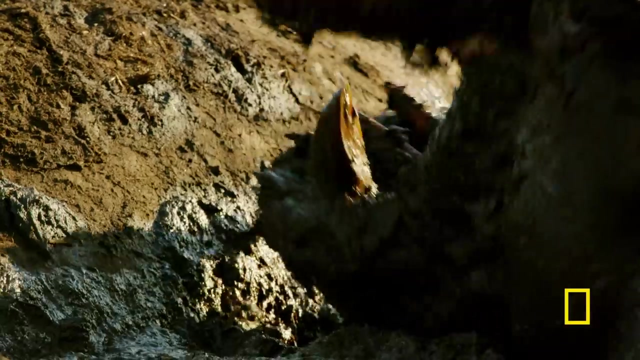 But the water hole is already full. It may not look very inviting. Oxpeckers ravage cracks in their delicate skin. How clever, and 20 tons of waste a day has turned it into a cesspit, But this hellhole could save his life. 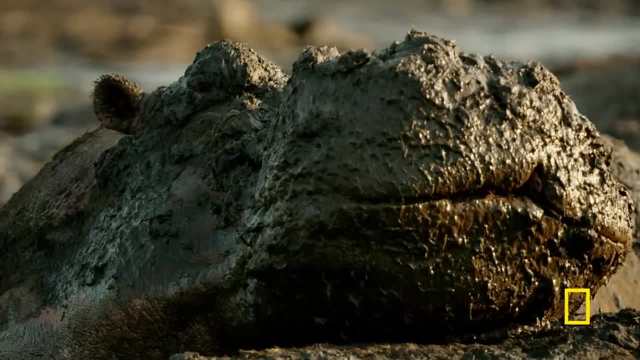 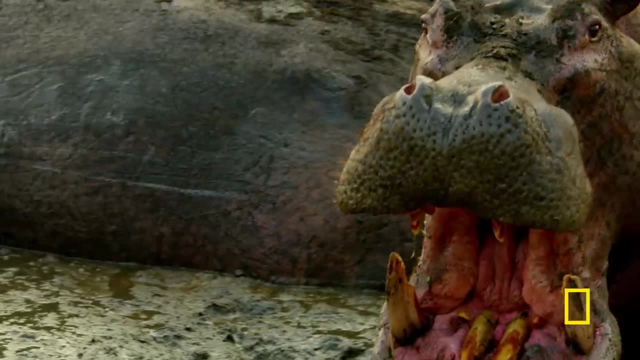 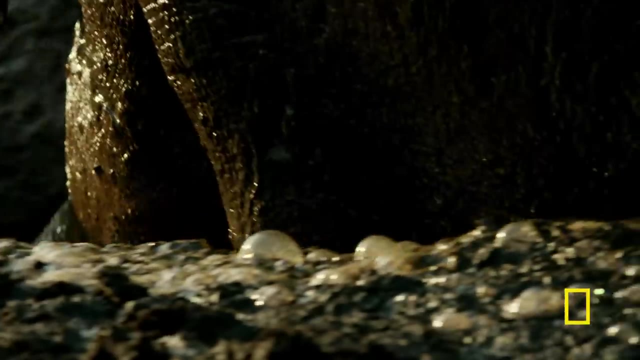 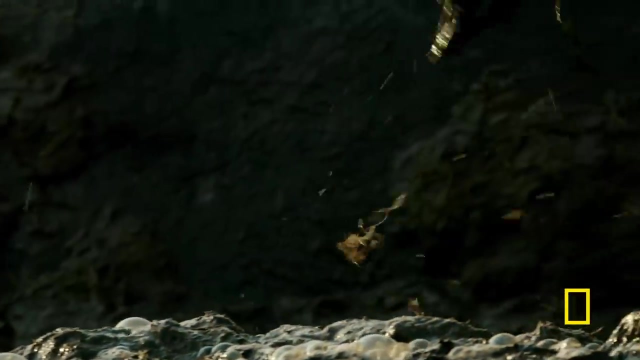 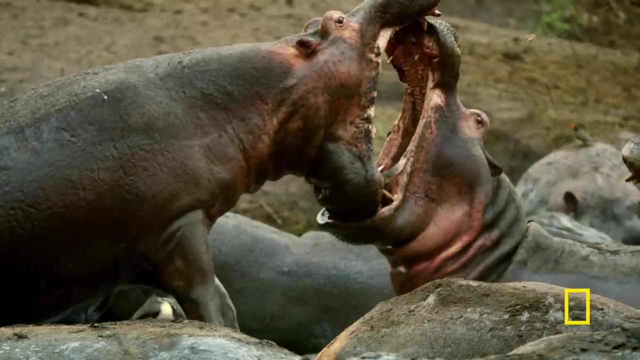 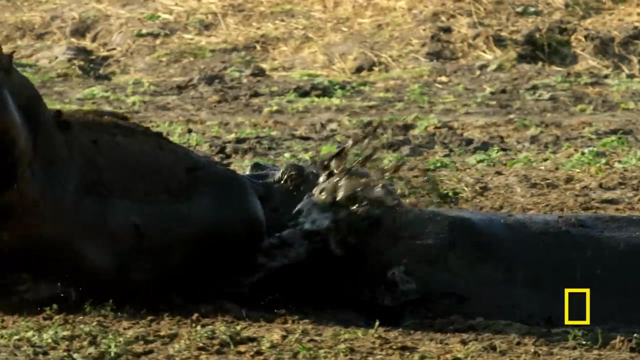 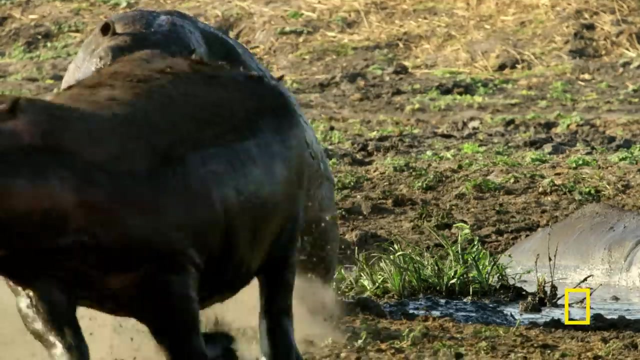 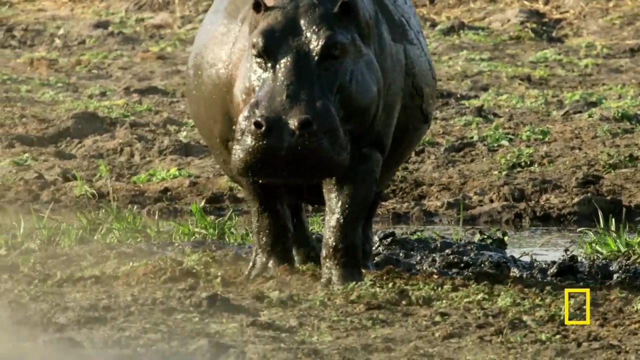 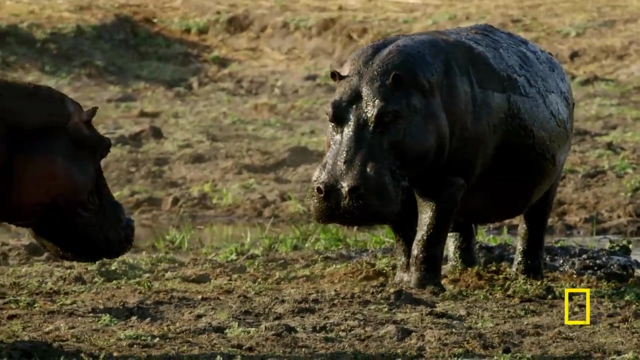 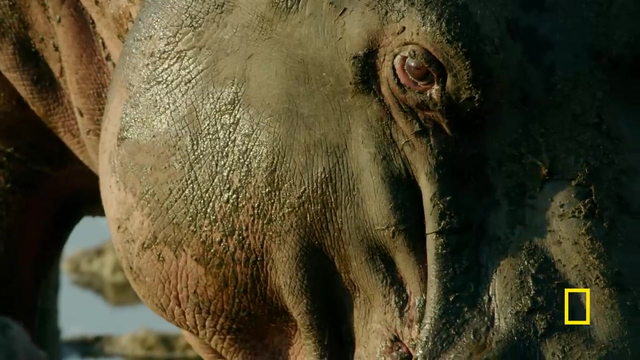 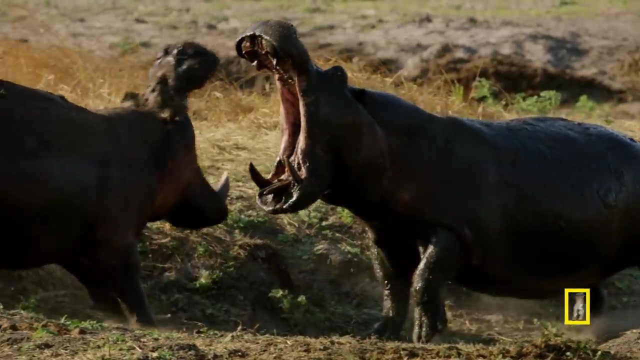 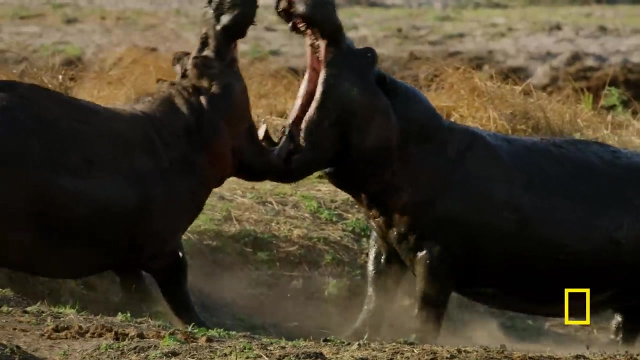 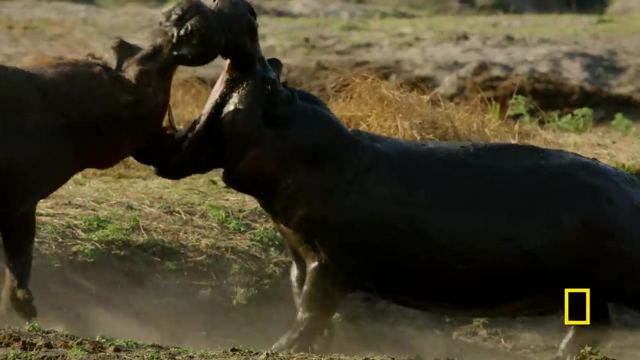 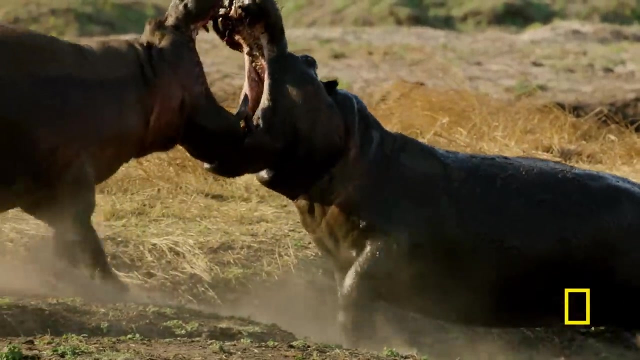 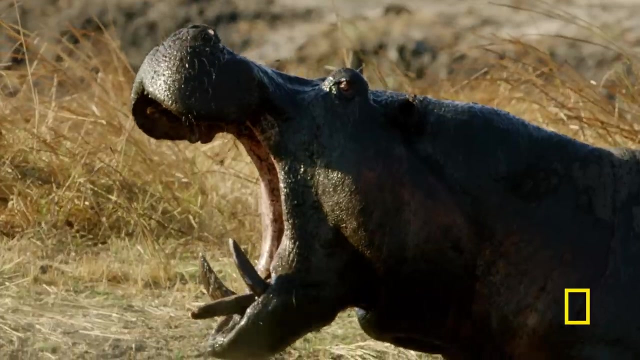 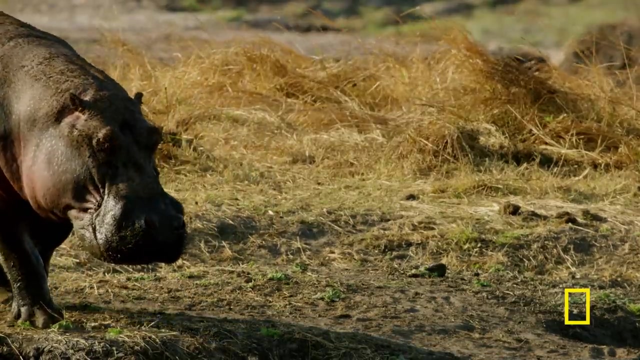 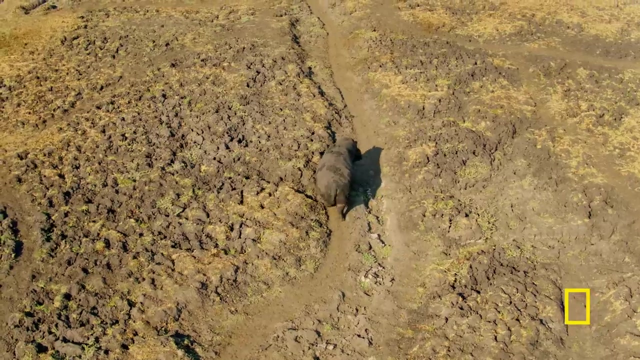 If he's allowed it. If he's allowed it, This resident bull is bigger, But the outsider is desperate. Five tons of hippo clash Testing bulk Bite size And brute force. The outsider accepts defeat. He must venture into the unknown. 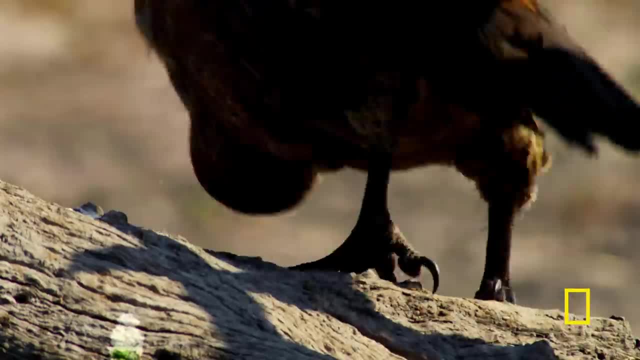 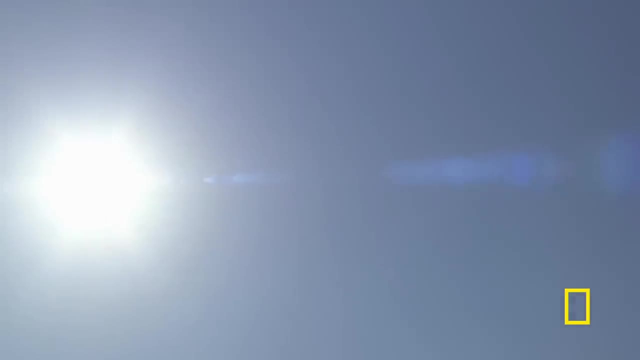 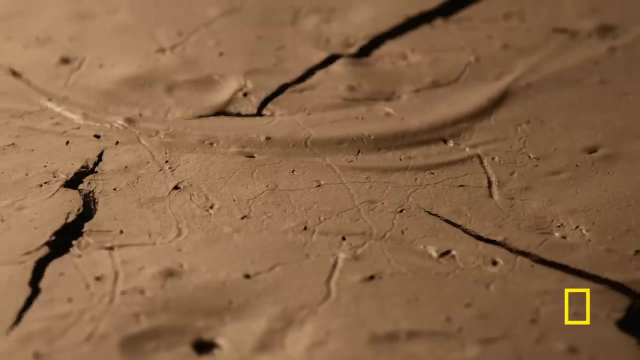 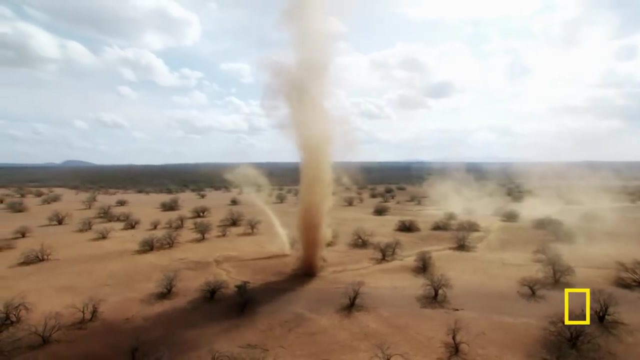 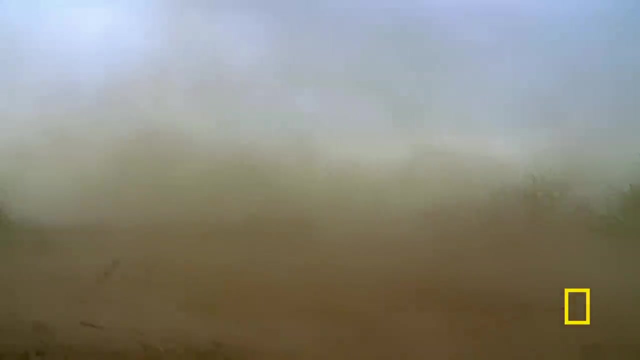 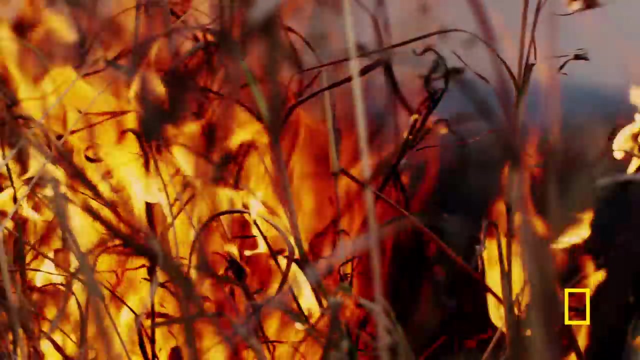 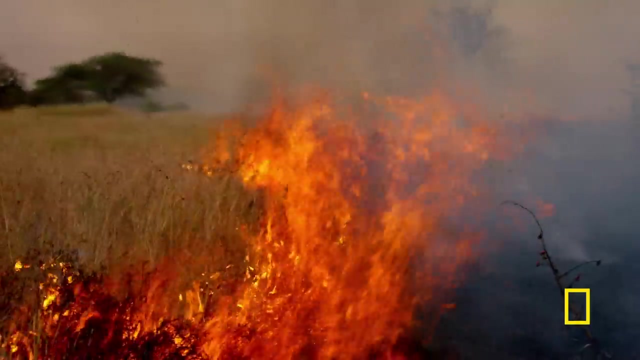 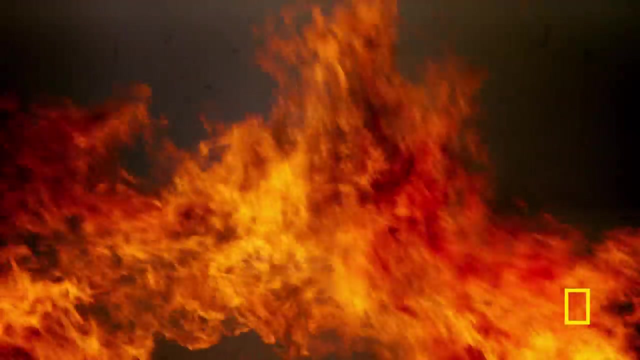 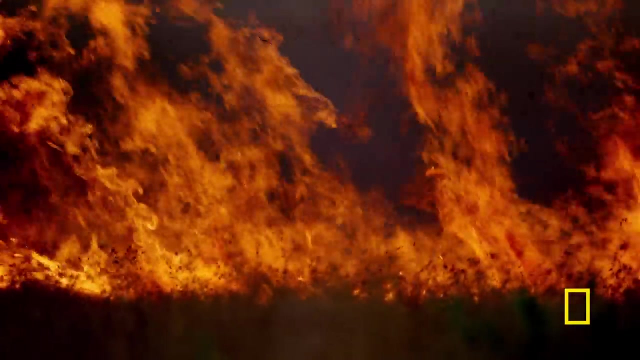 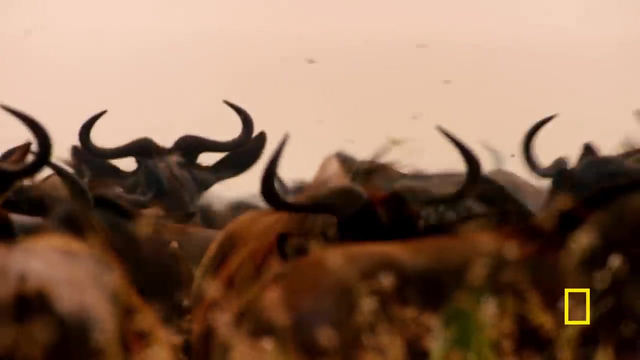 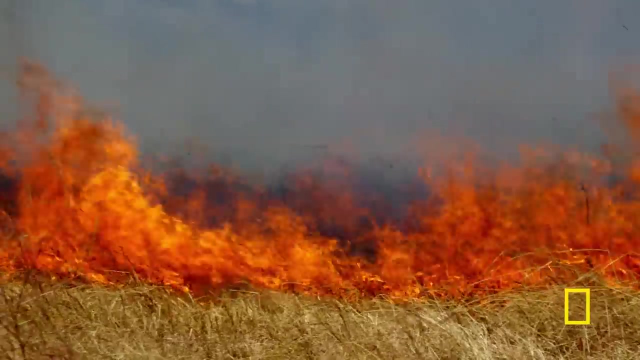 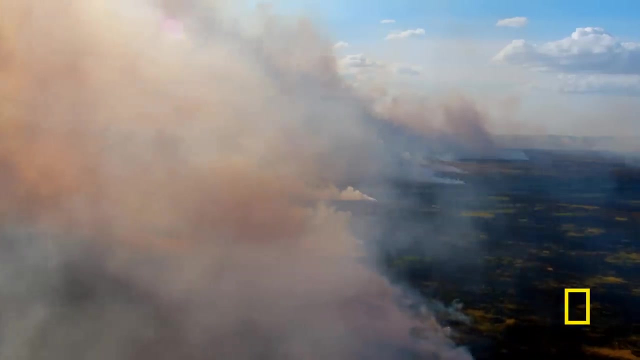 Drought, Drought, Drought. The Earth is parched and the grass tender. dry Fires can sweep across the plains at 40 miles an hour And reach temperatures of 800 degrees Across Africa, an area the size of half the United States. 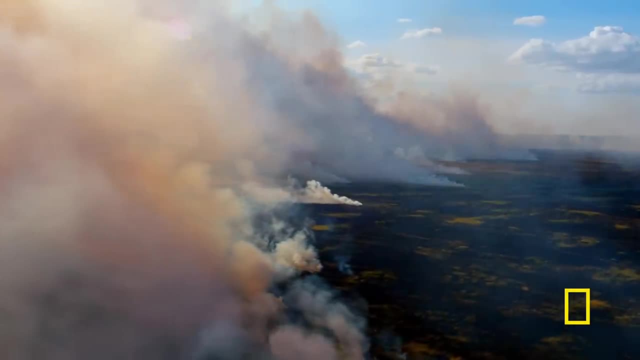 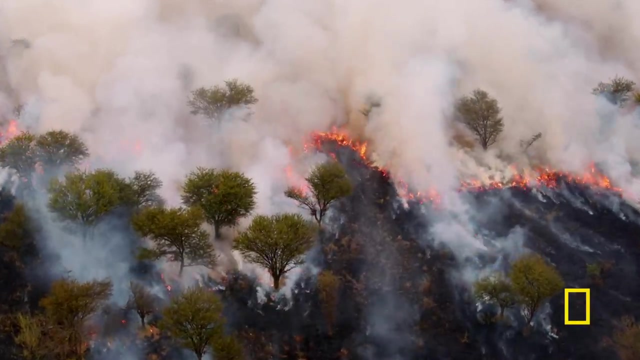 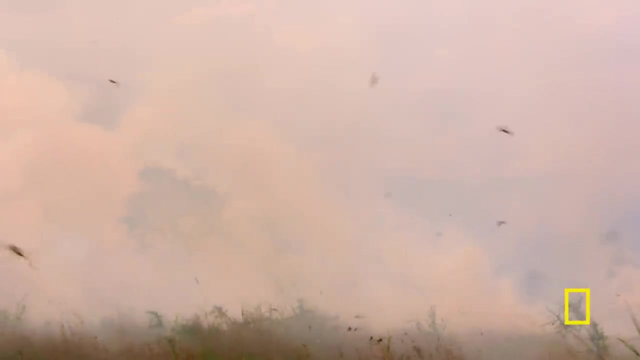 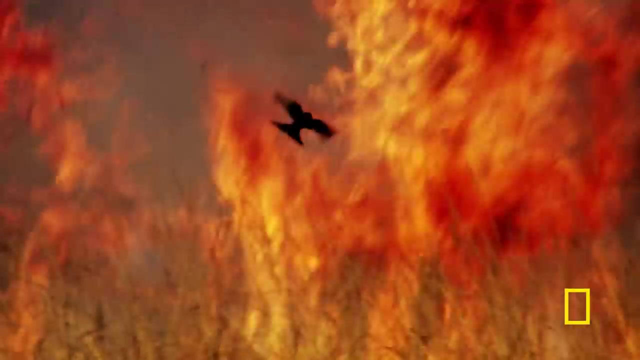 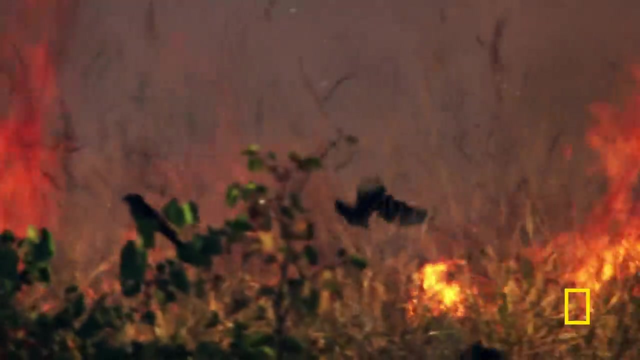 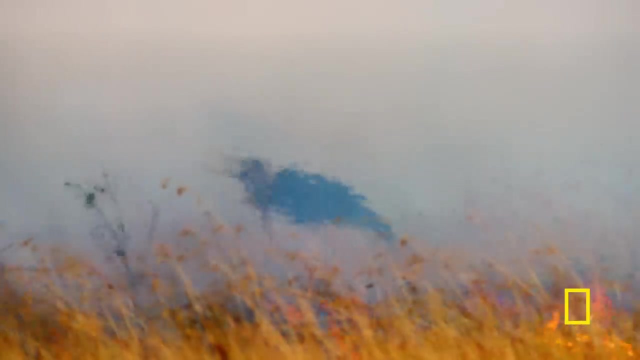 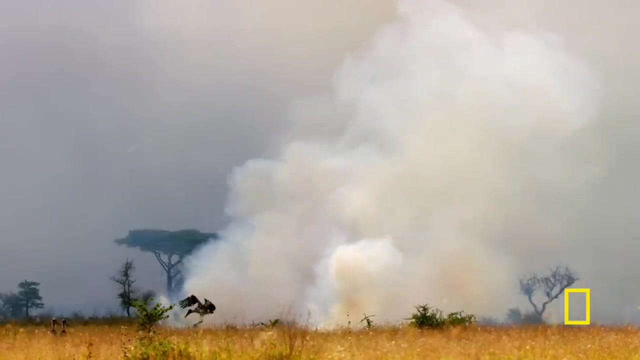 burns every year And with a warming climate, wildfires are set to spread even further. Third, marabou storks clean up afterwards. 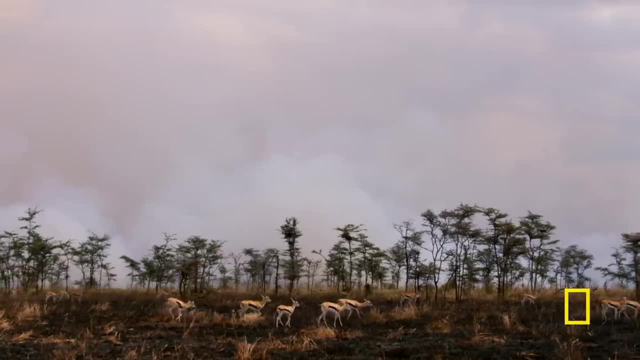 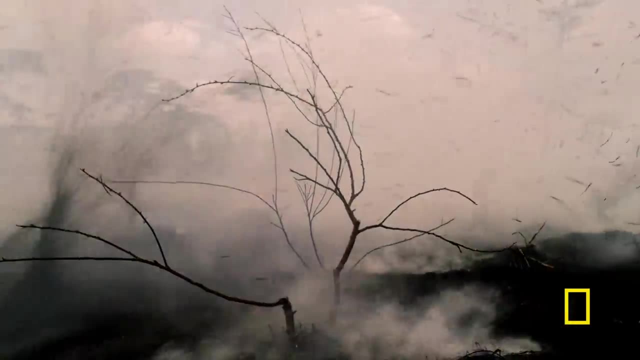 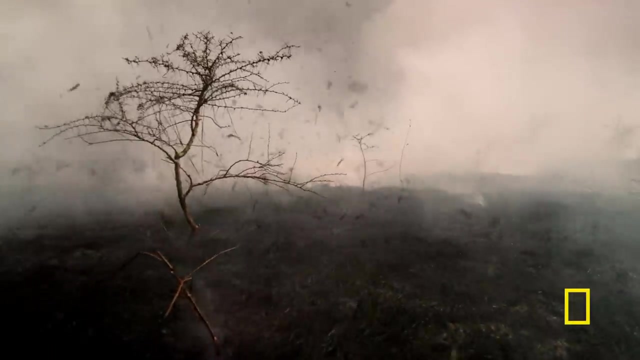 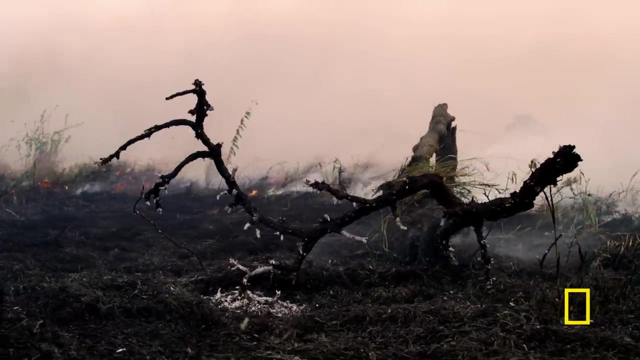 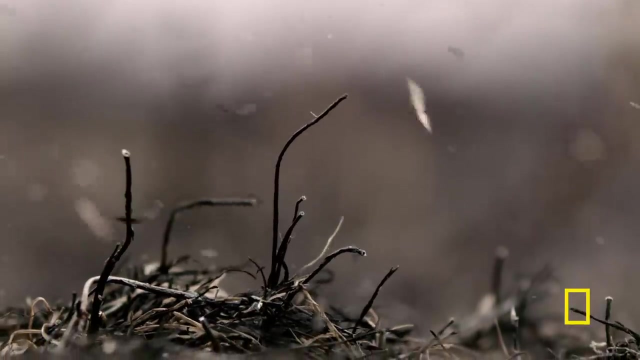 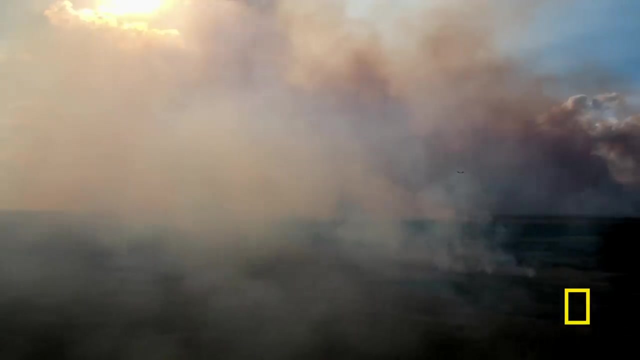 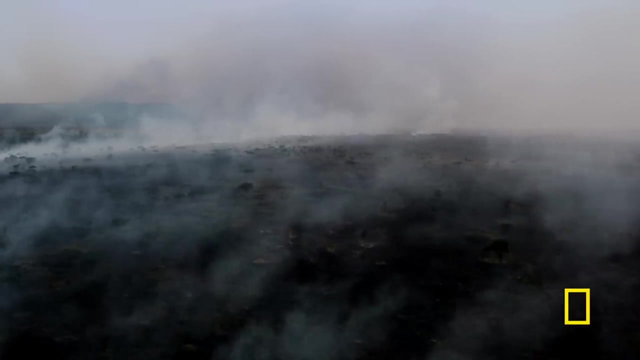 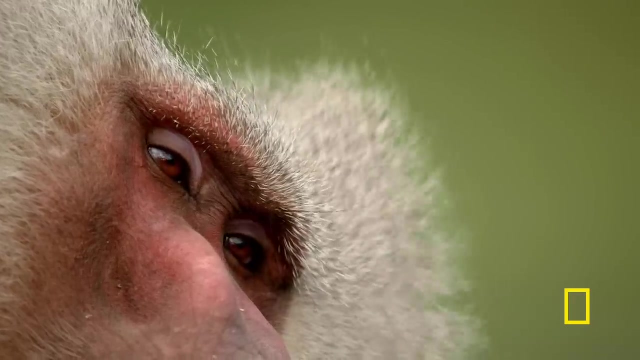 There's nothing left here for the graces, But the grass itself clings on its deep roots, untouched by the flames. All it needs now is water, But the grass itself clings on its deep roots, untouched by the flames. Hamadryas, baboons wait months for the rains to arrive. 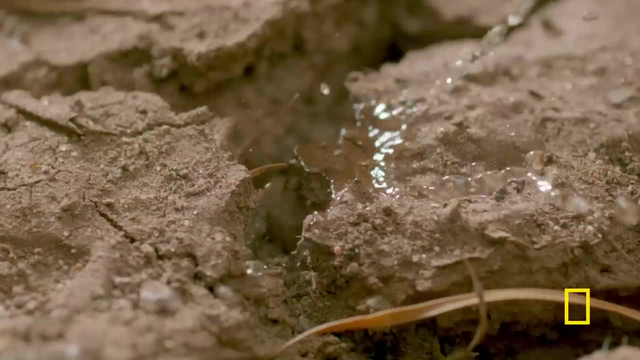 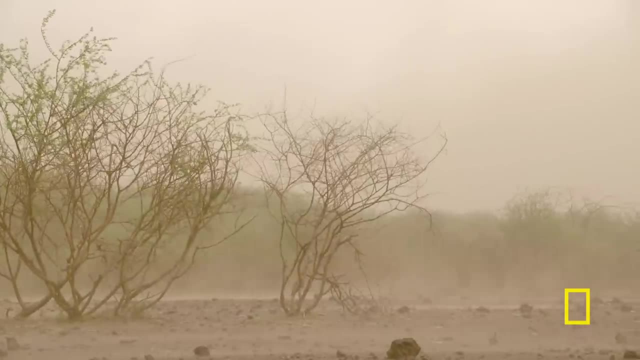 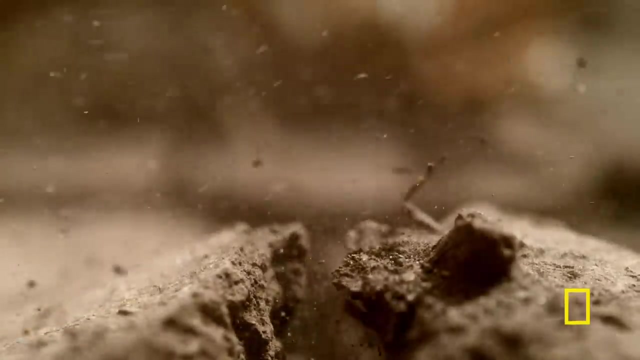 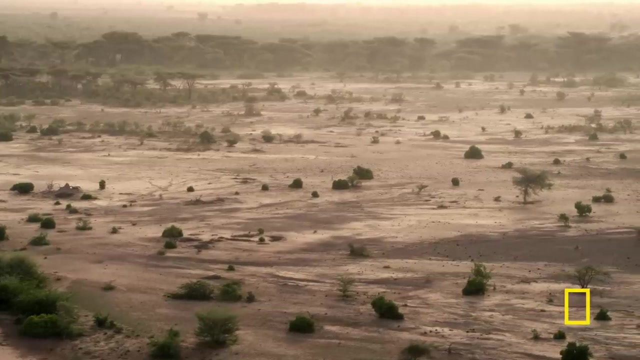 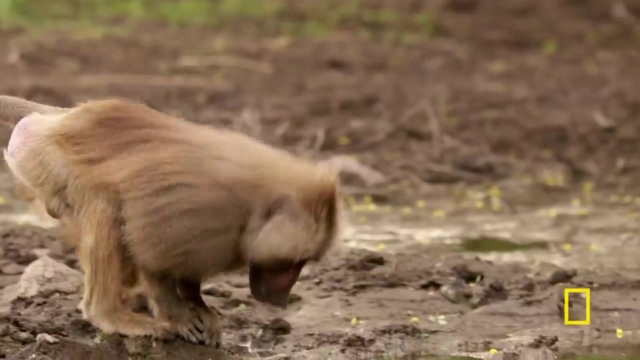 But earth this dry needs more than a shower. This is one of the most drought-prone countries in the world, And it's getting worse As our climate changes. water shortages are sparking conflict for animals and humans alike. One of the only waterholes for miles. 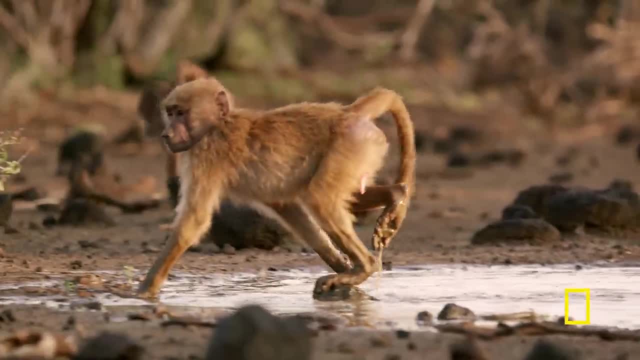 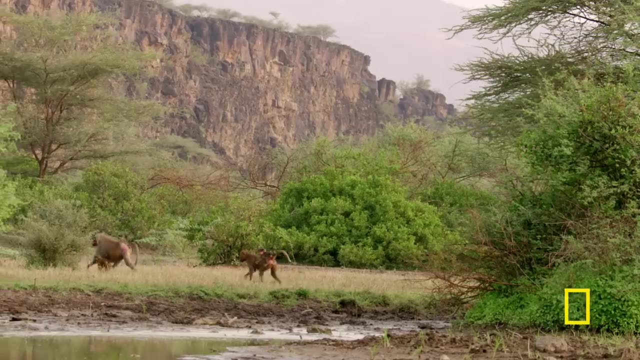 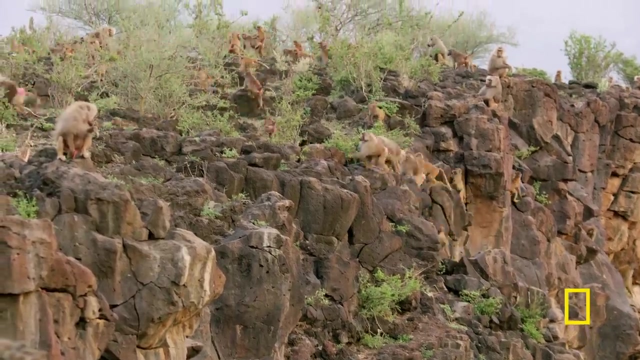 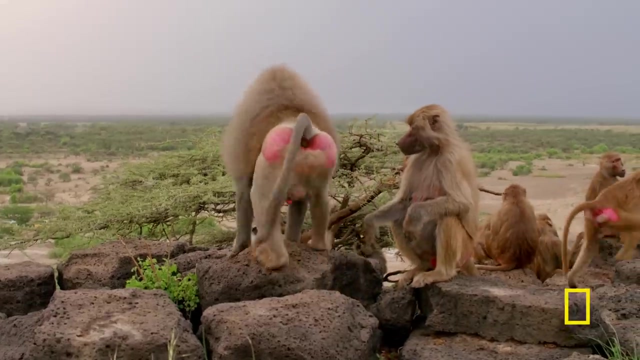 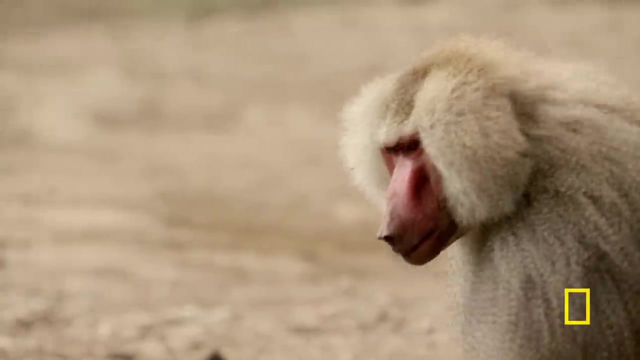 It provides enough water for this band of baboons to survive the dry season. They're relatively strong in health and numbers. They're relatively strong in health and numbers. Further out on the arid plains, another band is thirsty. Further out on the arid plains, another band is thirsty. 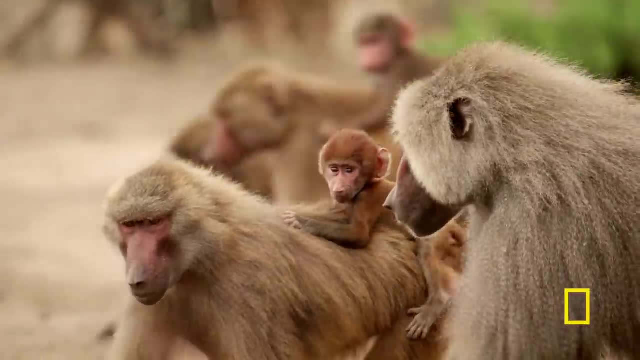 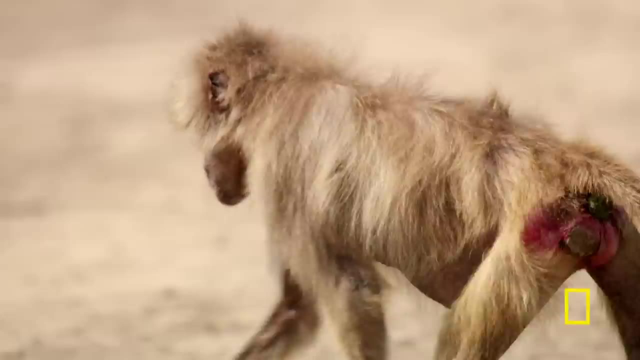 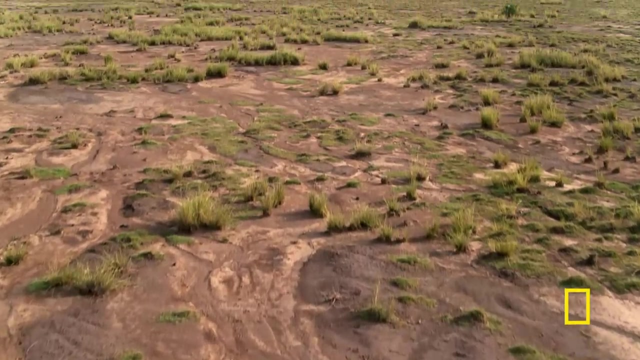 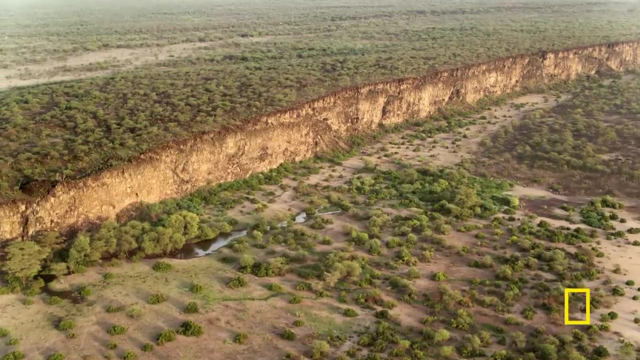 They're in close contact with the mist. There's a waterfall below the cliff, But when two bands meet, It nearly always ends in They're forced to the same waterhole below the cliff, But when two bands meet always ends in violence. 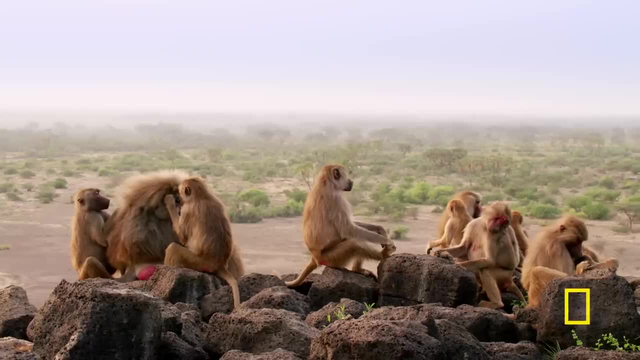 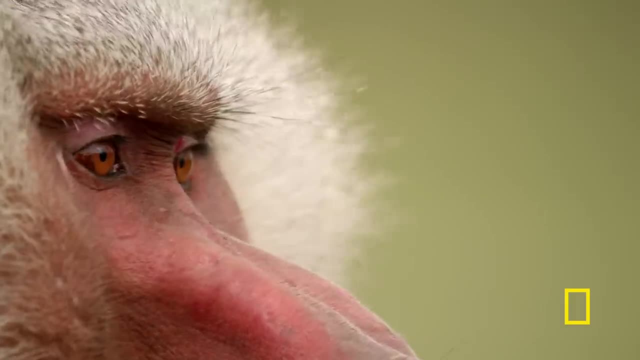 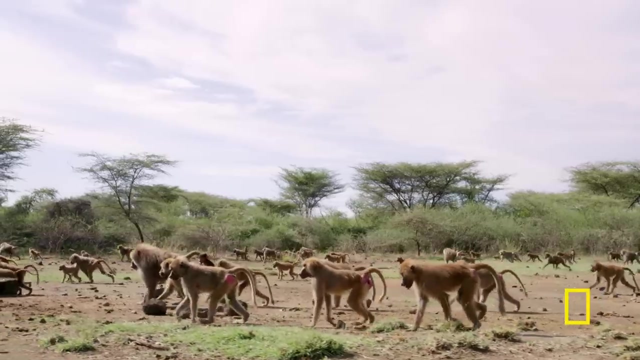 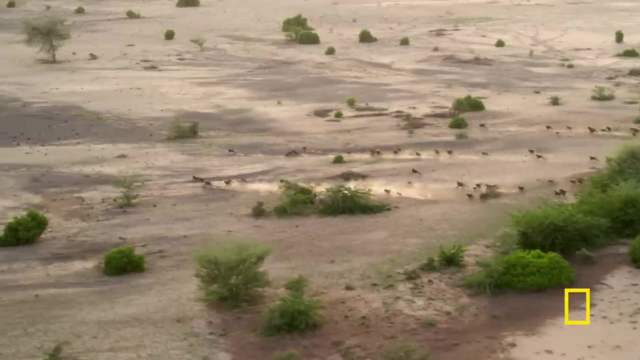 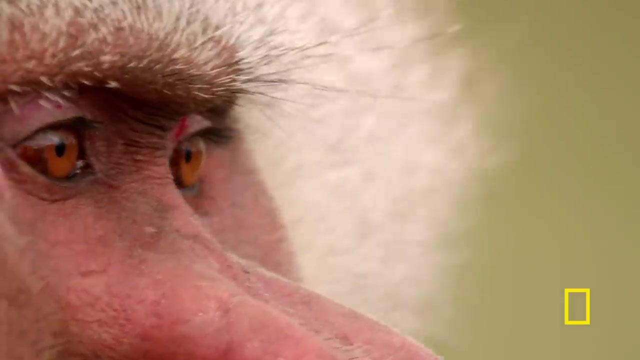 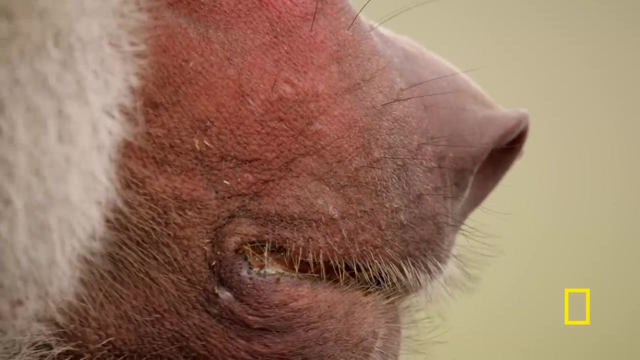 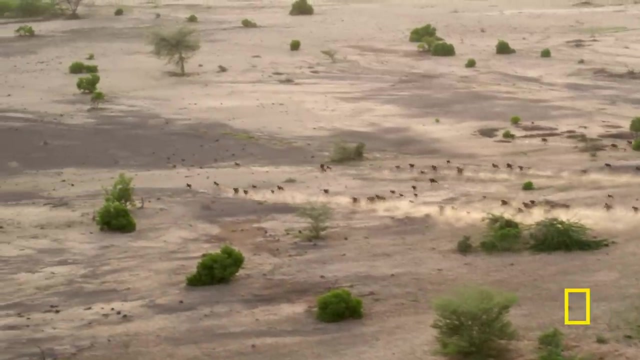 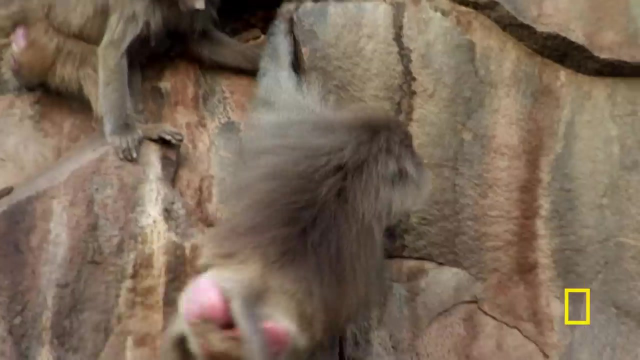 Females and babies are most at risk. If the outsiders want a drink, they'll have to fight One waterhole, Two bags of booze. The outsiders need to drink, But the band at the waterhole is stronger. This is how wars begin. 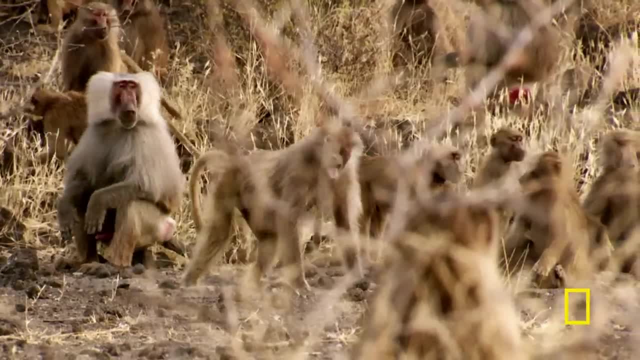 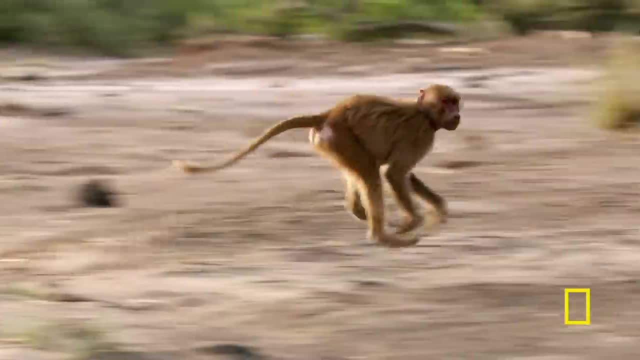 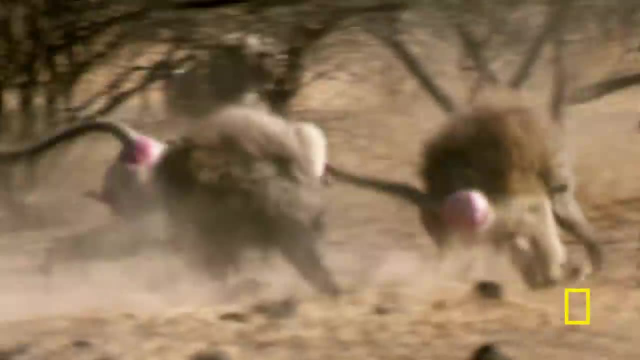 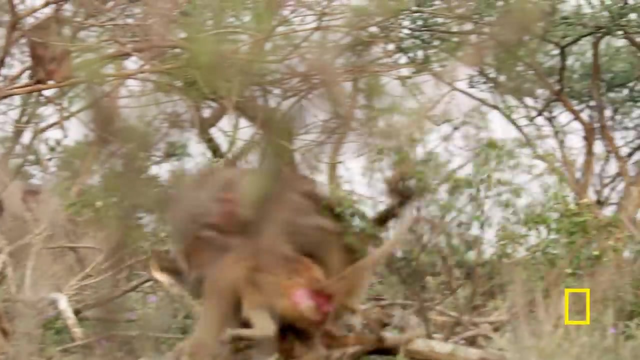 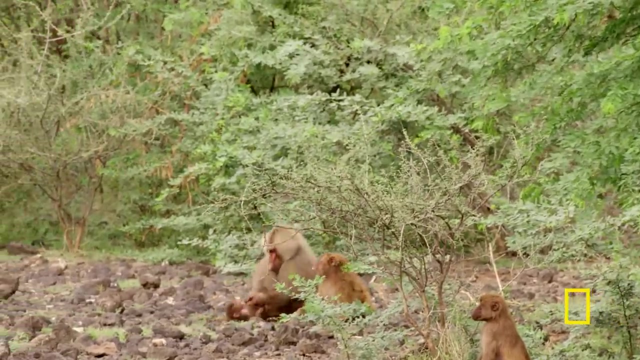 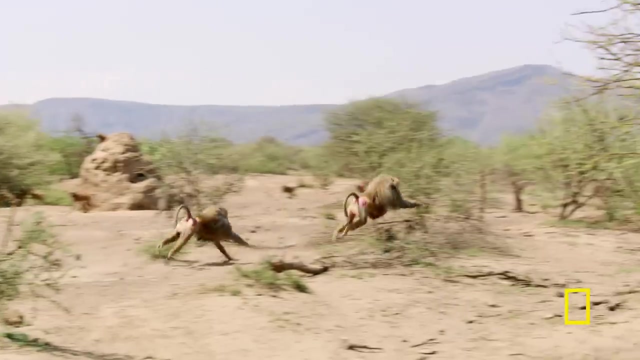 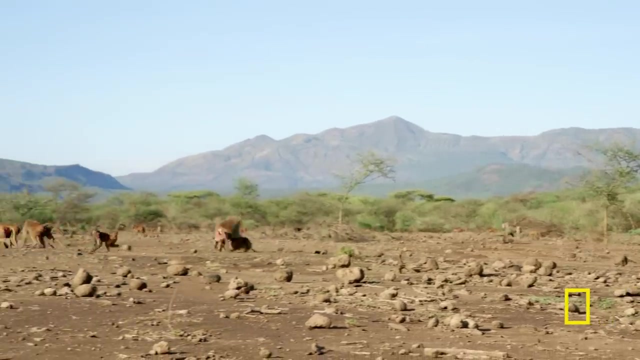 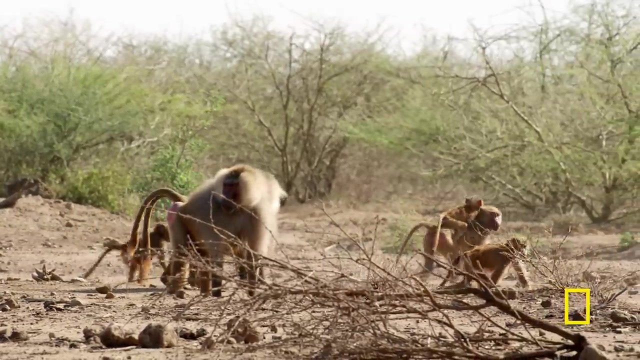 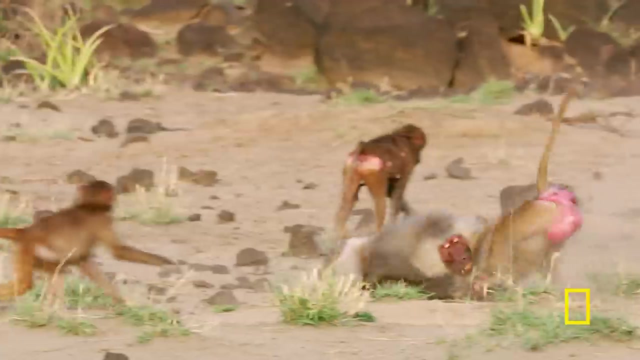 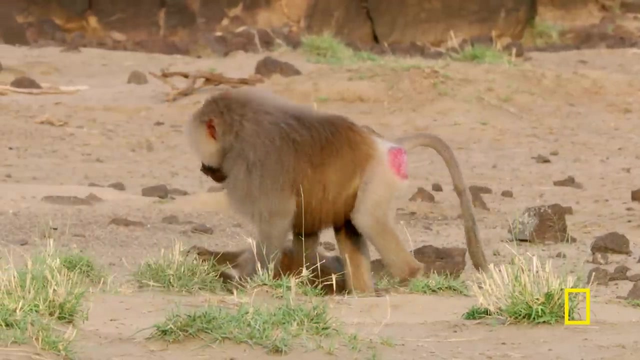 The best survival strategy here is to form super bands Bigger than the opposition. That's why they get far And fast. The outsiders are forced to retreat, But not fast enough. These baboons use battles to steal females from each other. 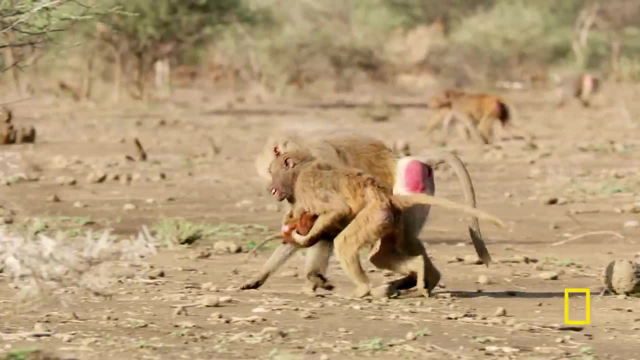 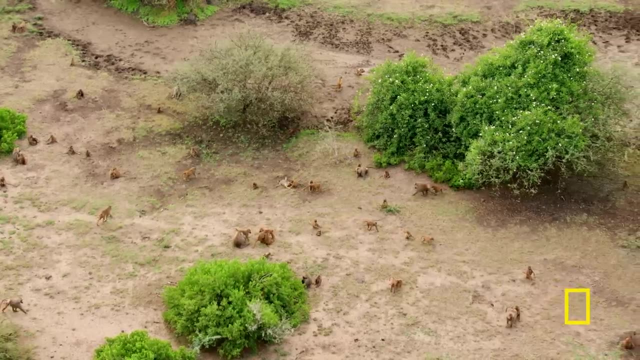 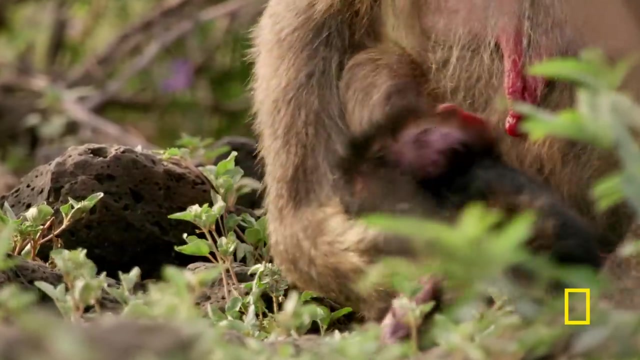 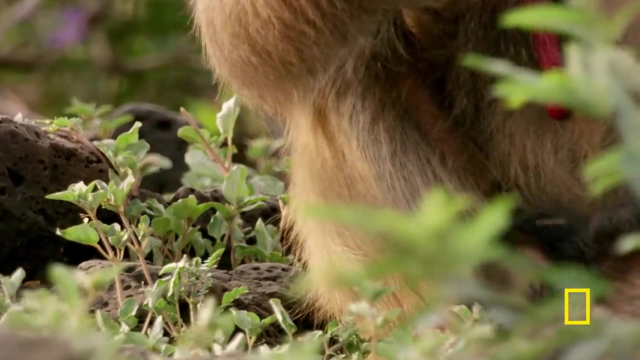 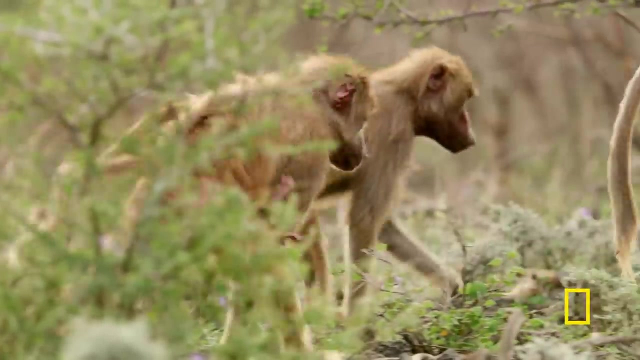 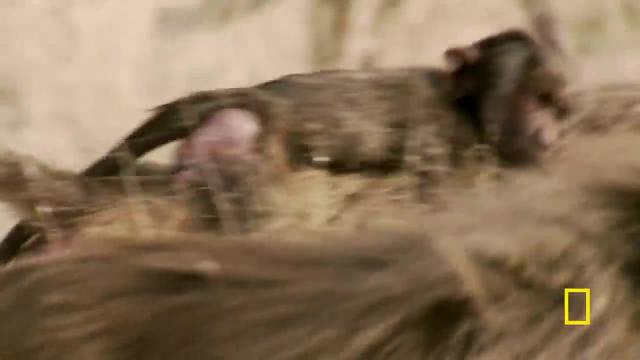 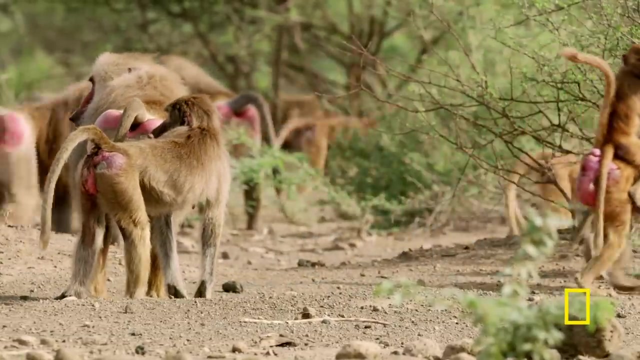 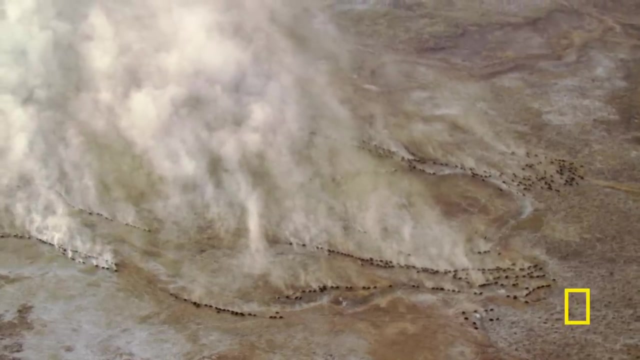 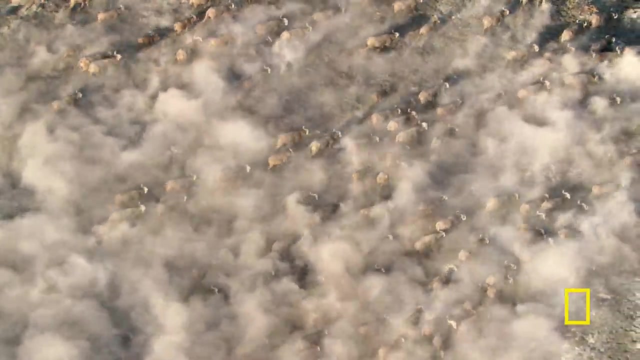 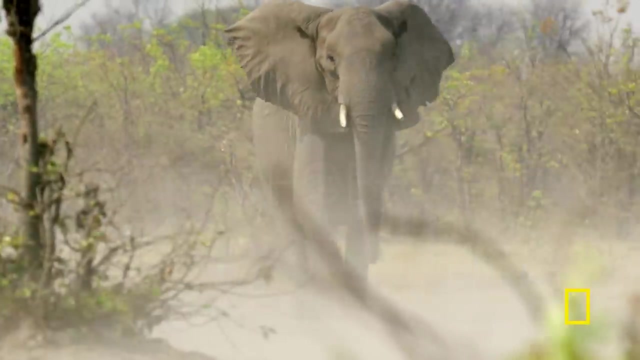 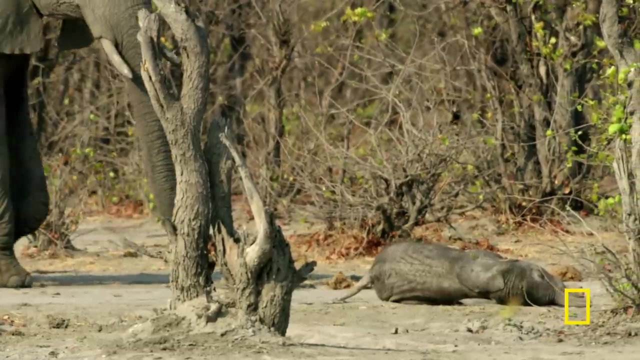 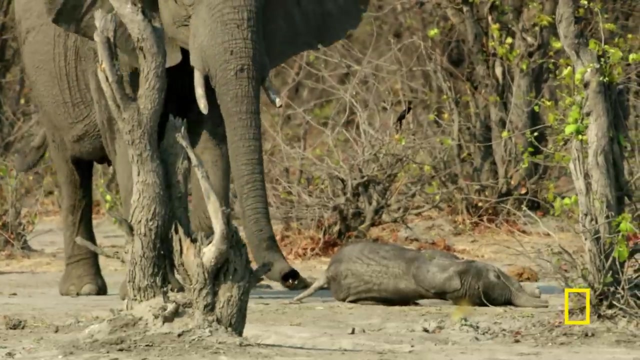 The winners expand their ranks, while the outsiders grow even weaker, All they can do is bide their time and try again. As the drought reaches its peak, famine becomes a harsh reality. Mum, just a few months old, born at the wrong time. 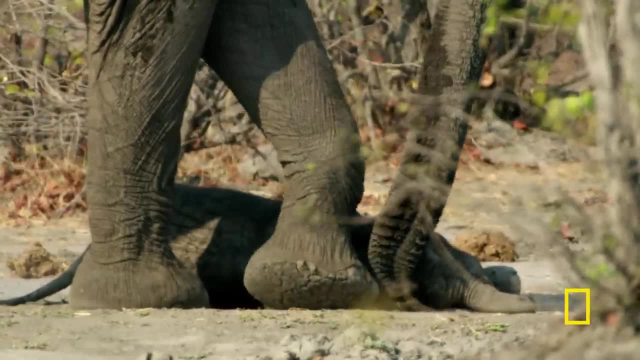 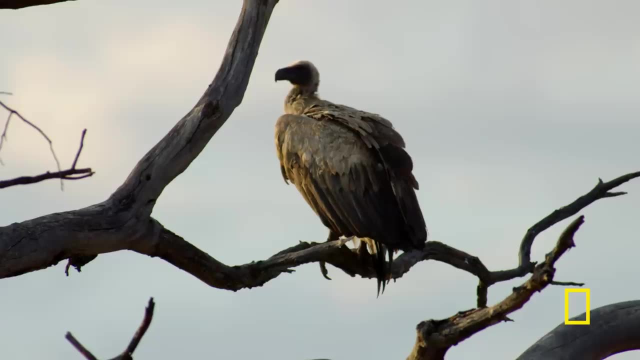 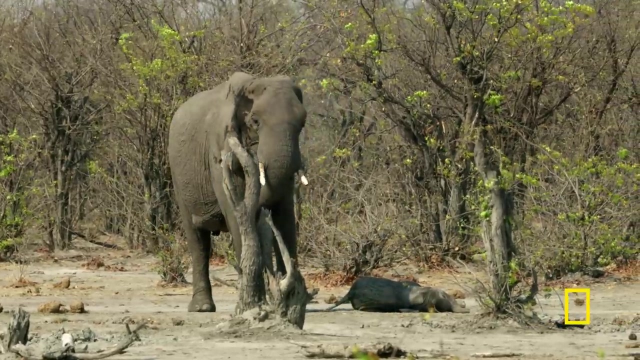 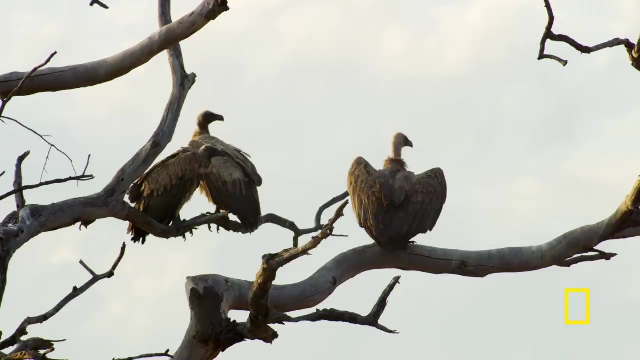 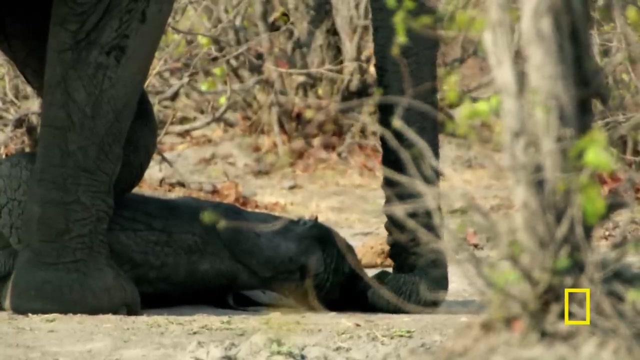 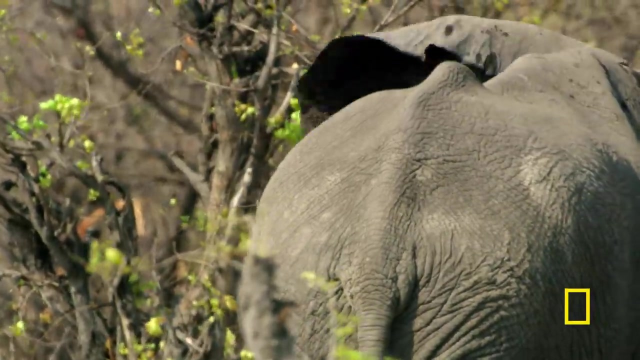 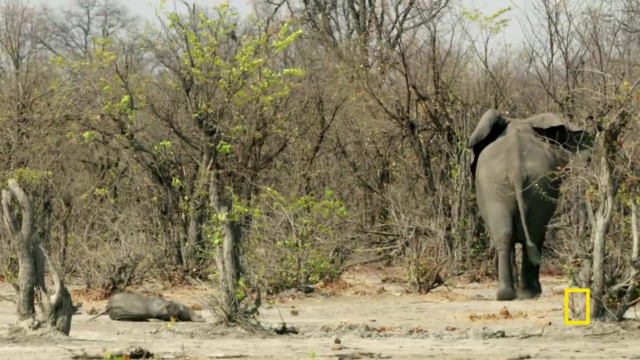 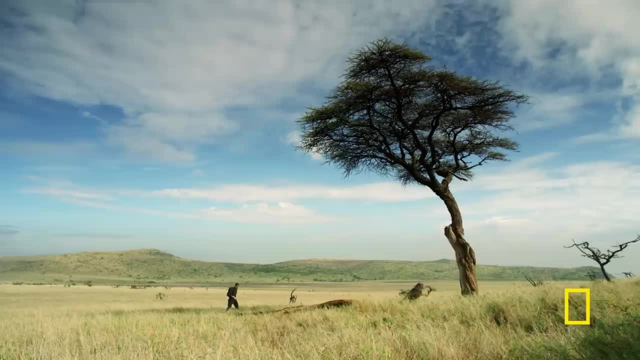 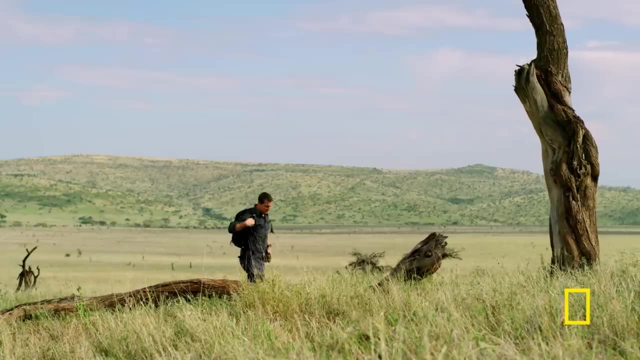 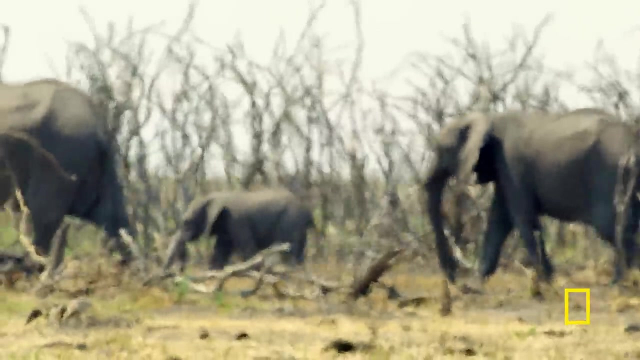 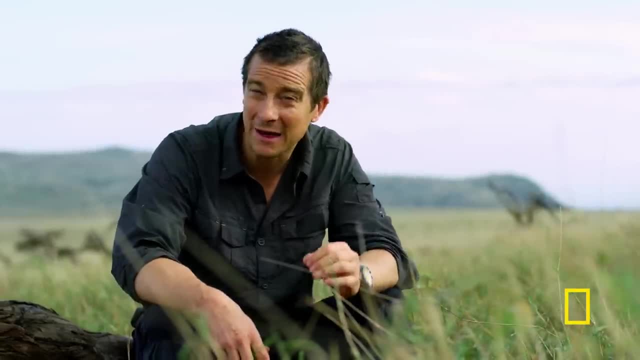 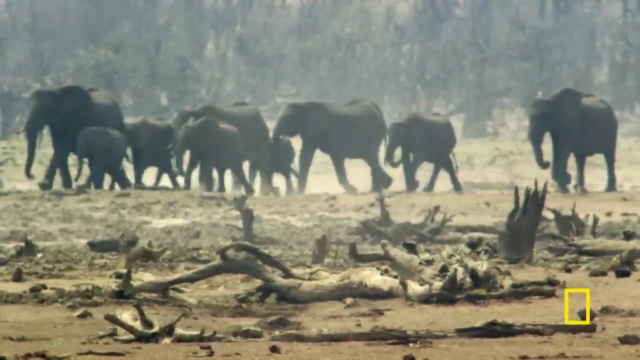 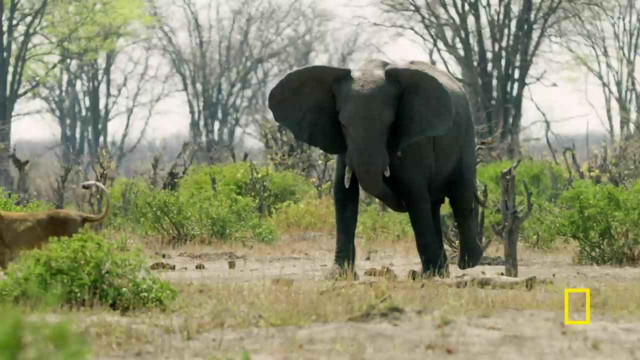 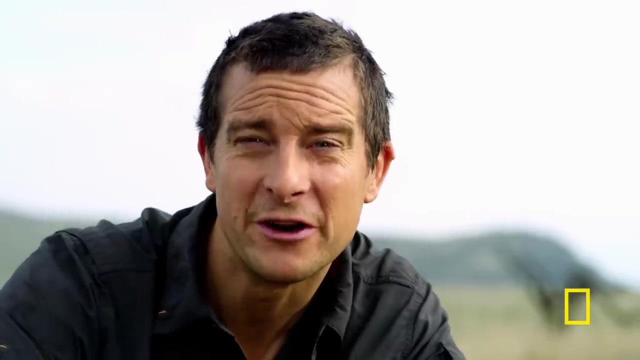 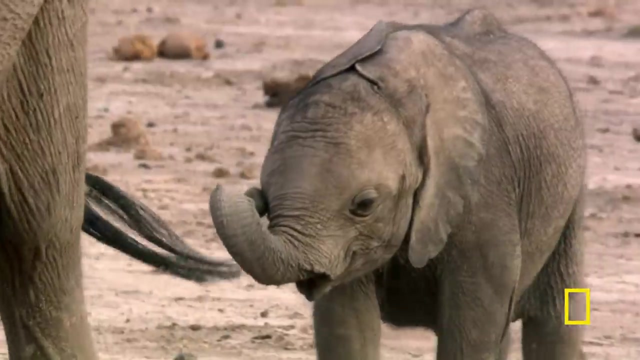 and unpredictable. only the strongest will have what it takes to make it, through Adaptability, Unfailing resolve And the hope that eventually, better days will return. Six months older and born just before the wet season, this calf had a stronger start. 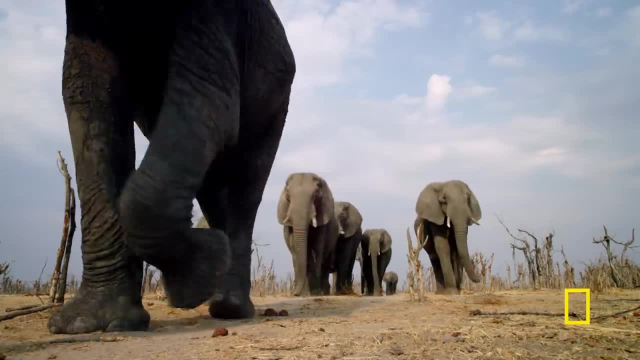 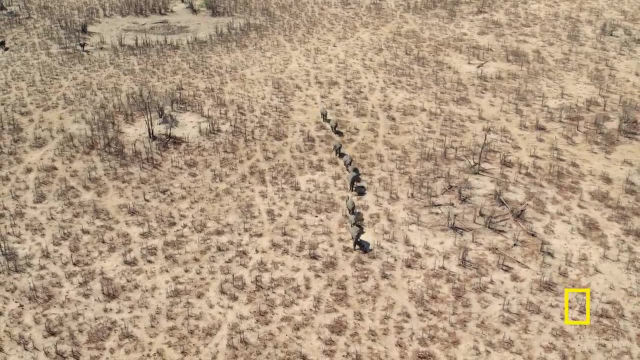 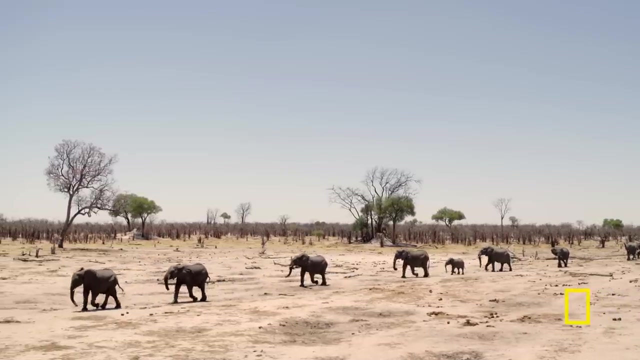 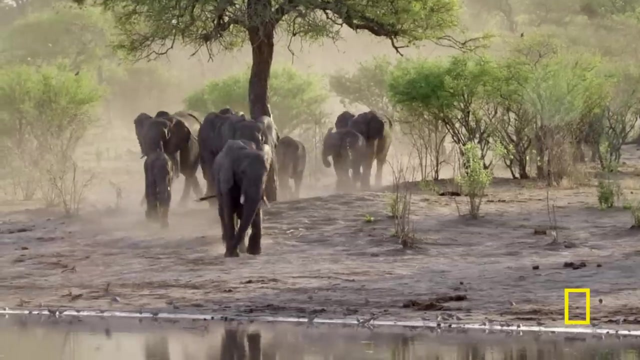 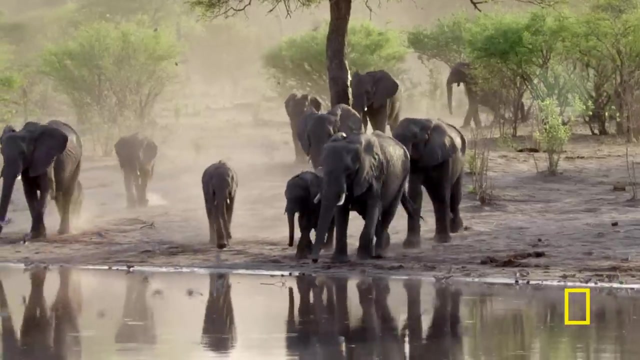 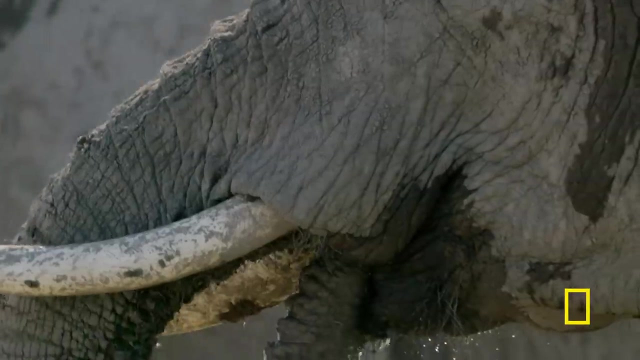 The matriarch has seen hard times before. She knows how to lead her family through. She's turned over, But she's not alone. Enough water to go round until the rains return. PUSHING, PUSHING, PUSHING, PUSHING, PUSHING, PUSHING.